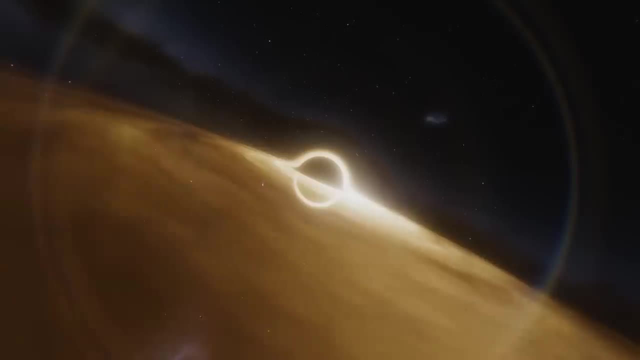 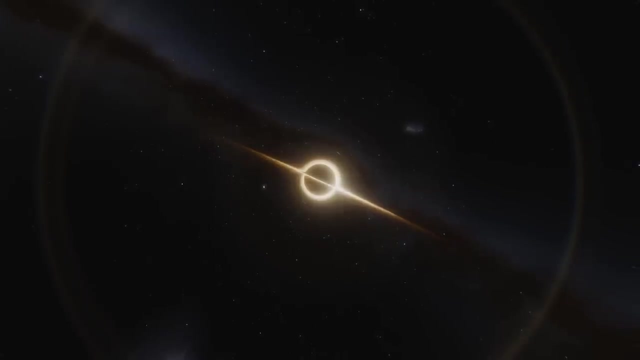 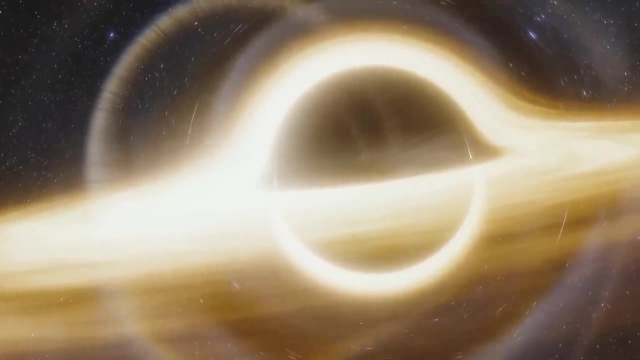 could escape. everyone you know and their distant descendants are already dead. And it isn't just time that warps. Assuming you approach the black hole's gaping maw feet-first, then your lower body will be experiencing a stronger gravitational pull than your head. Your entire body begins to. 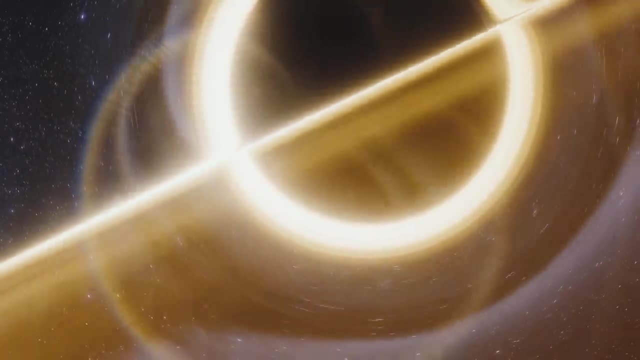 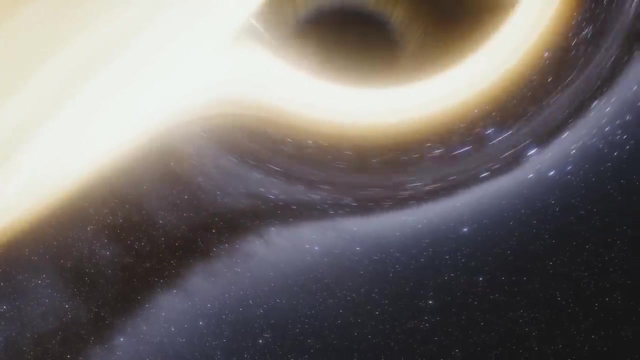 distort. although you can still see the black hole, Your entire body begins to distort, although the effect isn't as severe as it could be. A supermassive black hole like Sagittarius A-star only has a moderate gravitational gradient compared to their smaller stellar. 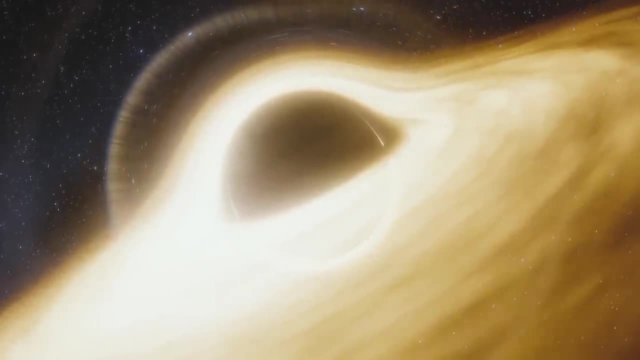 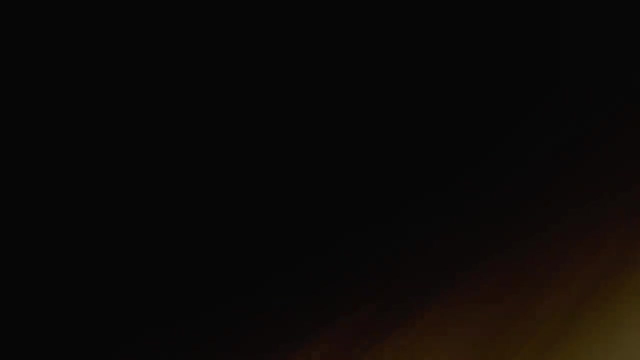 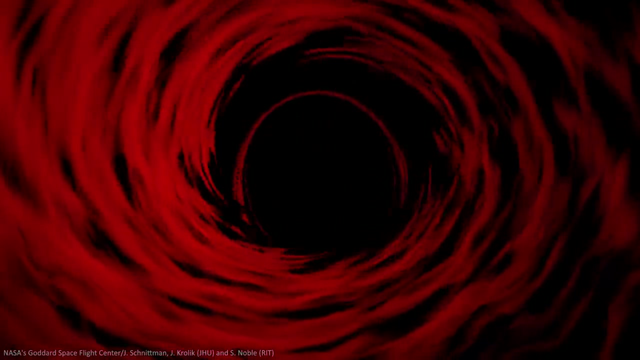 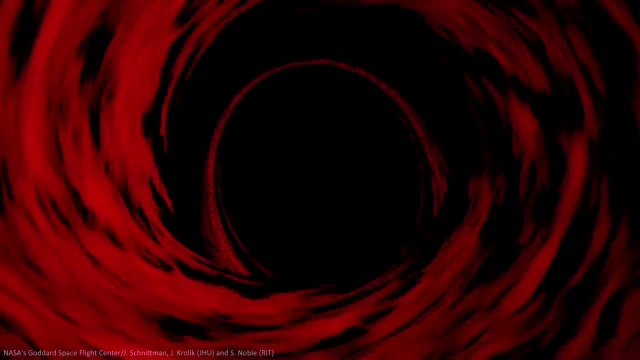 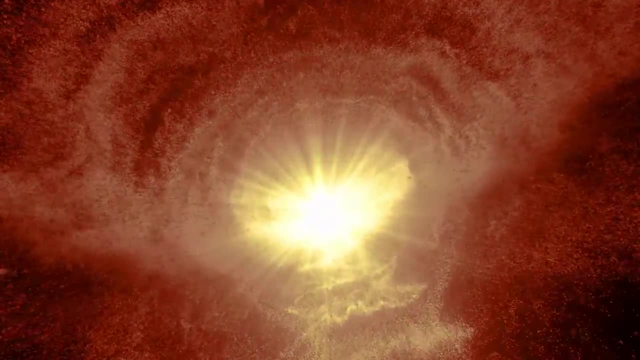 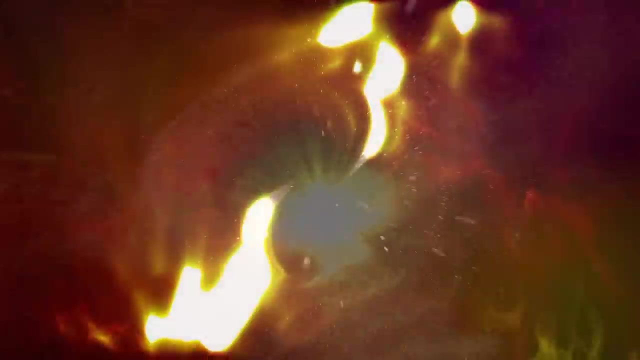 Inside, everything is turned on its head. Time and space trade places, and beyond the event horizon, it is time itself that pulls you down towards the center. No force in the universe can stop this, just as nothing can stop the flow of time itself. 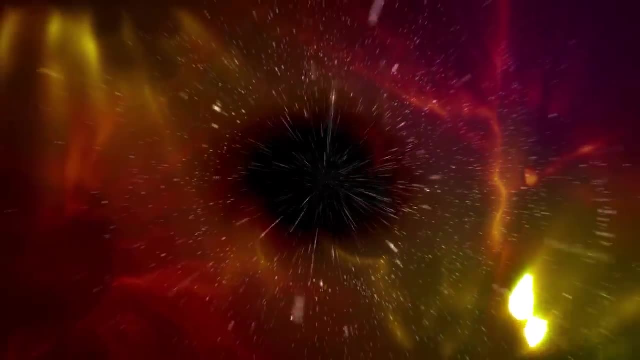 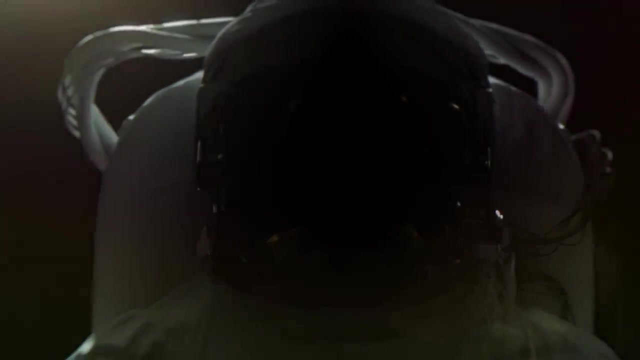 What all experience will give you insides, no one can say, And not you. Even if, impossibly, you survived irradiation, spaghettification and the aging of the universe, then your voice would be forever silenced by gravity itself. 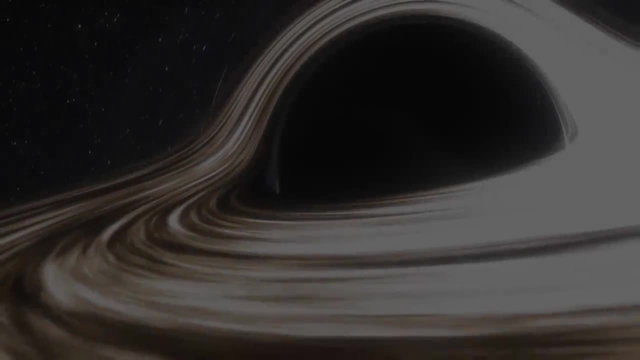 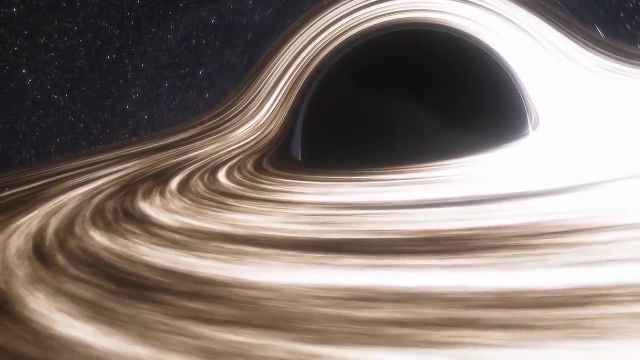 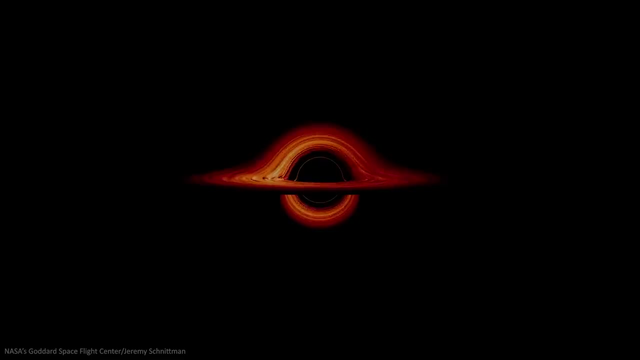 All that is left is the slight mass increase of the leviathan that consumed you, a mass increase that will only help your captor pull in more victims. Such is the fate of anyone or anything unlucky enough to fall into the mouth of a black hole. First mooted in 1783,, the incomprehensible horror of these ultimate galactic predators has captured the imagination of scientists and pushed the boundaries of science for decades. Indeed, the supermassive variety are thought to reside at the centre of every galaxy. 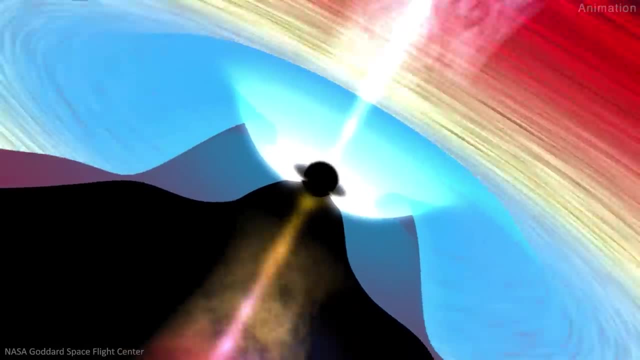 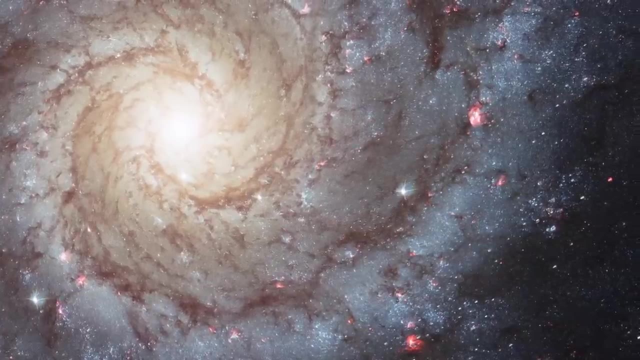 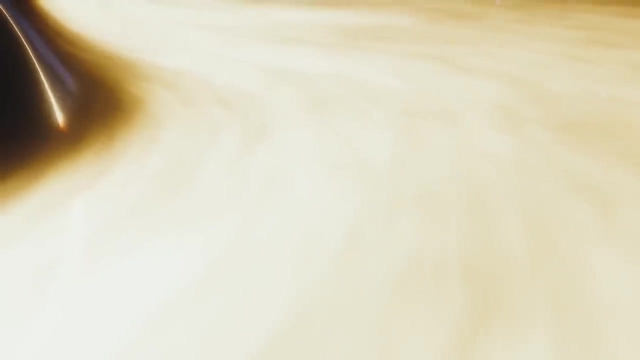 and may well be the agents of their creation. While black holes can bring about ultimate destruction, their supermassive counterparts can also feed and fuel the universe. They can also fuel the very stuff of stars, planets and life. But many of these supermassive black holes also leave us with a mystery. 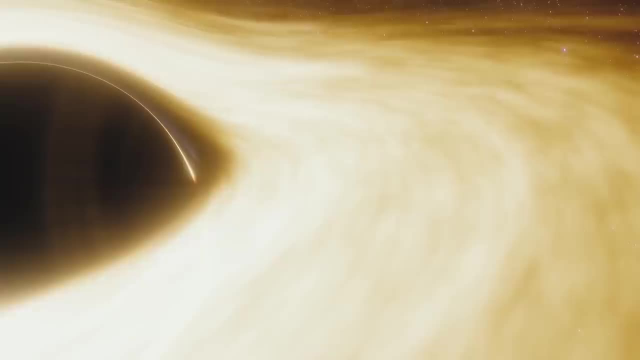 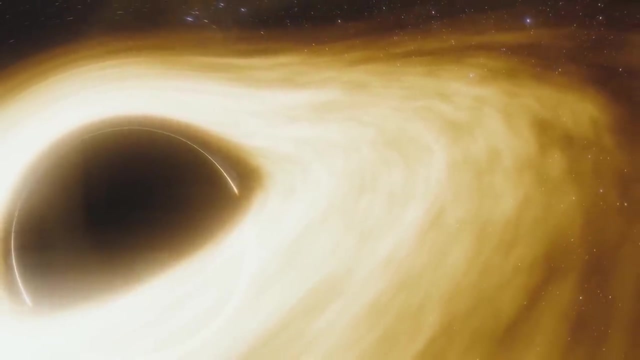 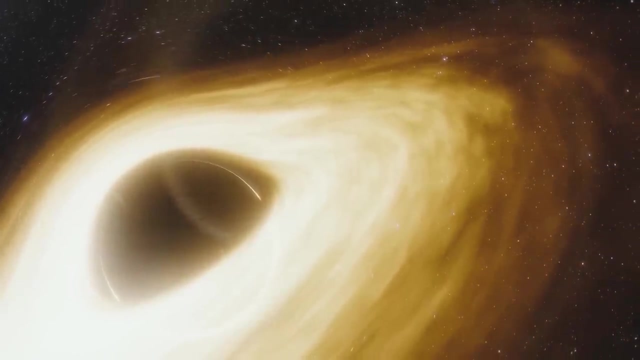 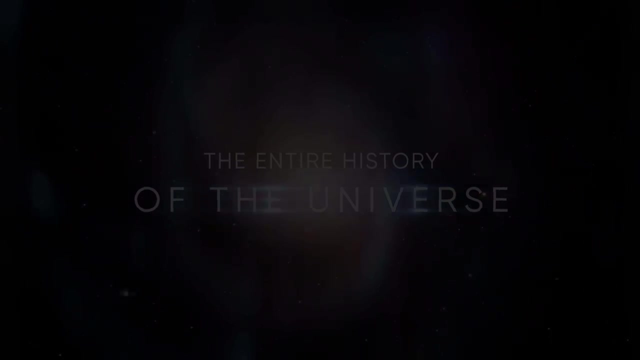 Just how did they get so big in the first place? If they are the seeds of galaxies, then what were their seeds? And finally, when and indeed what were the first black holes? Let us know in the comments below. Thank you so much for watching and I'll see you in the next video. 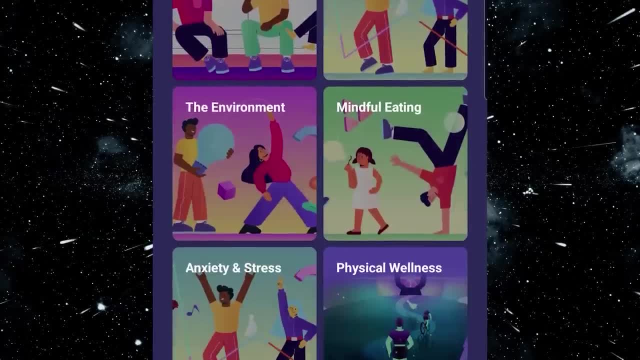 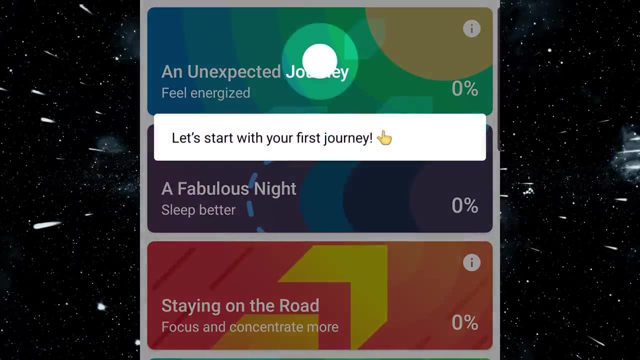 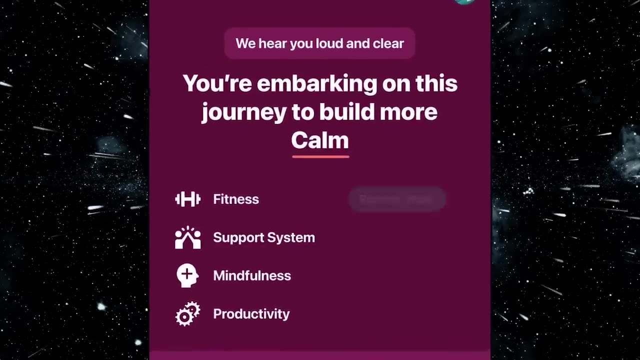 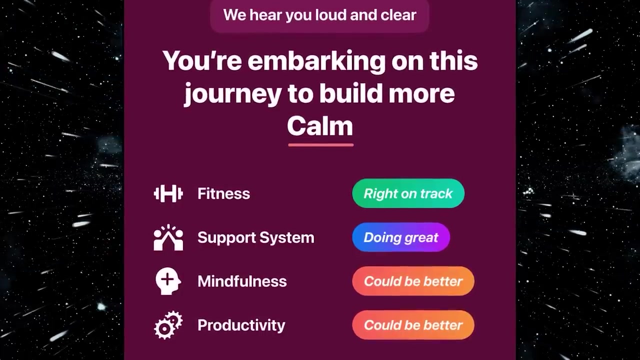 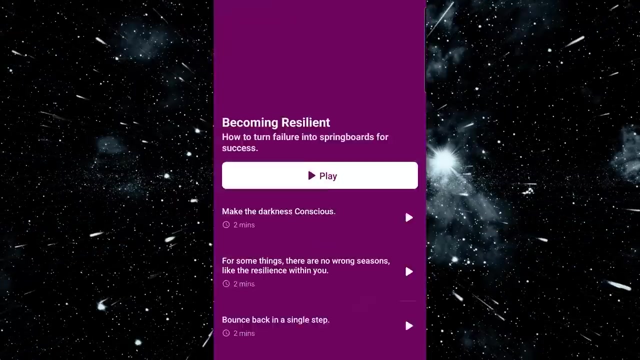 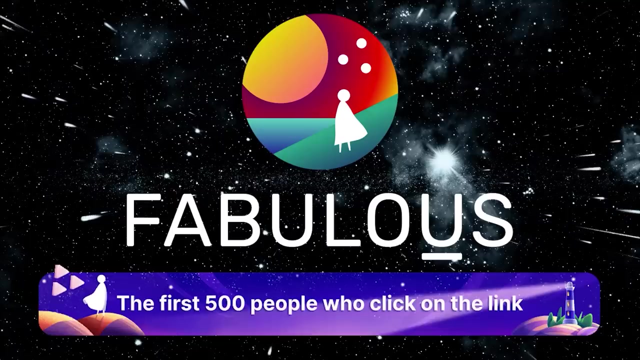 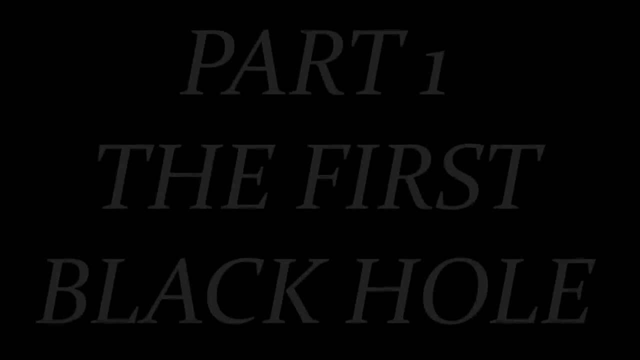 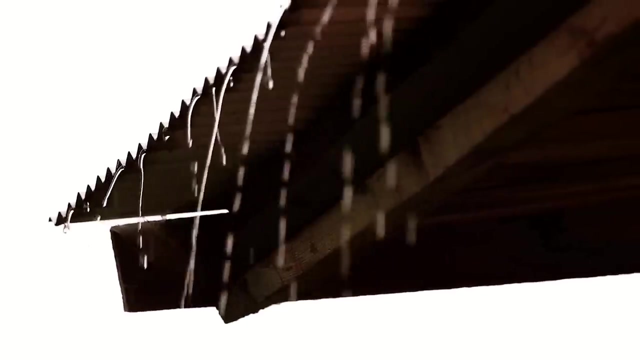 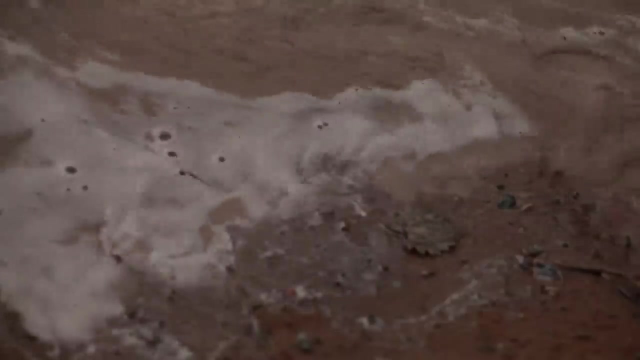 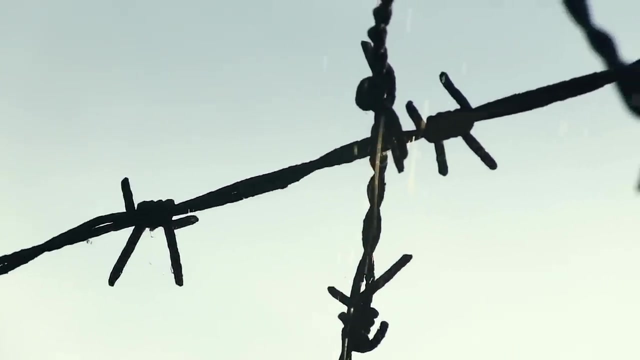 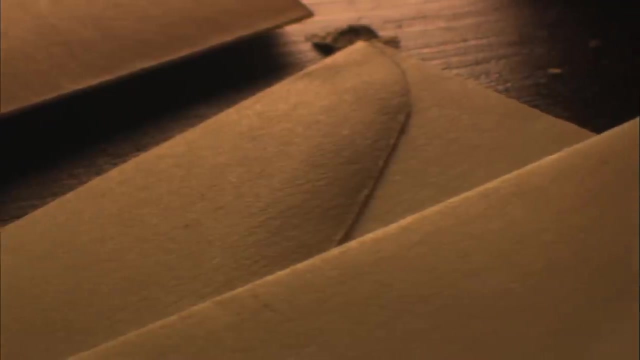 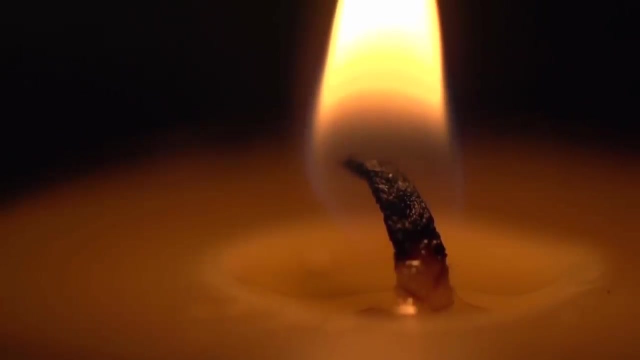 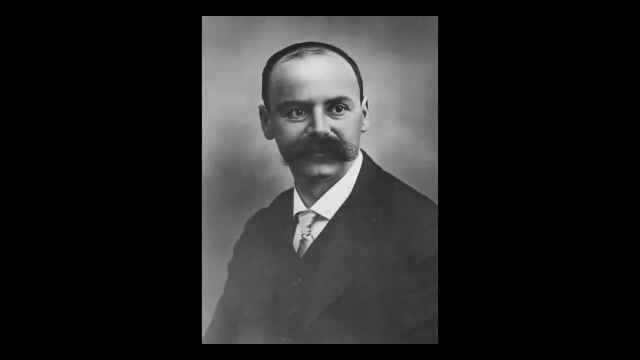 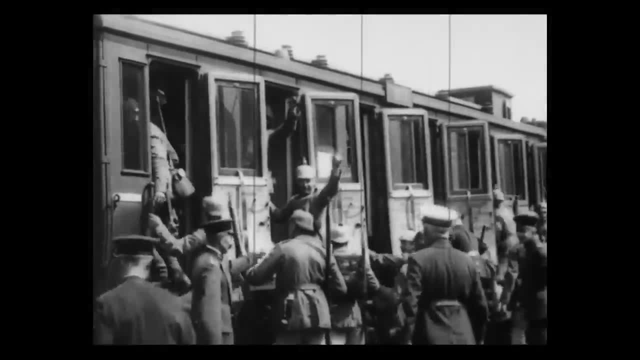 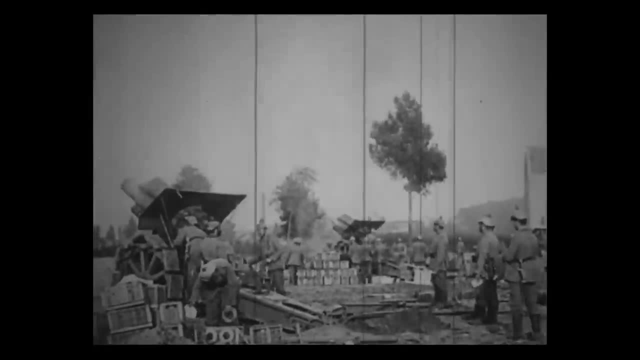 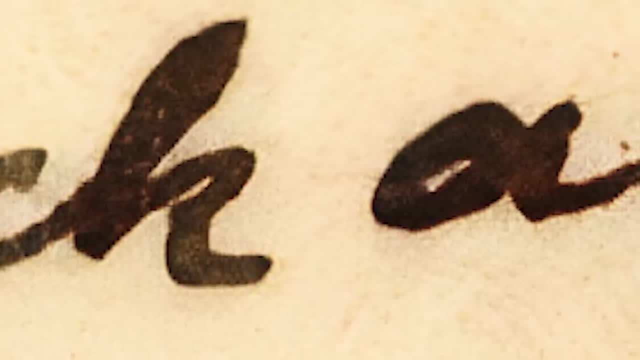 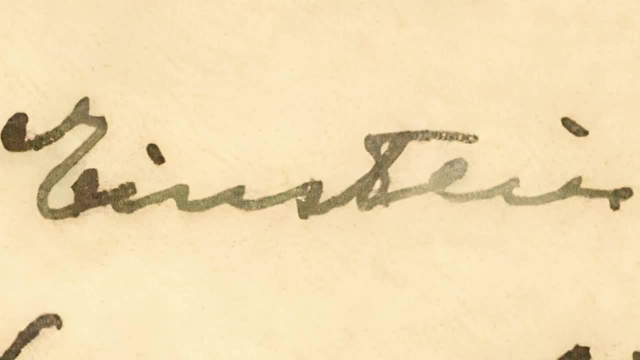 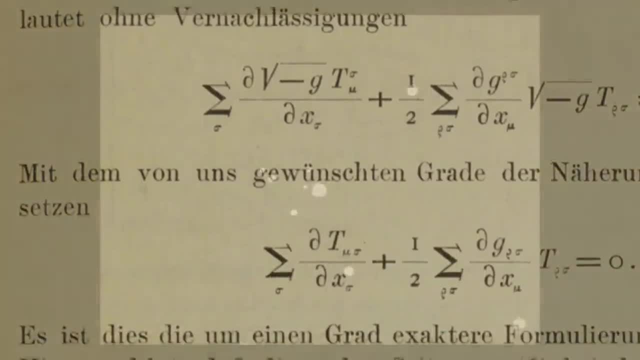 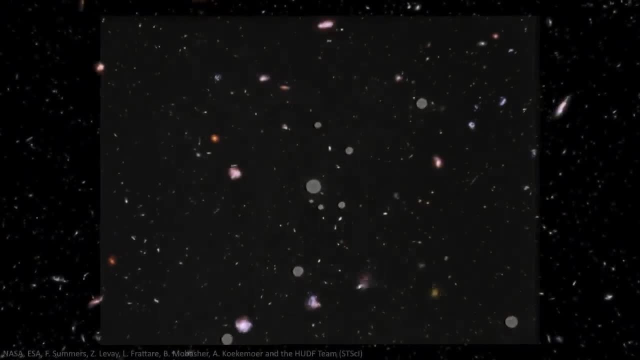 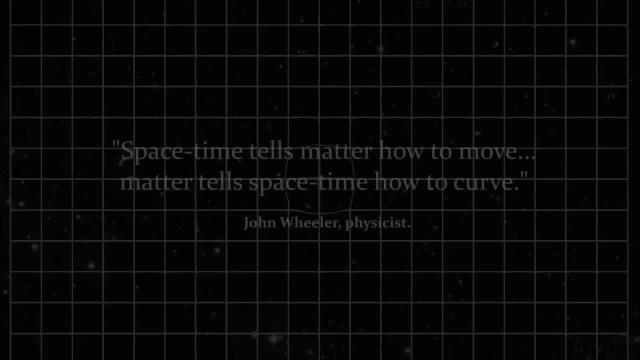 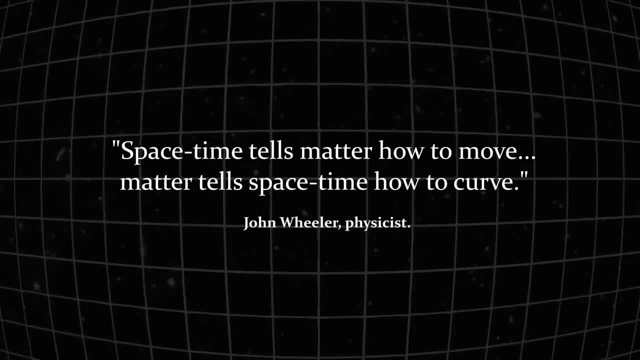 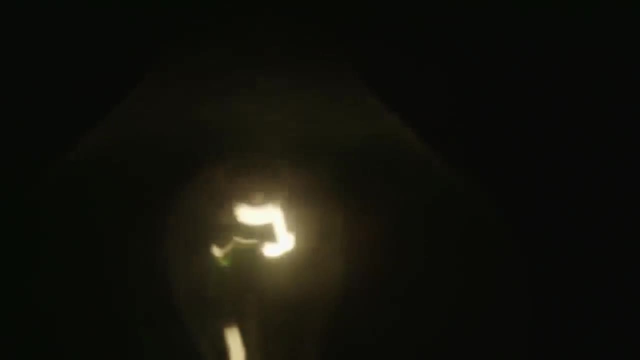 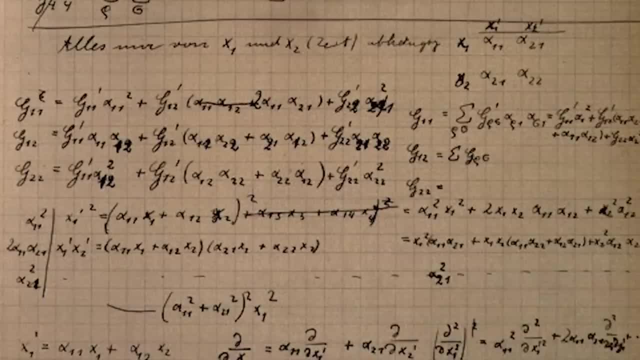 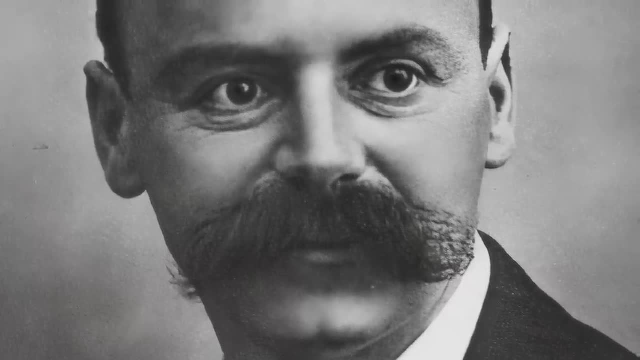 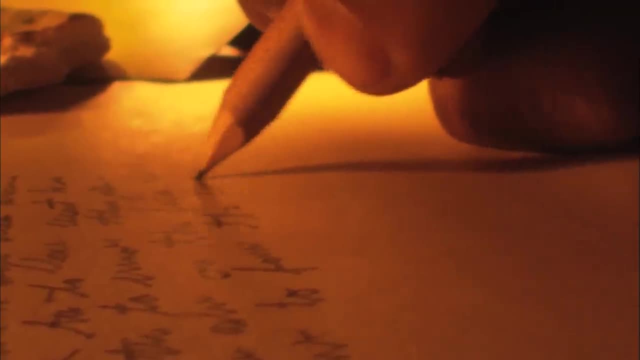 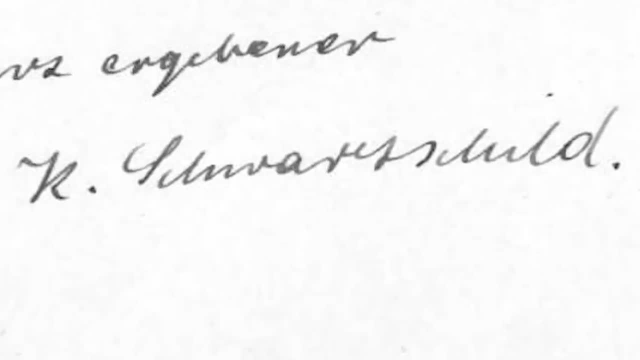 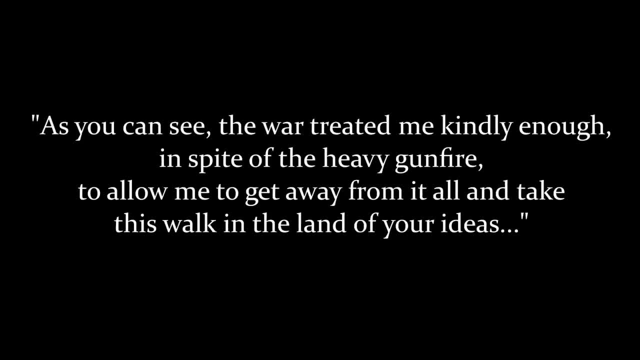 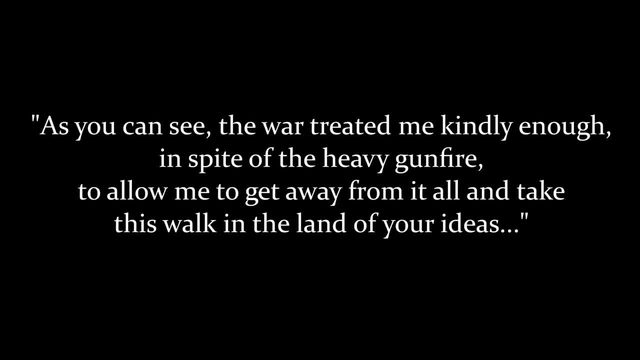 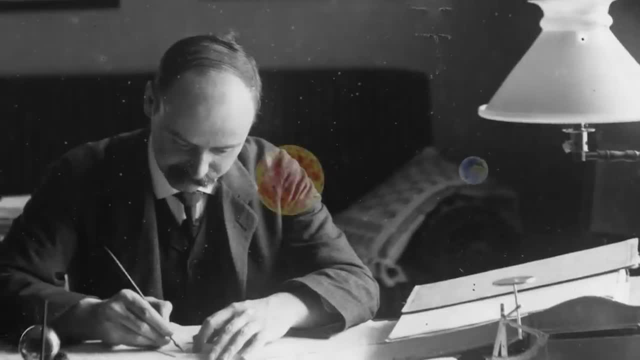 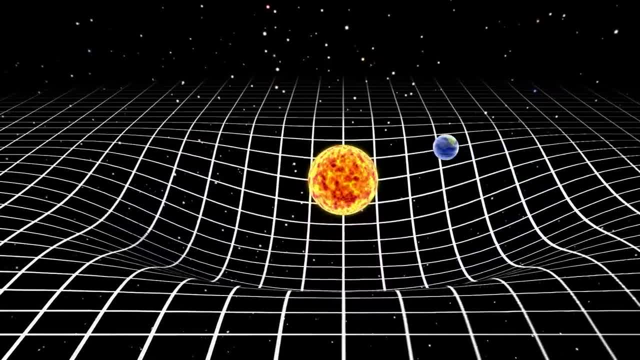 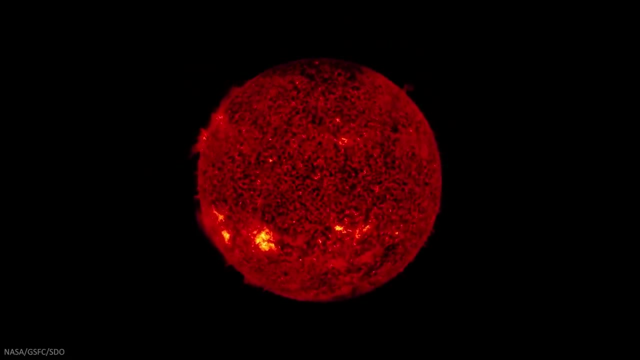 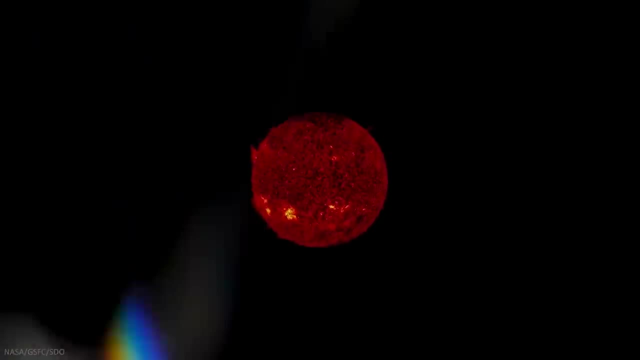 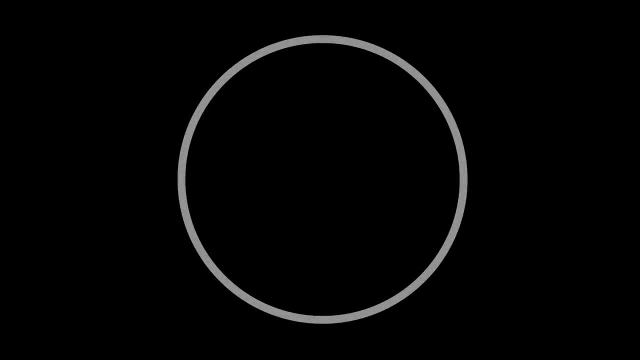 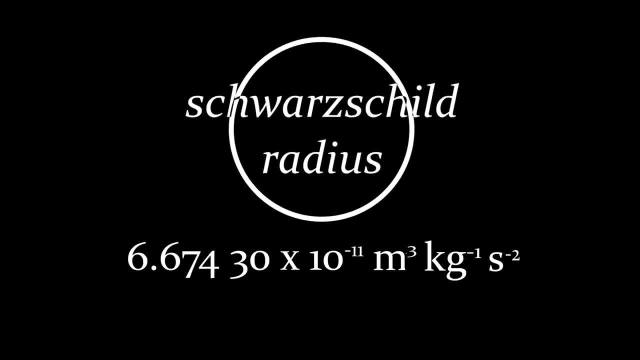 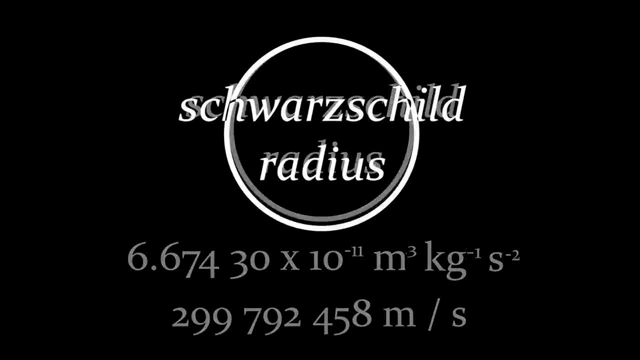 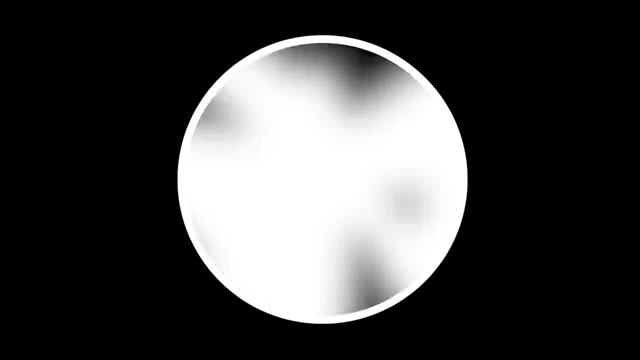 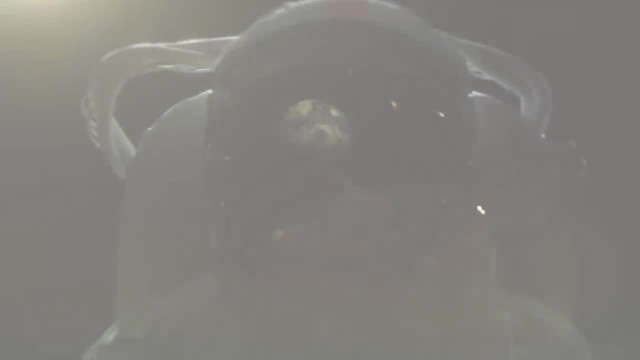 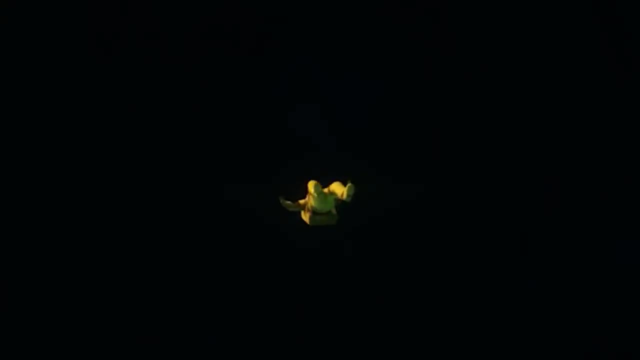 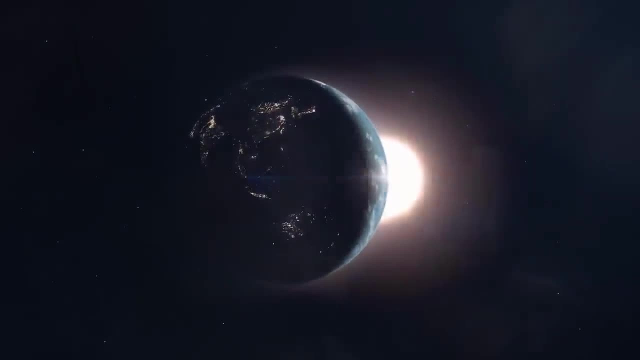 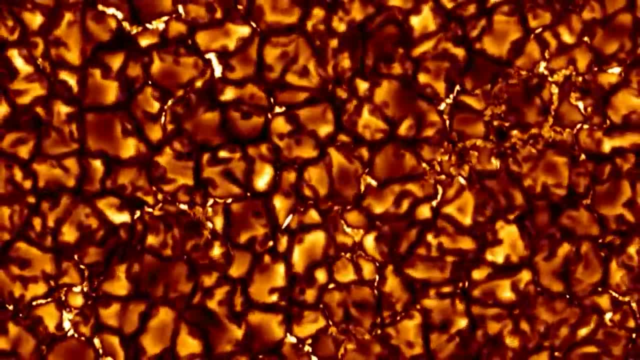 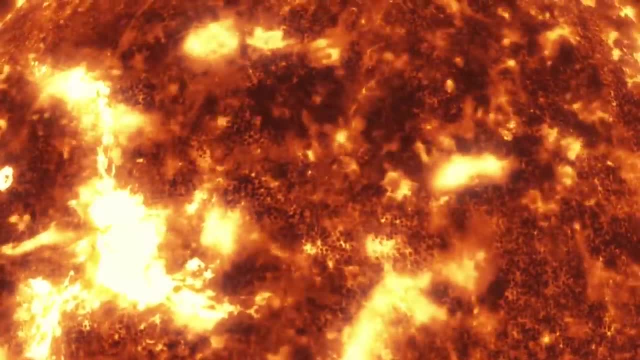 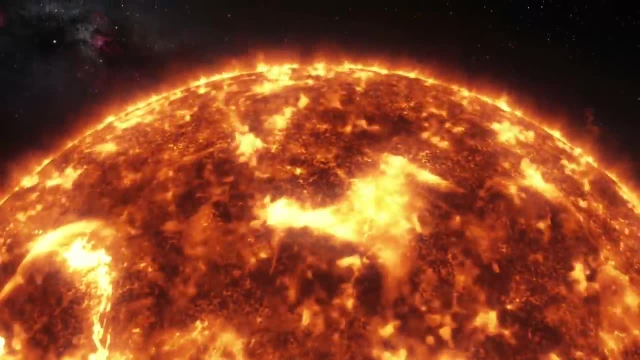 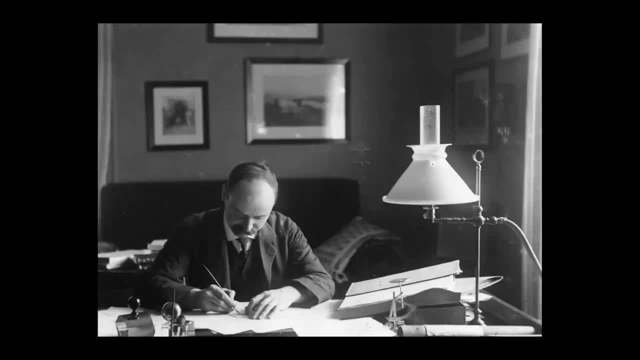 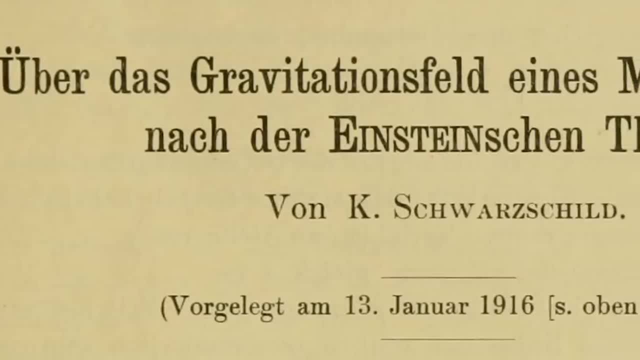 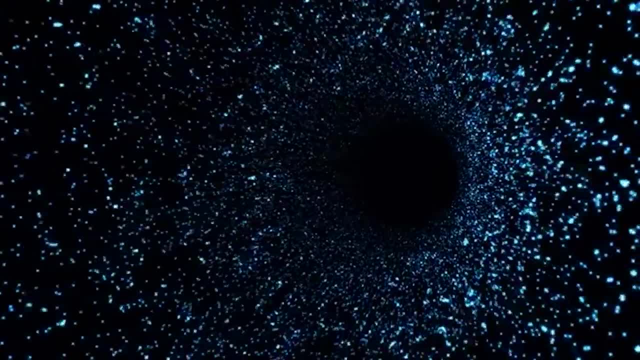 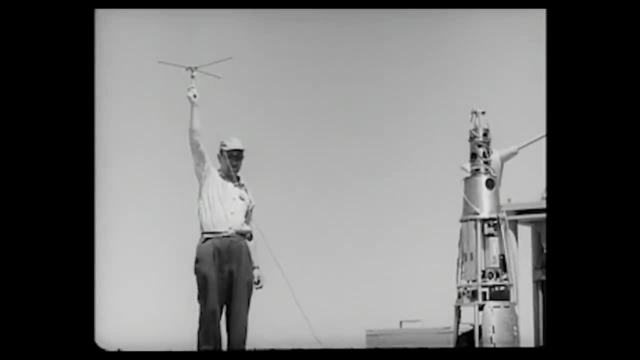 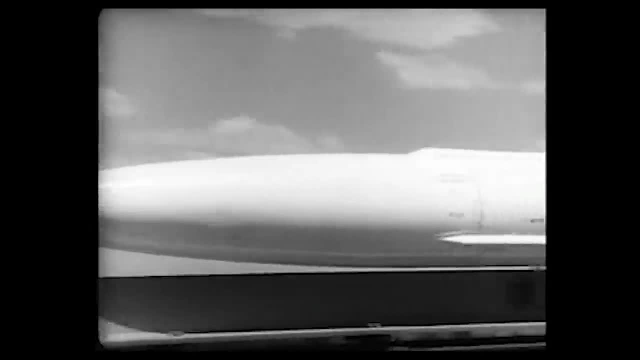 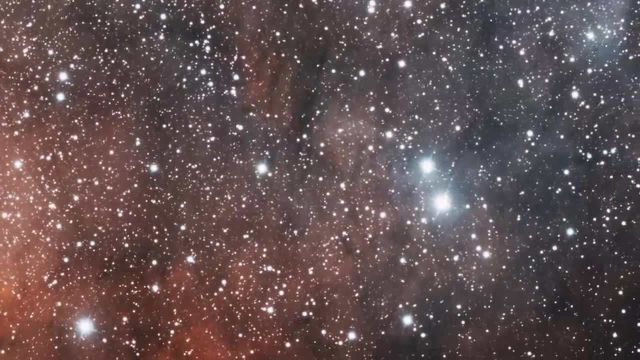 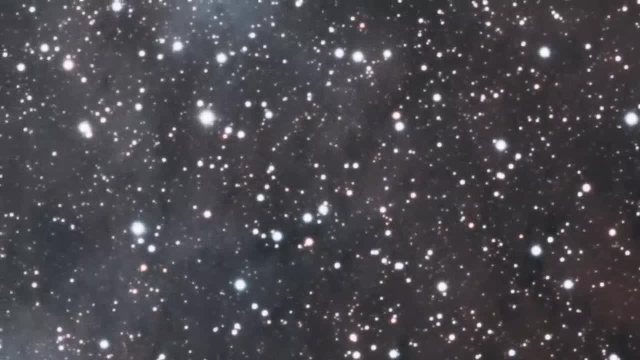 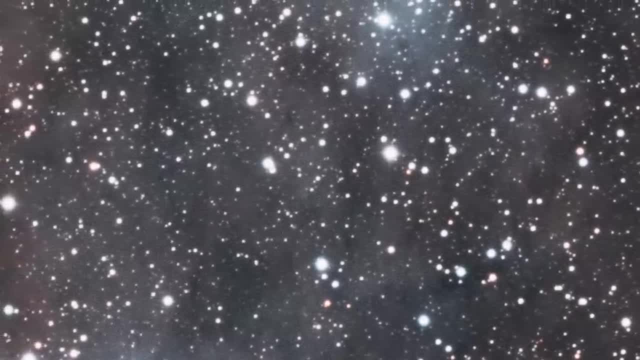 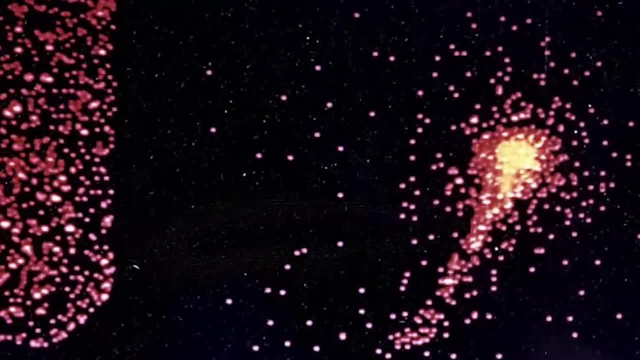 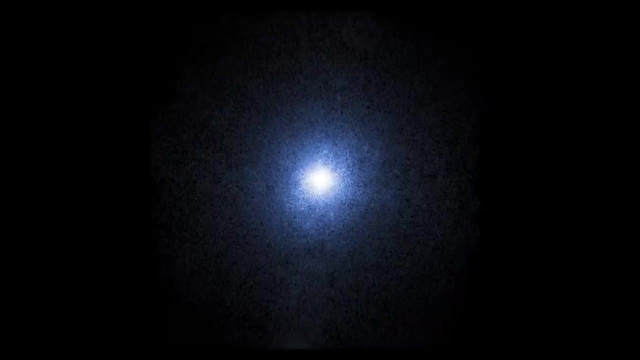 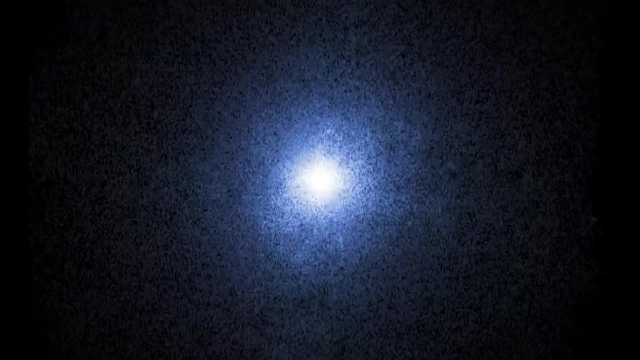 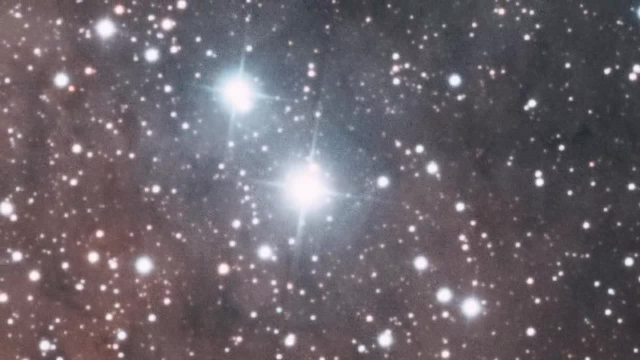 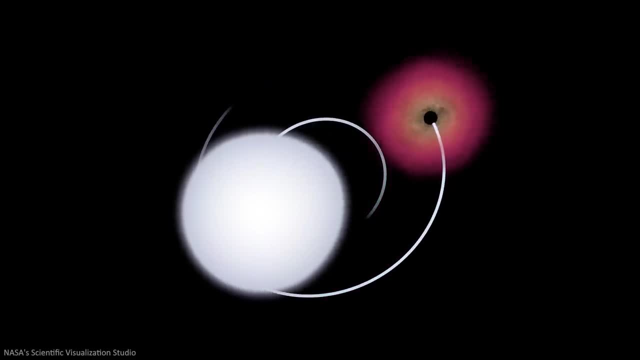 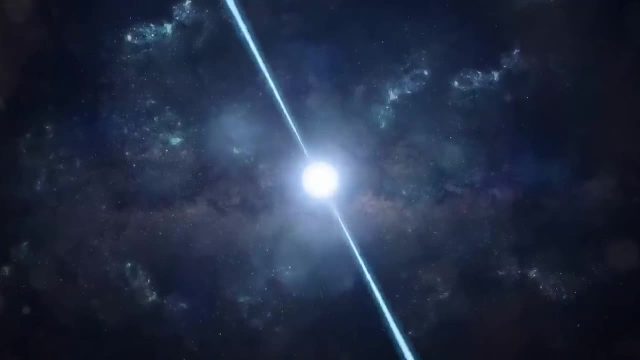 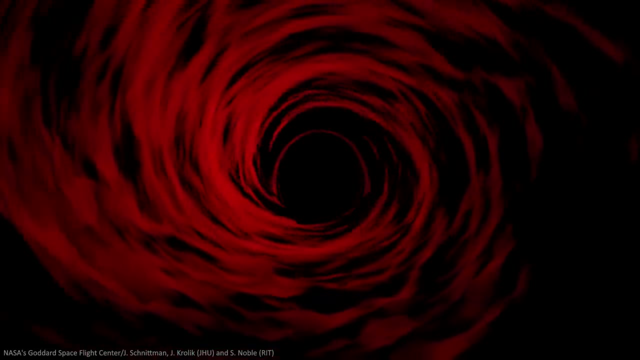 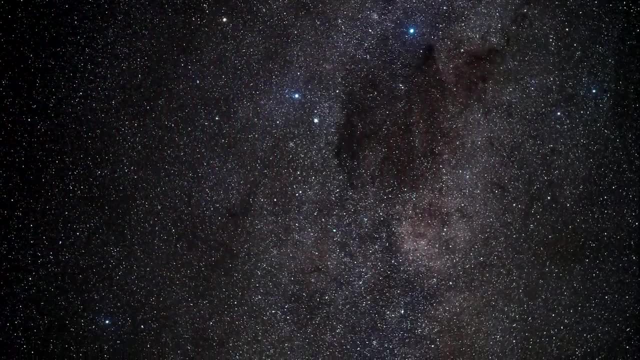 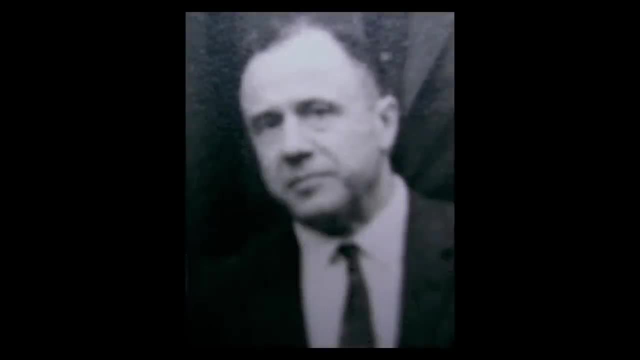 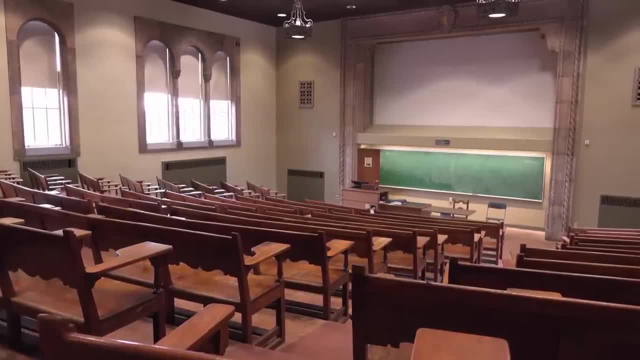 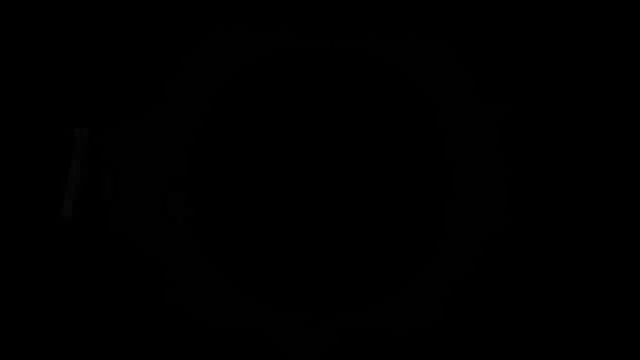 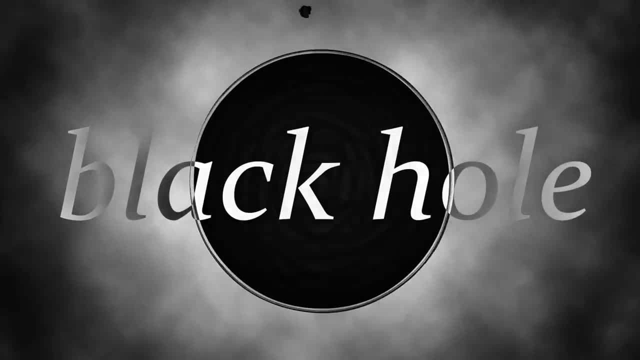 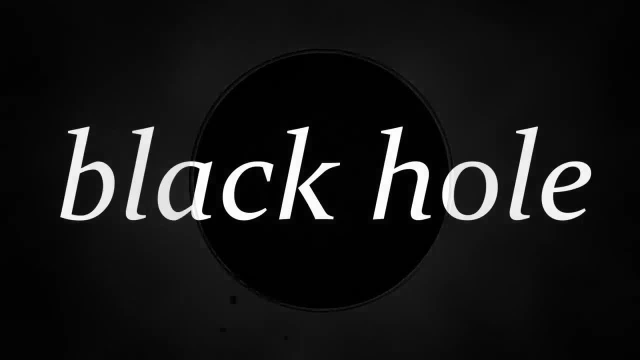 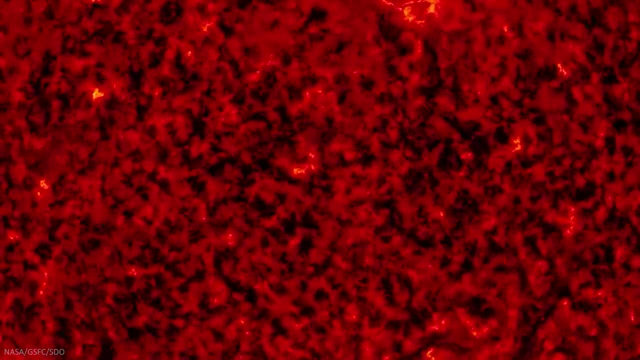 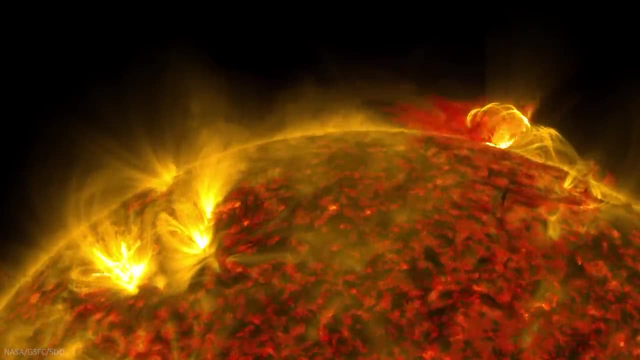 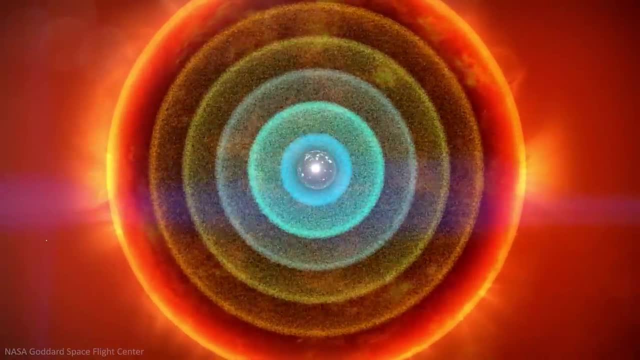 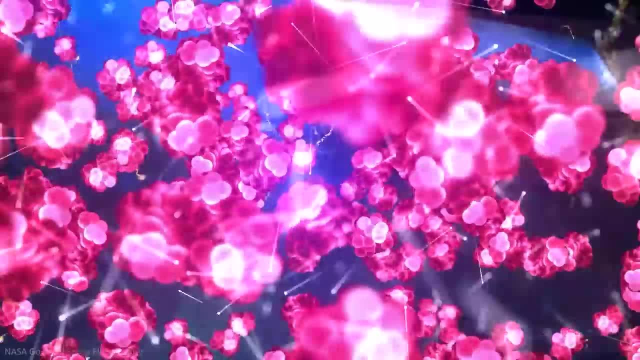 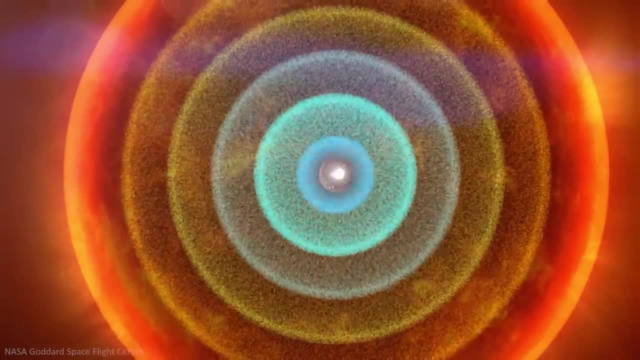 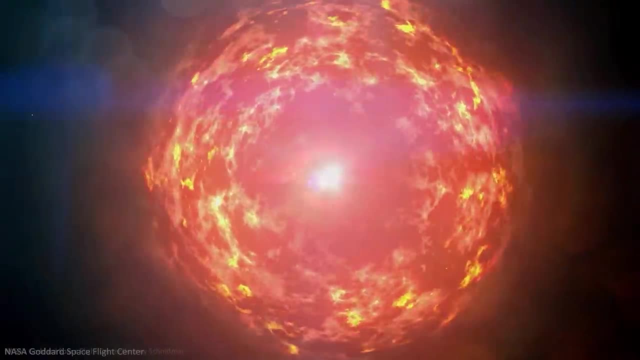 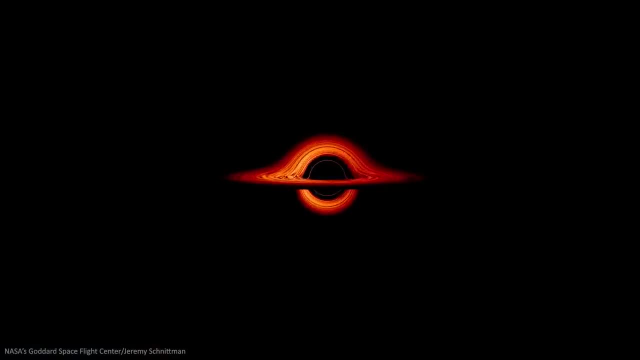 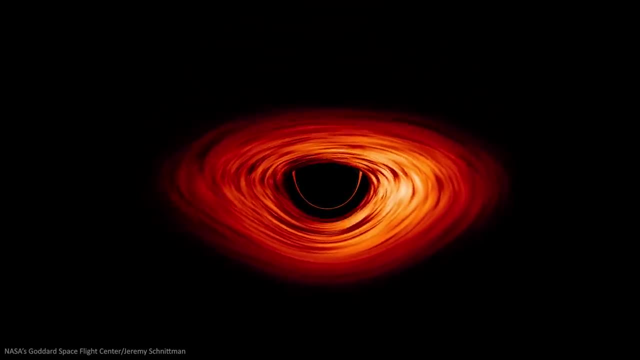 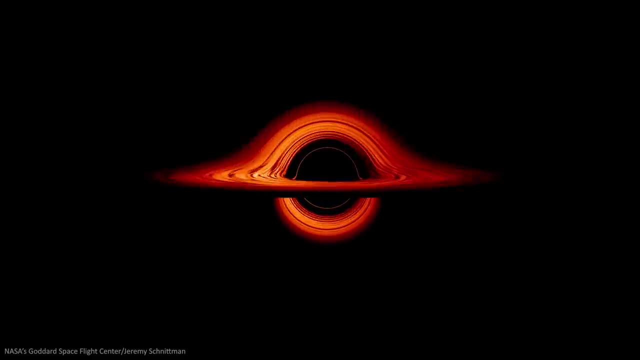 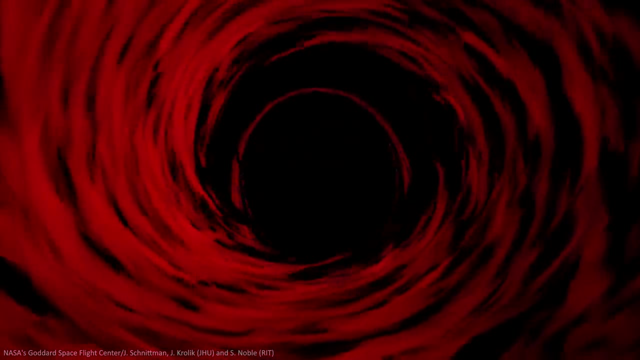 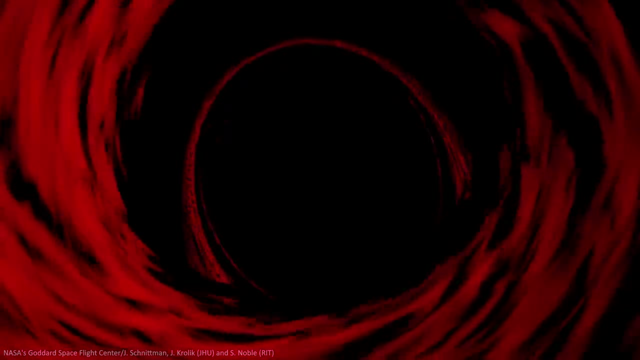 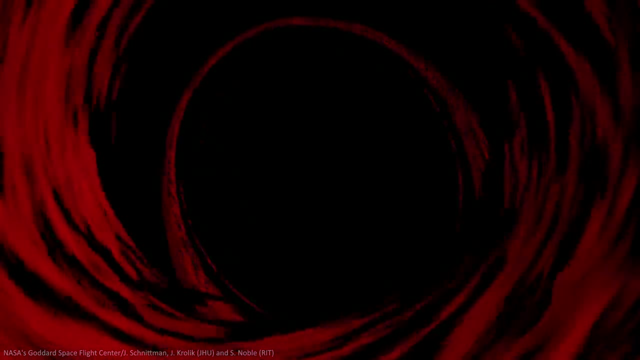 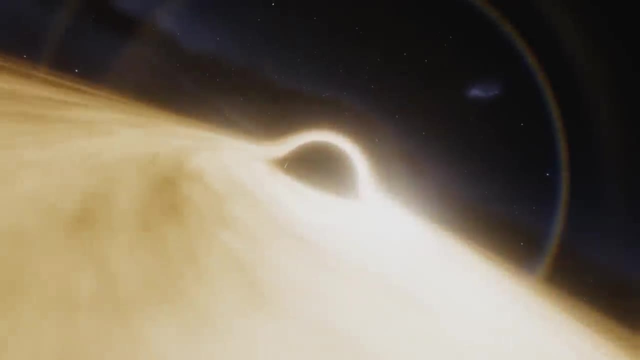 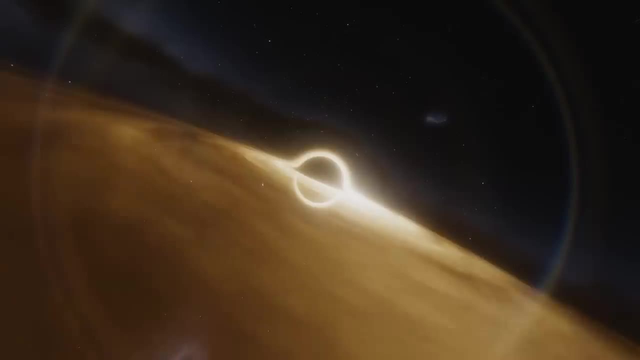 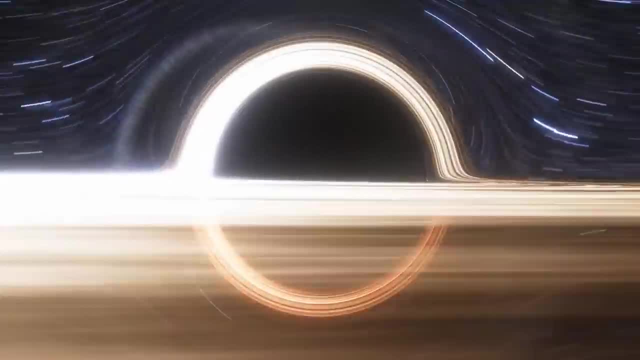 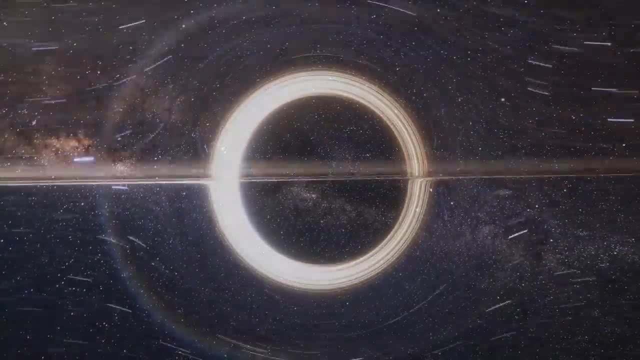 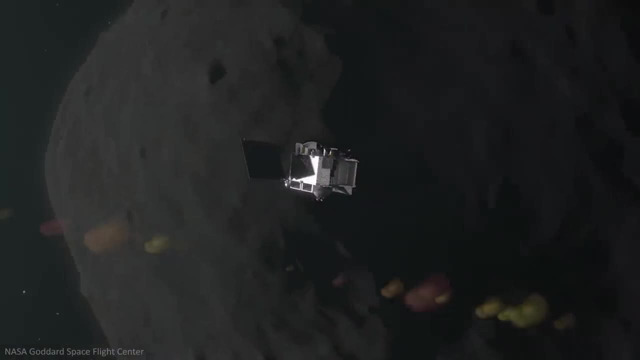 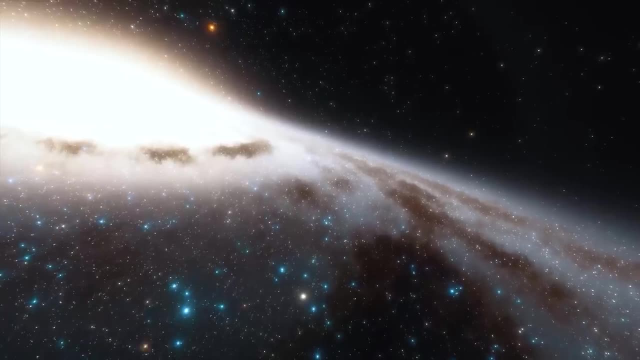 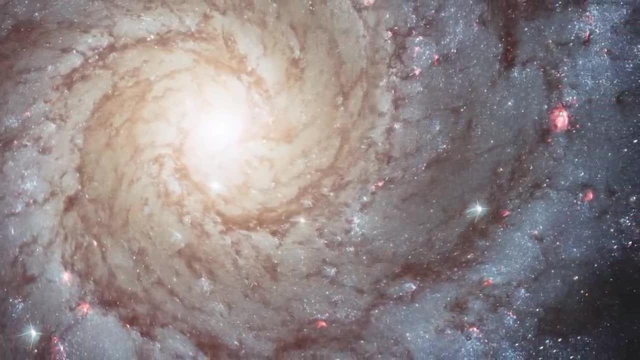 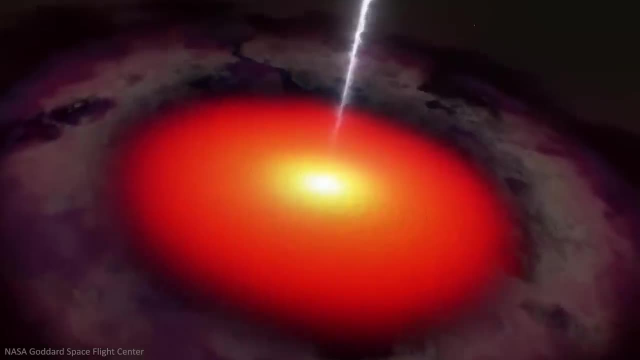 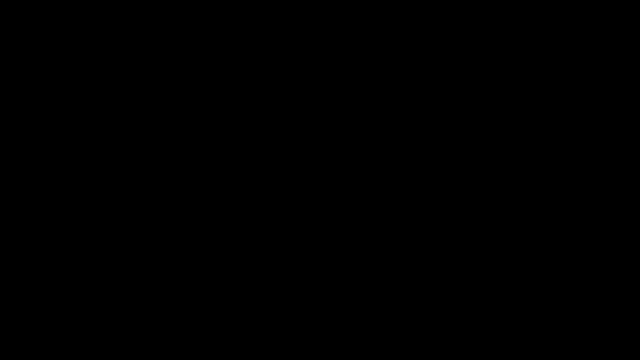 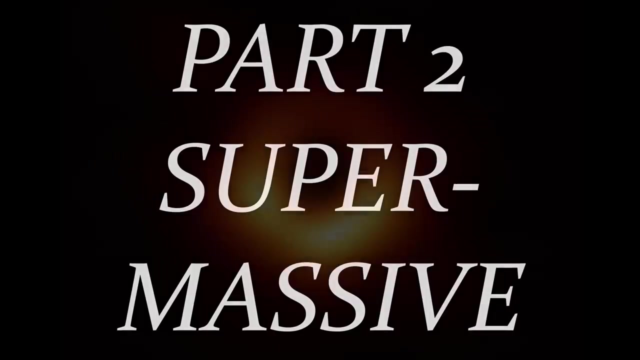 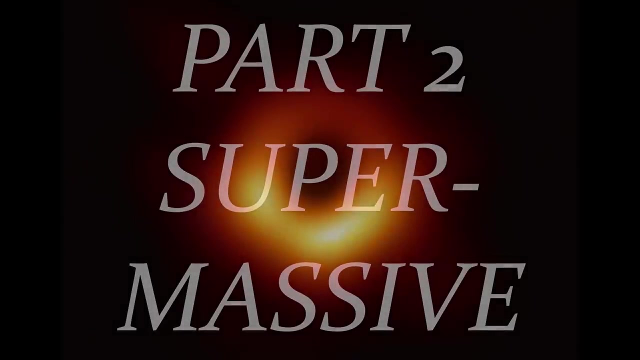 much, much more mysterious. April 10th 2019.. A picture sweeps the globe, instantly becoming a viral sensation. Unlike most viral images, this one wasn't visually impressive on its own. It was fuzzy and indistinct: An orange torus on a plain black background. 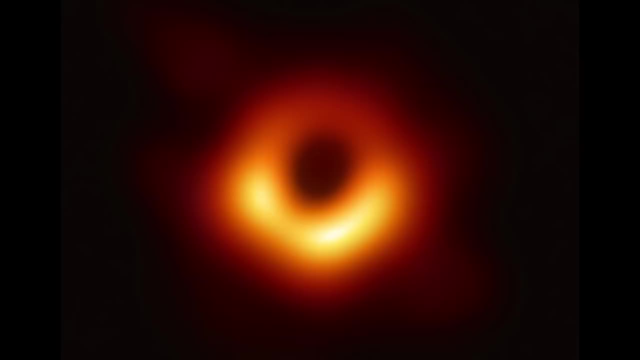 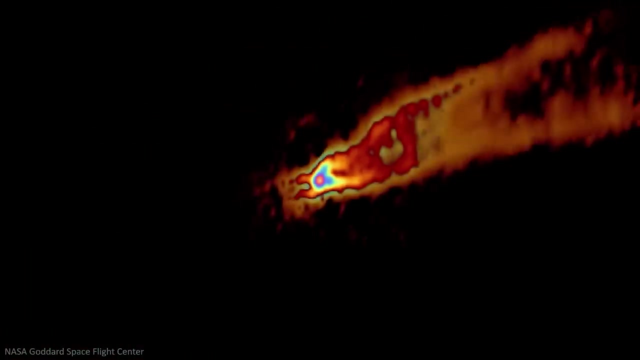 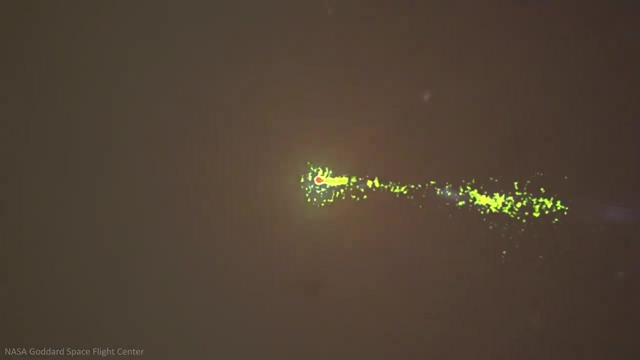 But it nevertheless represented the work of hundreds of scientists over half a decade. Just a few weeks later, more than a billion people had laid eyes on the very thing that physicists had refuted for years and which most astronomers never expected to see directly outside of their imaginations. 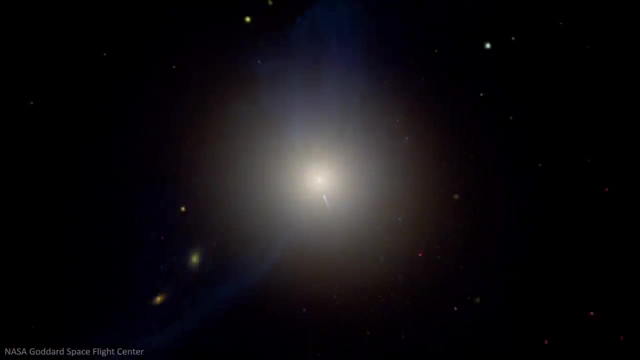 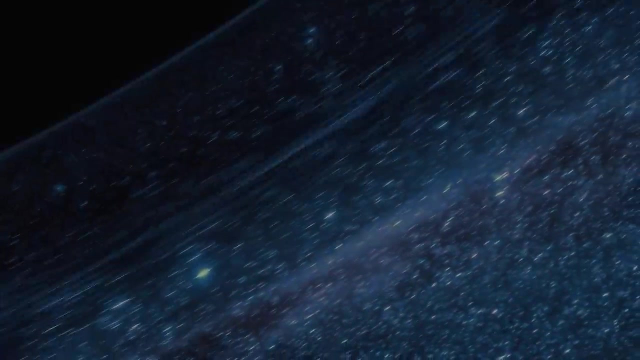 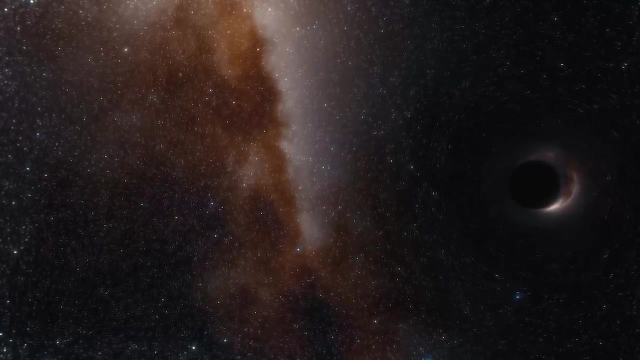 It was, of course, the first ever image of a black hole. Black holes, as their name and very definition dictate, are black. At first glance, this makes the prospect of photographing them seem like a fool's errand. But scientists have seized upon the voracious nature of these gravitational chasms and 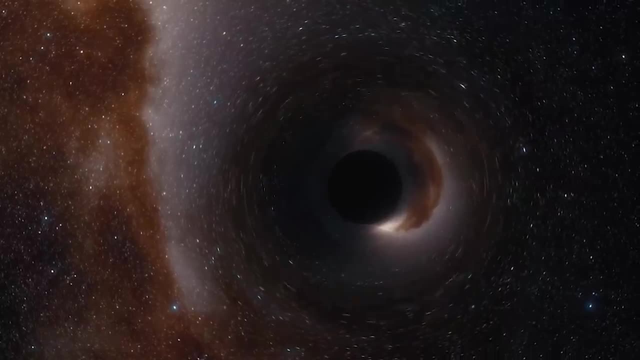 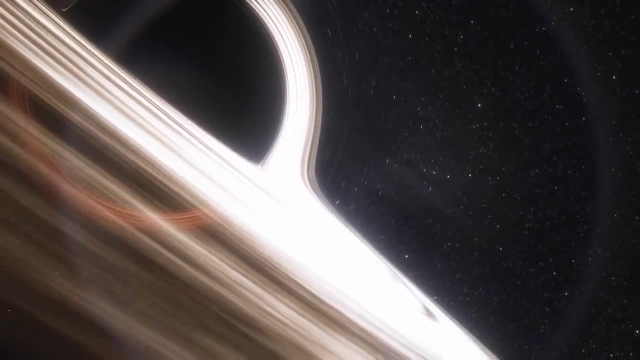 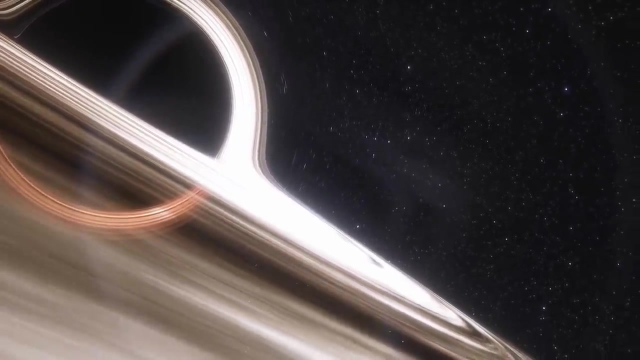 their effects on the matter that surrounds them. A sufficiently massive black hole surrounded by a sufficiently large disk of gas and dust theoretically gives off enough radiation in the form of high frequency radio waves to be detected by a sufficiently large radio telescope here on Earth. 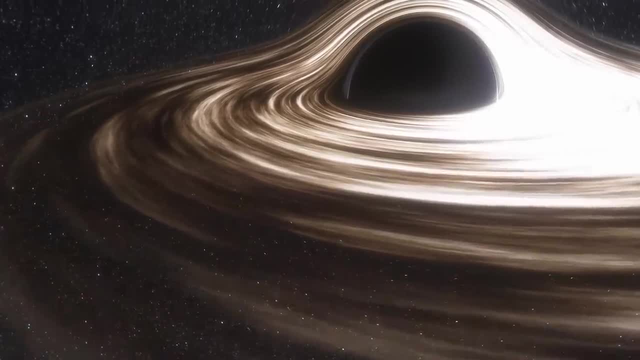 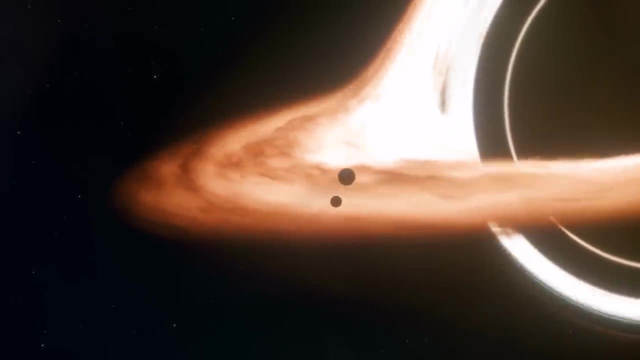 These black holes needed to be more than massive. They had to be supermassive- The name for a black hole that weighs millions or even billions of times that of our sun. Astronomers believe that these leviathans reside at the centre of most large galaxies. 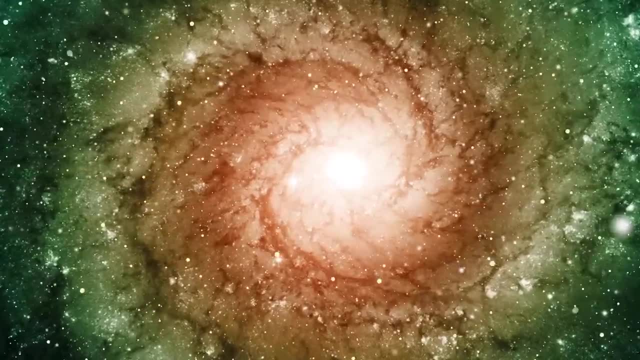 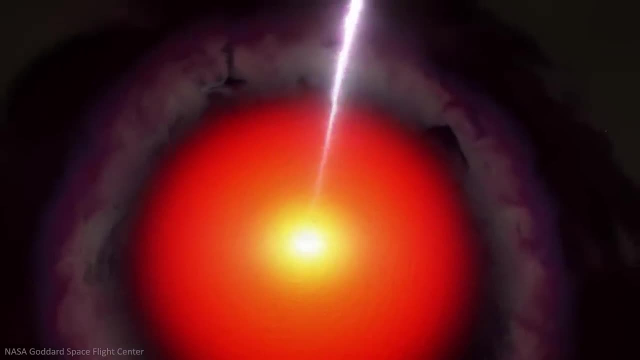 And indeed may be crucial to the formation and evolution of the galaxies themselves. As they feed and grow, the supermassives occasionally change their shape, But they don't always change. Supermassives occasionally spit out accelerated globs of gas, counter-intuitively helping. 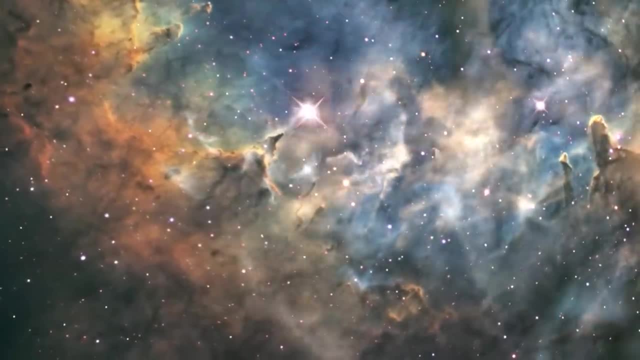 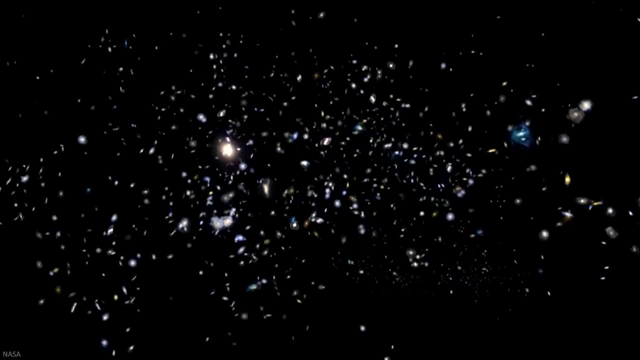 stars to form just at the moment of others' death. The link is so strong that some astronomers have begun to grapple with the question of which came first. Did the earliest galaxies feed and fuel supermassive black holes or did the supermassives already? 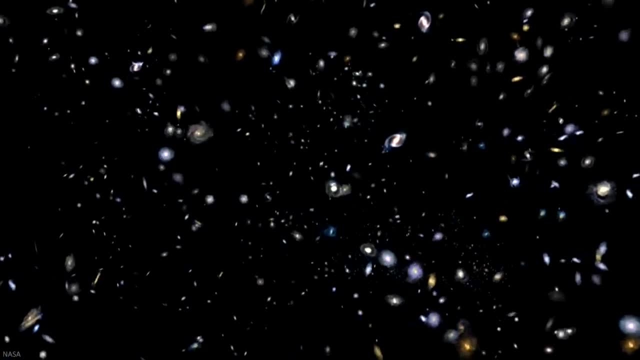 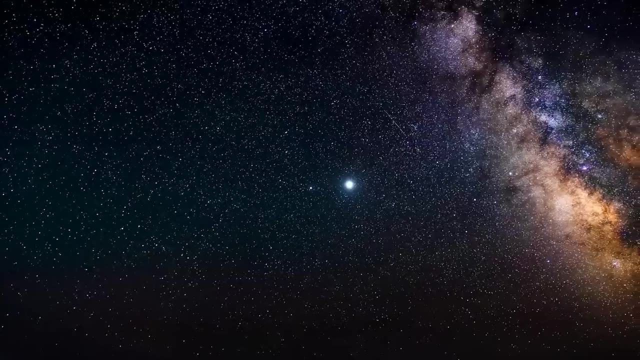 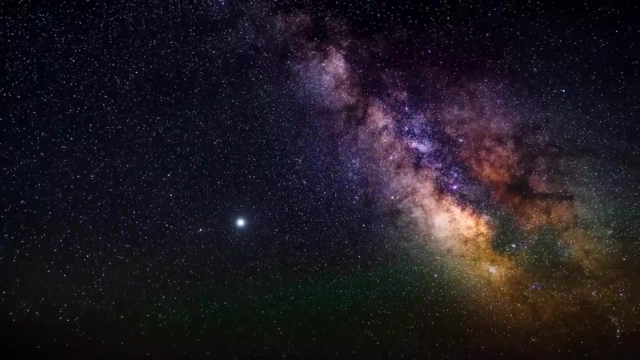 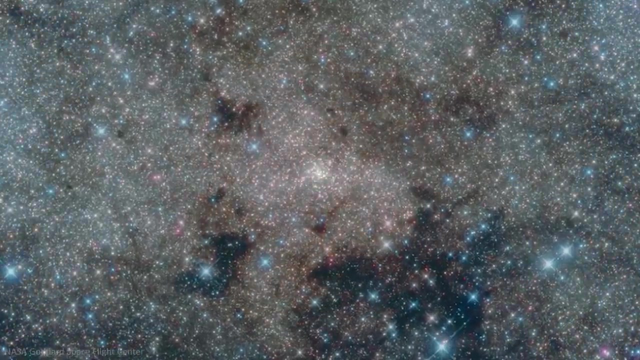 in existence somehow seed the stars and galaxies of our modern cosmos. So in searching for the ideal supermassive candidate, the black hole imaging, scientists needed only to turn to the heart of our own Milky Way. Here the supermassive black hole known as Sagittarius A-star looms 25,000 light-years. 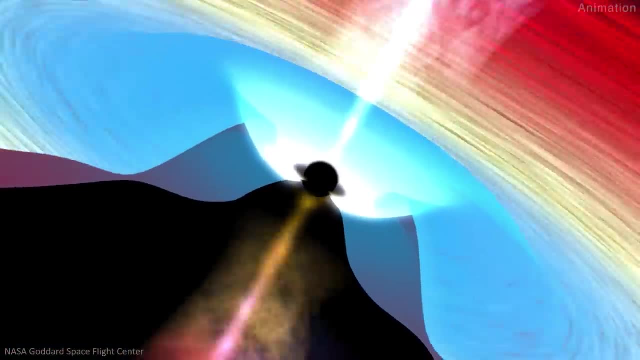 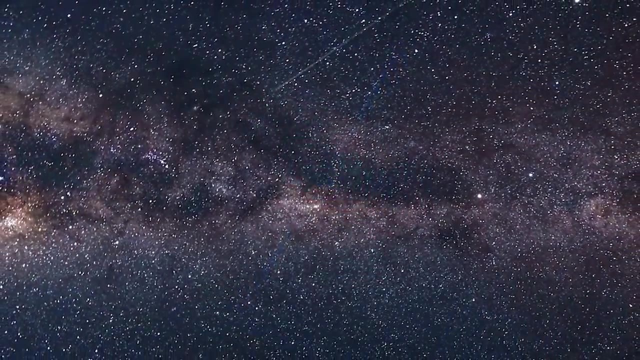 away from Earth with a mass of some 4 million suns. Its relative proximity may have made it an obvious target, but that nearness also brought with it additional problems. Embedded as it is within the Milky Streaker galaxy, the black hole is the largest black-hole. 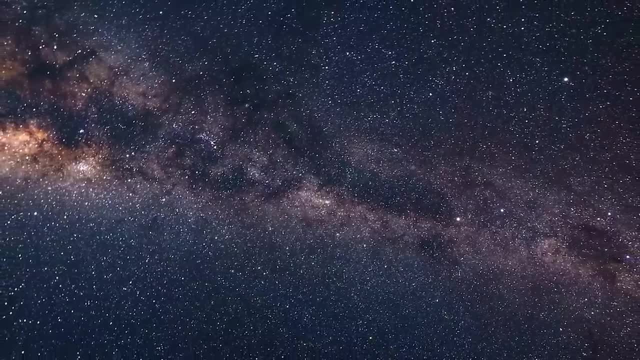 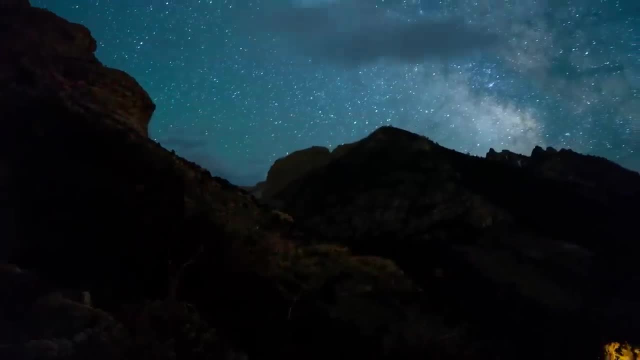 in the universe. In addition to the number of stars that give our galaxy its name, there are countless celestial objects blocking a clear view of the supermassive black hole. Not only that, but as the Earth turns, so the centre of the galaxy sweeps across the 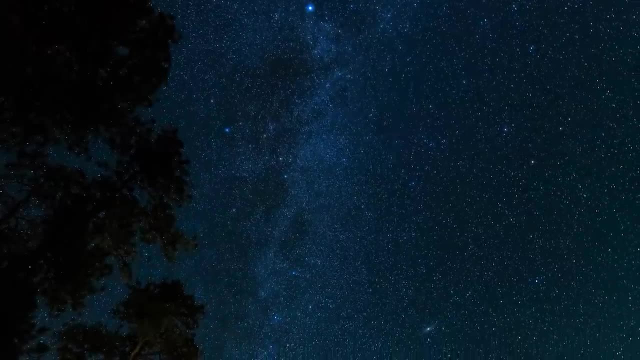 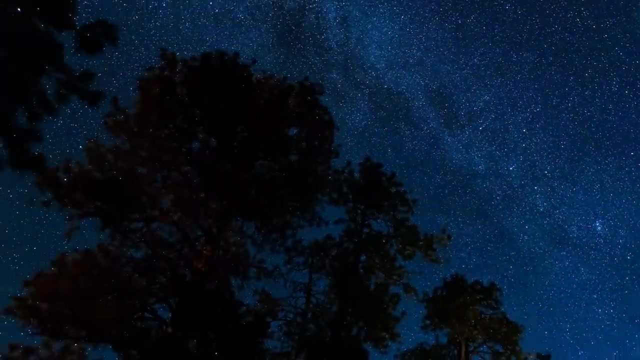 sky each night. it would be very difficult to maintain a telescope fix for long enough to gather the necessary data. Therefore, to begin with, the international team of scientists set their sights on a more distant supermassive, This time residing at the centre of the Messier 87.. 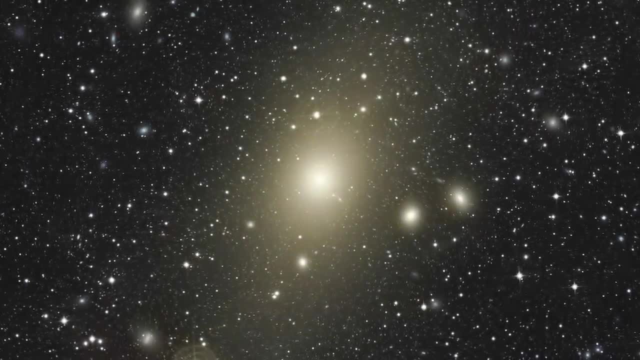 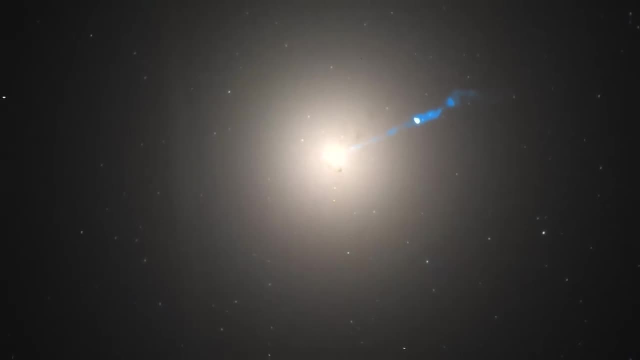 The Messier 87 is the largest supermassive galaxy in the world. It is the largest supermassive galaxy in the Virgo Cluster. At first this may seem odd. M87 is some 55 million light-years away, far further than. 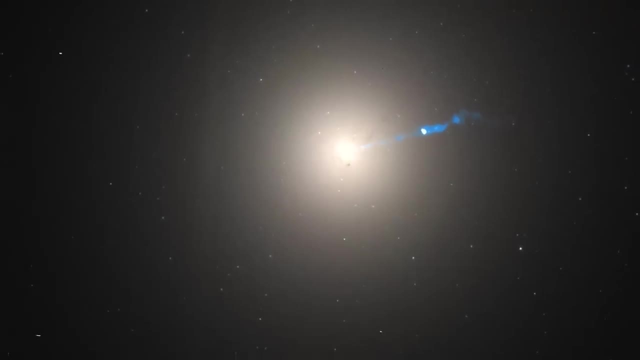 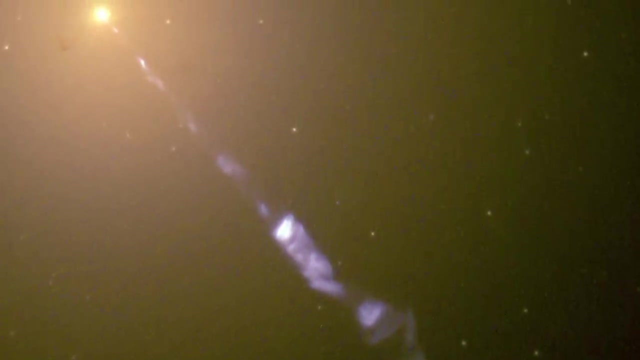 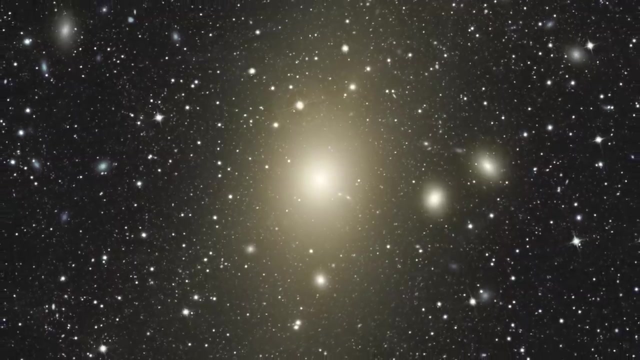 the mere 25,000 light-years to Sagittarius A star, but its sheer size made up for the distance, for M87, weighs an incredible 6.5 billion times our sun's mass. Also, at such a distance, it stays relatively still. 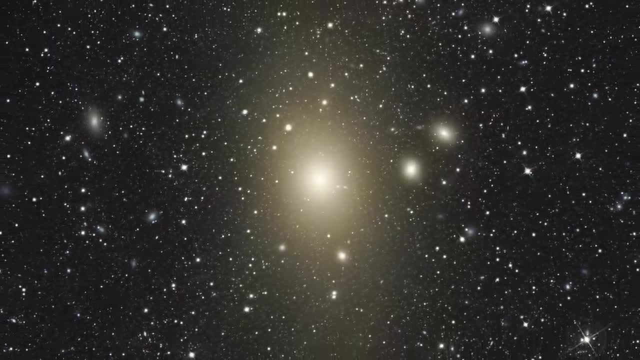 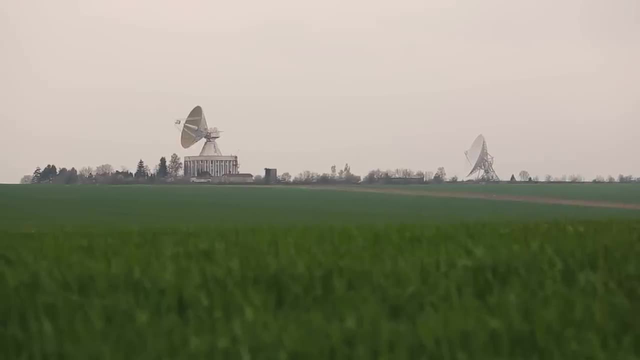 There is a clear line of sight all the way. The next challenge, however, was to actually build a telescope that was big enough to reveal M87's blackened core In radio astronomy. the resolution of the final image obtained depends on the size of 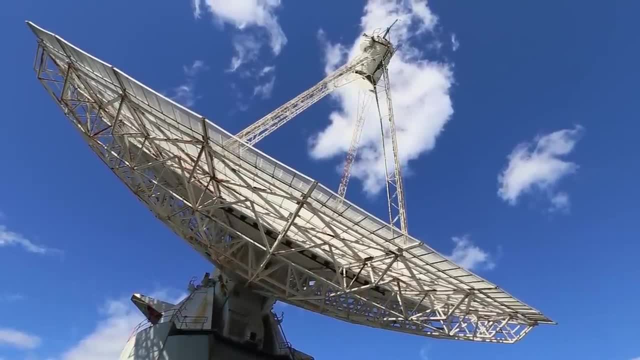 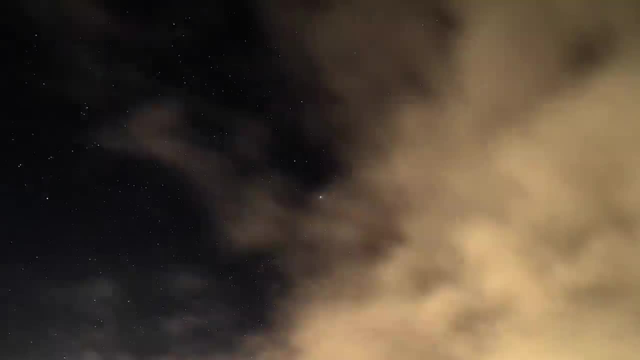 the telescope aperture that collects the radio light. This means that for small and distant objects, bigger is always better, leading to some fairly on-the-nose names for modern high-resolution radiotelescopes. This means that for small and distant objects, bigger is always better, leading to some fairly 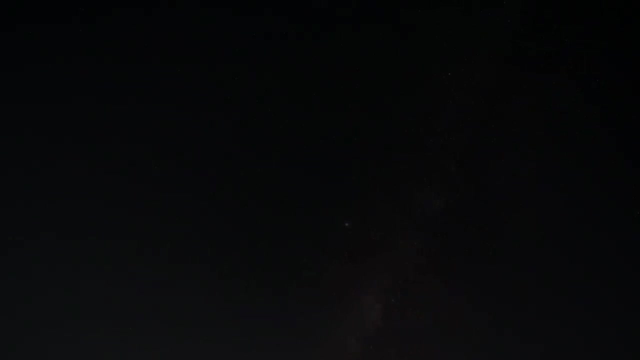 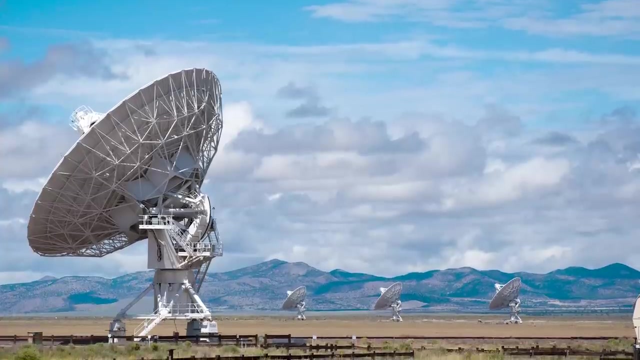 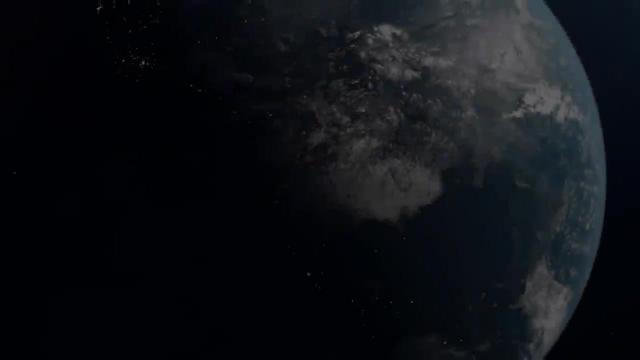 on-the-nose names for modern high-resolution radiotelescopes: The giant Ukrainian radio telescope, The large millimetre telescope, The very large array, But for M87, even very large- was not large enough. The radio telescope would have to be roughly the size of the entire Earth. 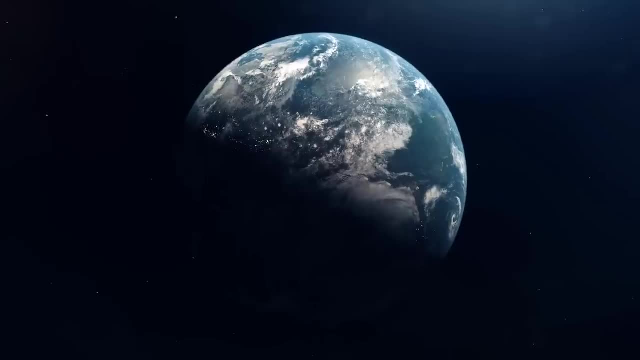 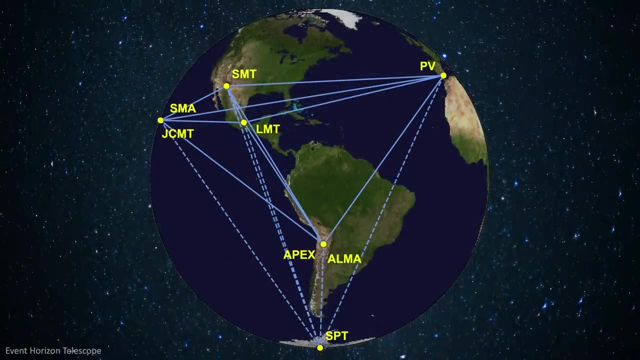 And so researchers worldwide collaborated to connect eight radio telescopes from across the globe, Forming a composite telescope with an aperture that spans 1.5 million light-years, With an aperture that spanned from the South Pole to Spain And a resolution around 4,000 times better than the Hubble Space Telescope. 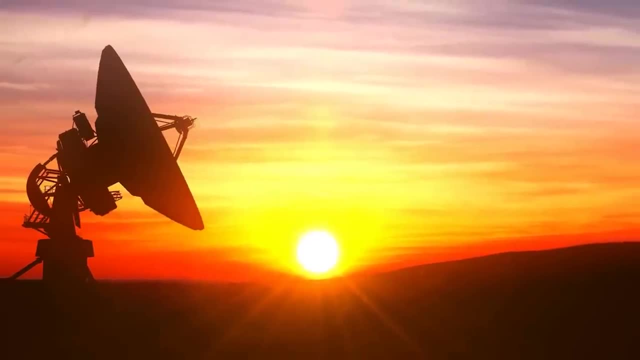 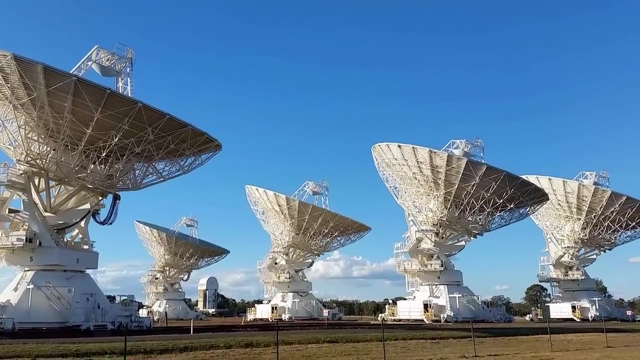 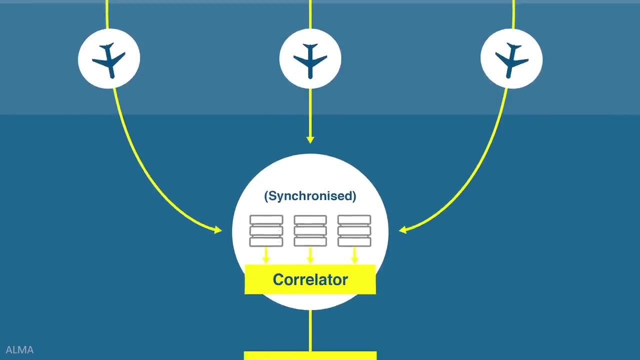 This so-called Event Horizon Telescope, with its component parts synchronised by atomic clock, collected radio waves from the direction of M87 for four days in 2017.. The observations from each monitoring station were delivered on physical hard drives, since internet speeds were unable to cope with the volume of data. 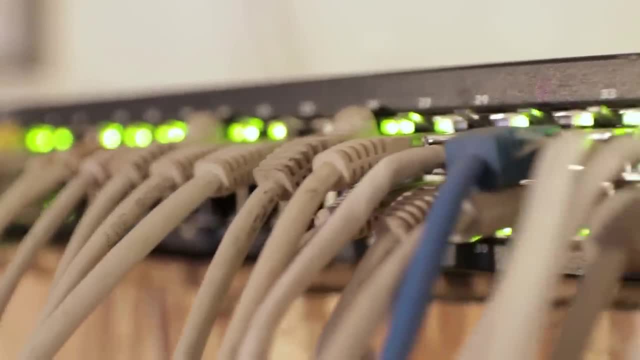 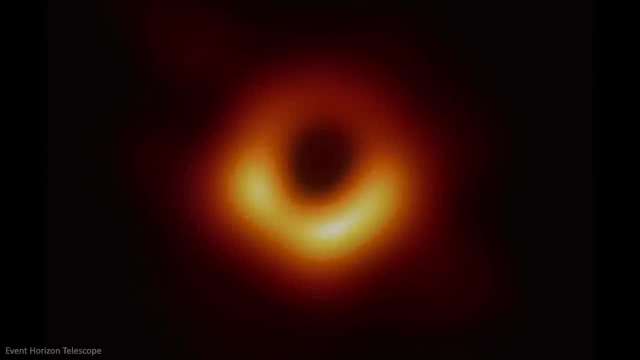 Two years of intensive data processing later and the team finally had their impossible image: A silhouette of the M87 supermassive's black hole event horizon lit by the radio light of its accretion disk. But the discoveries didn't stop there. 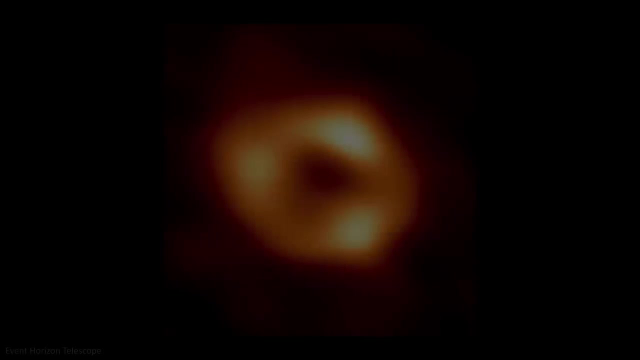 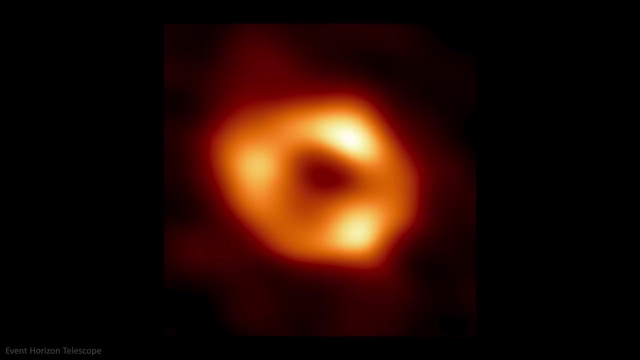 In May 2022, after an additional three years of processing data from the Event Horizon Telescope's initial observations of the Milky Way were finally resolved into the second-ever image of a black hole. We finally caught a glimpse of the beating heart of our own galaxy. 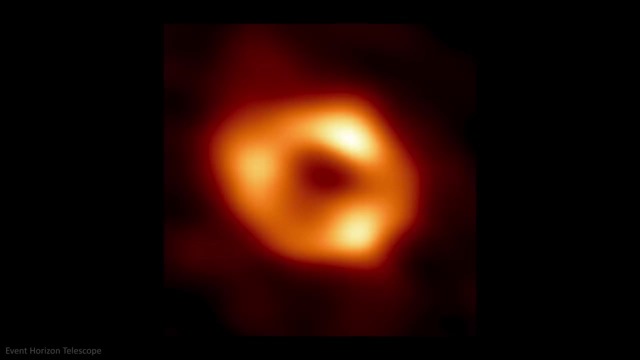 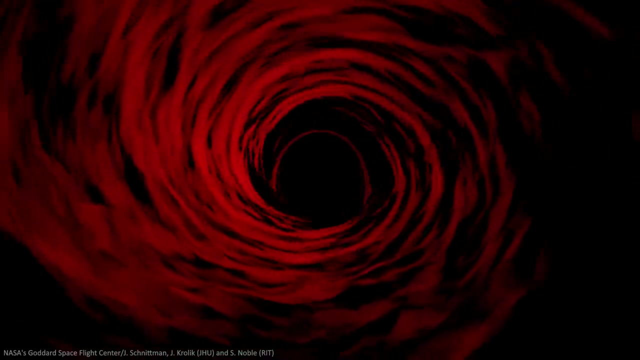 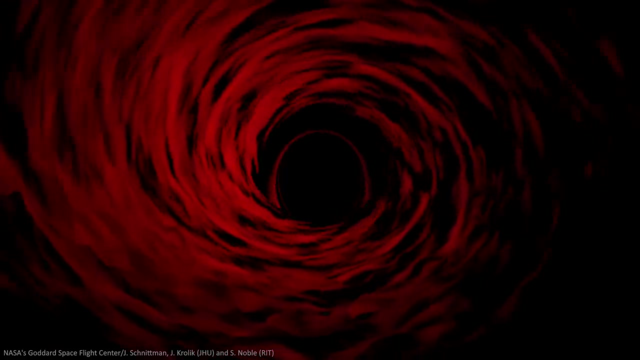 Sagittarius A-star Imaging and analysis continues to break new ground in visualising and understanding these supermassive black holes, But there are still so many unanswered questions surrounding their lives and, crucially, their formation. Just how does a black hole get away from the surface? 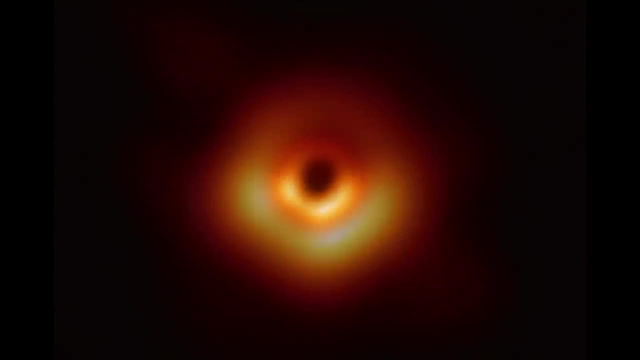 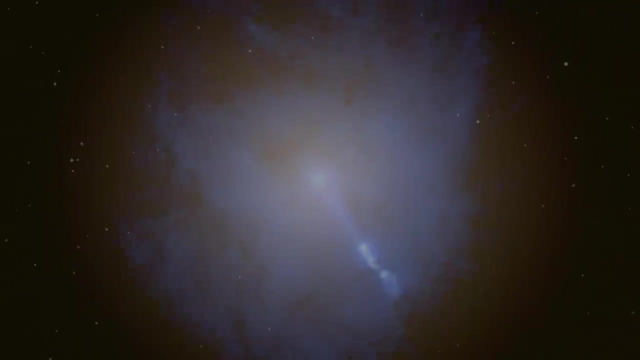 How does a black hole get away from the surface? Does it get away as much as M87 does, Or, more Indeed, 6.5 billion times the mass of our sun doesn't even come close to the largest black hole we've found. 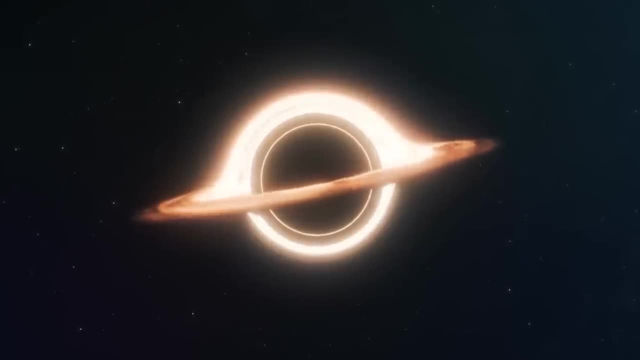 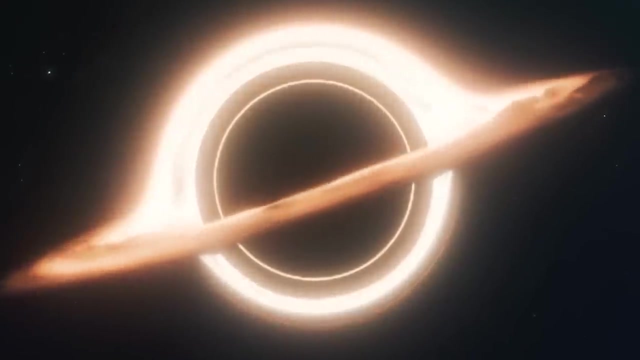 TON618,, belonging to a quasar 10.4 billion light years from Earth, tips the balance at an incredible 66 billion solar masses, making it a so-called ultramassive black hole. It alone is heavier than all the stars. 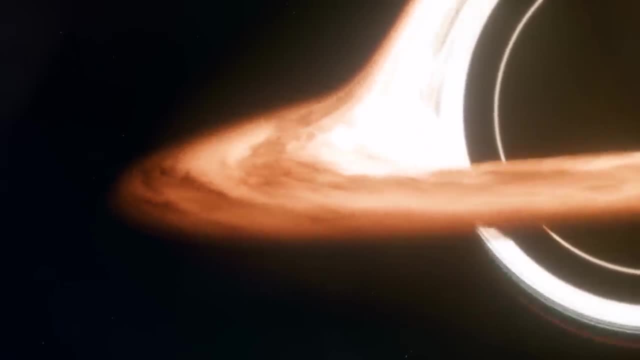 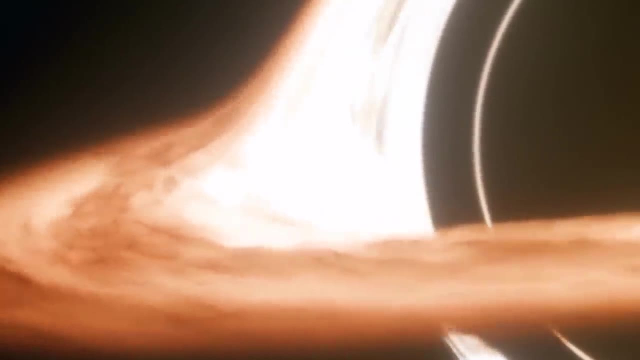 It is about 99% heavier than all the stars in the Milky Way combined, and with accretionary winds that reach 20% the speed of light. it consumes matter at such a rate that its luminosity exceeds that of all the stars in its galaxy. 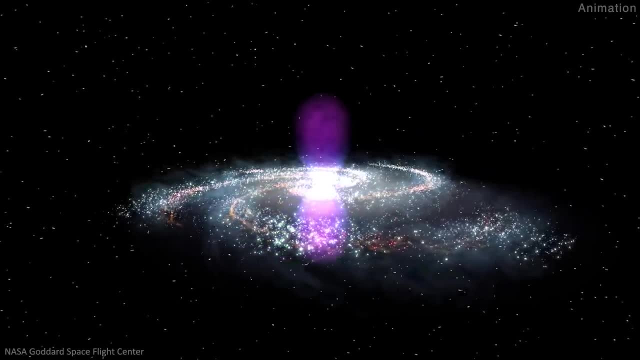 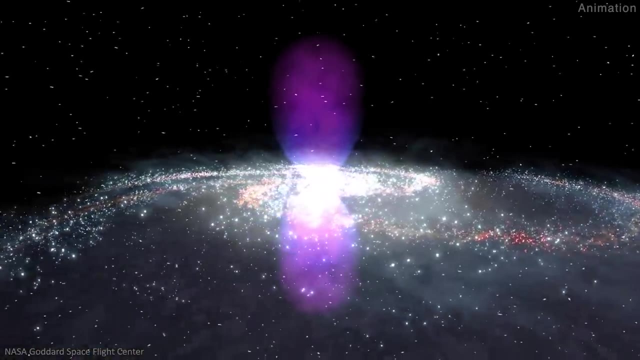 When astronomers detect quasars- the brightest objects in the universe- they are detecting these super or ultramassive black holes with inactive galactic nuclei. They are arguably the most impressive single objects in the entire galaxy. That's why they are called quasars. 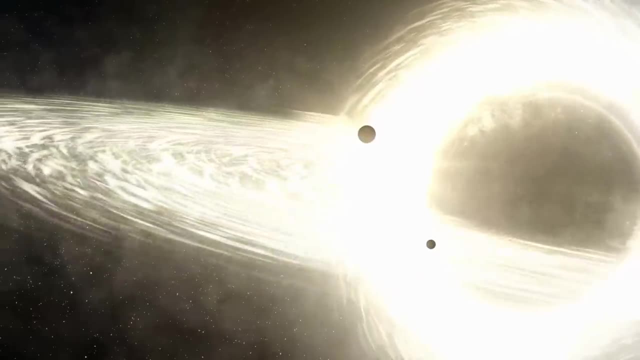 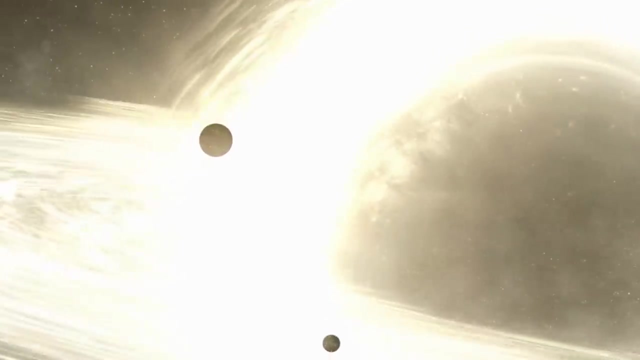 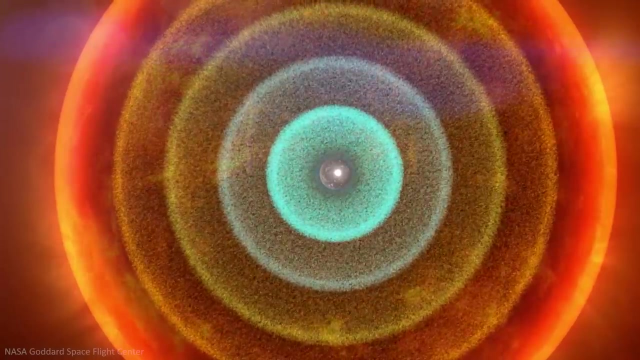 But how do they detect quasars? entire cosmos, But how did they form? Some suggest that these heavyweights started out just as their stellar black hole cousins. A gigantic star lived, died dramatically and left behind a bulky black hole in its 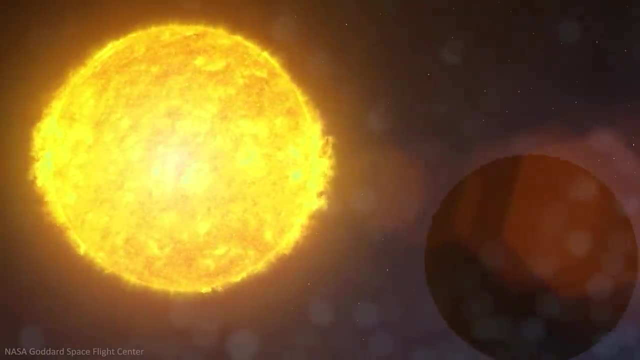 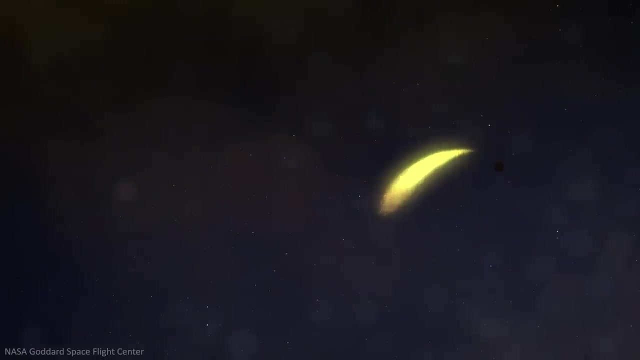 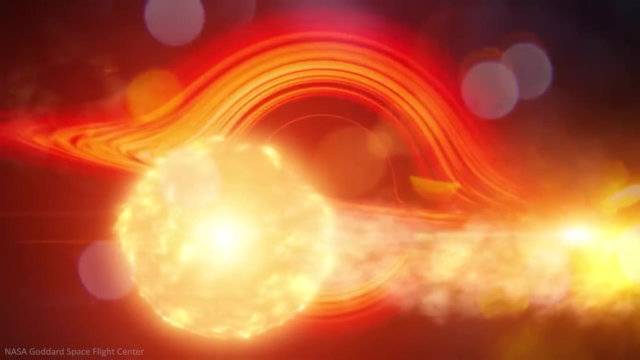 wake. Then, over a period of billions of years, that gravitational titan got lucky, encountering star after gigantic star to feed its insatiable hunger, growing gradually until it attained mammoth proportions and ensnared entire star systems into stable orbit around it. 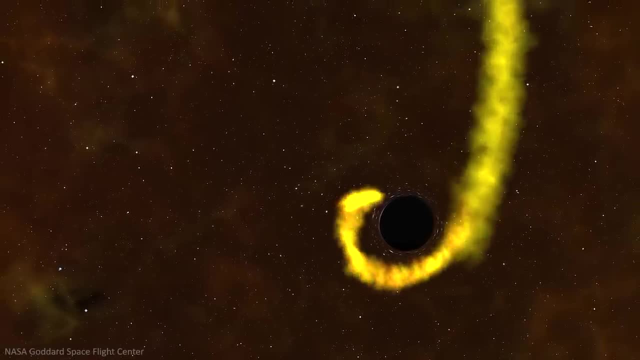 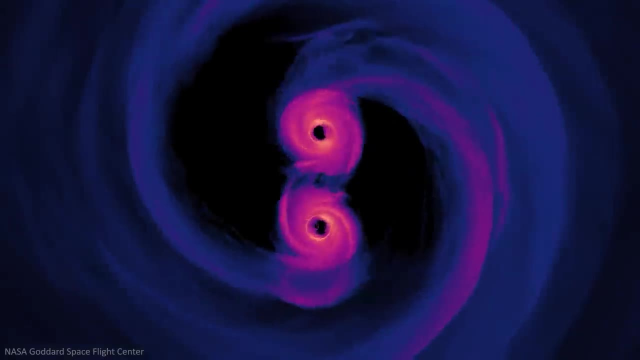 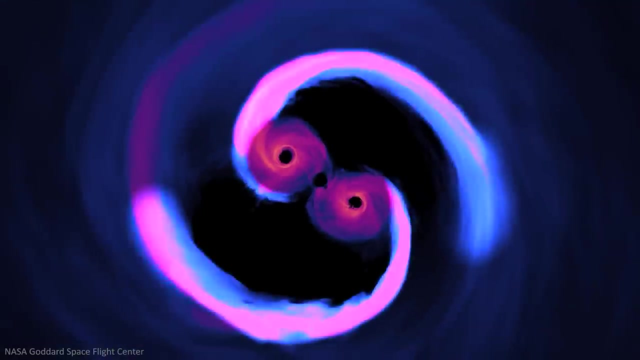 But critics fail to see how such growth could be accomplished by gradual means alone and suggest a much more staggered approach. Instead of a single voracious beast consuming stars and gas, alternative theories see supermassives born in mergers between several smaller stellar masses. 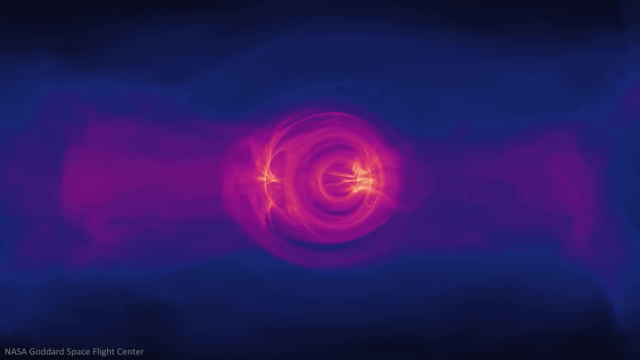 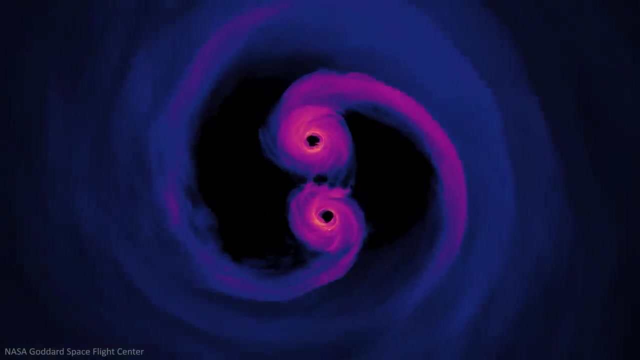 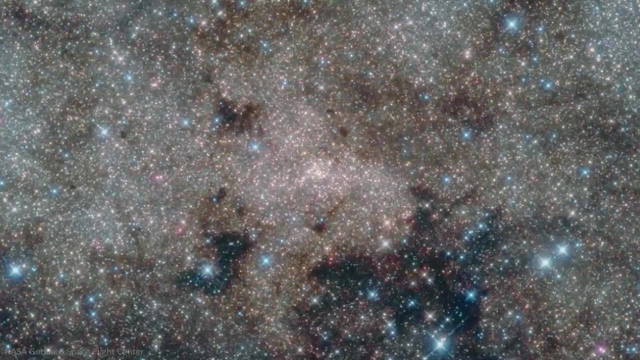 Indeed, such mergers have already been observed by the gravitational waves that ripple out from them. It would certainly be a shortcut to acquiring mass, but questions remain as to how likely these binary black hole encounters are. Perhaps our continued observation of the supermassive black holes in our galactic neighbourhood will. 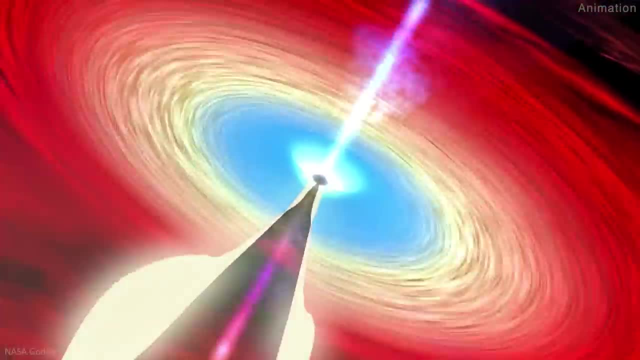 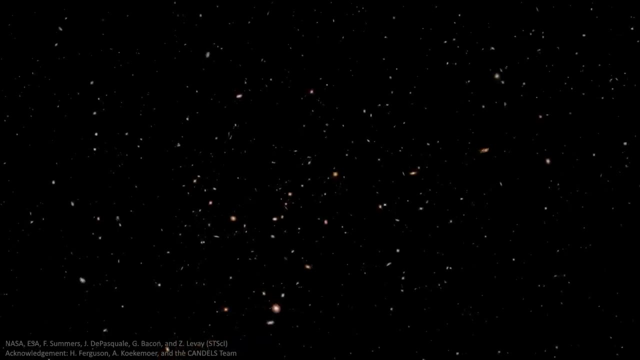 help to answer these questions, But there is one overarching mystery that stands regardless. When we peer back into the galaxy, we can see that the black holes in our galaxy are still there. In the distant, and consequently ancient, cosmos, we still find supermassives. 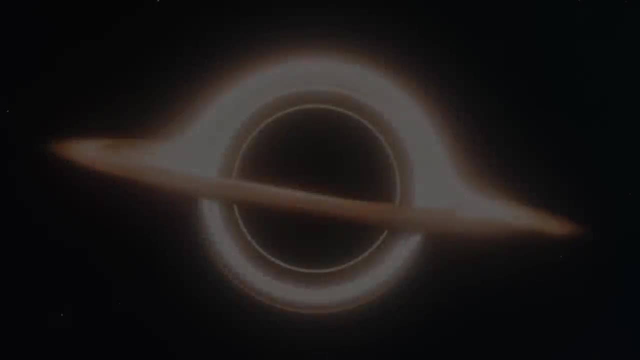 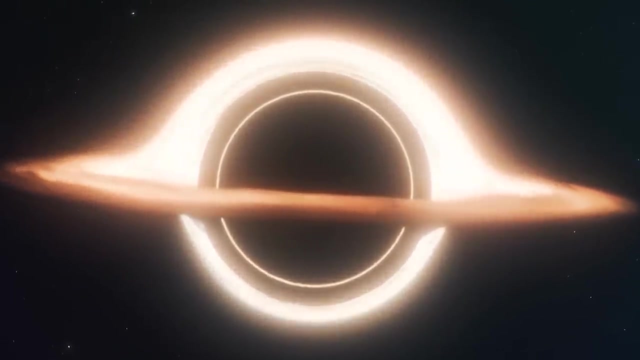 The ultramassive black hole TON 618 is nearly 11 billion years old, and many supermassive black holes have been detected dating back to just a few million years after the big bang. So if they assembled gradually or through repeated mergers of stellar black holes, their 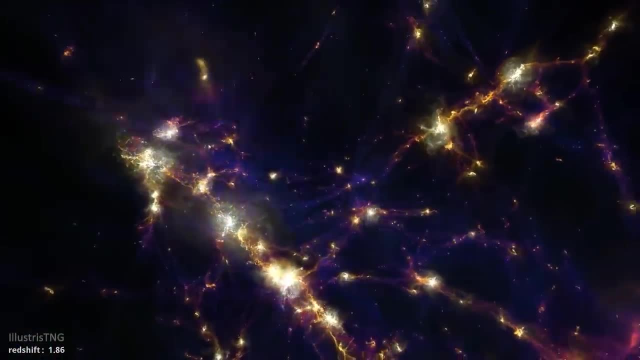 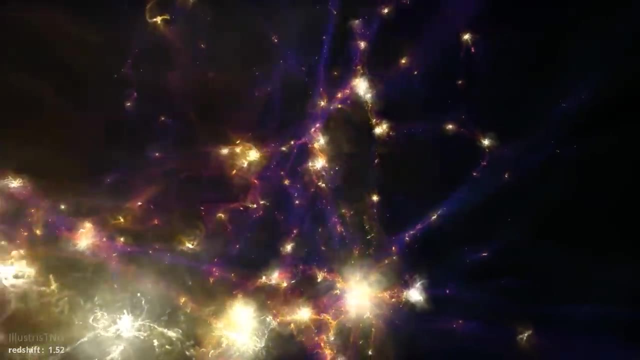 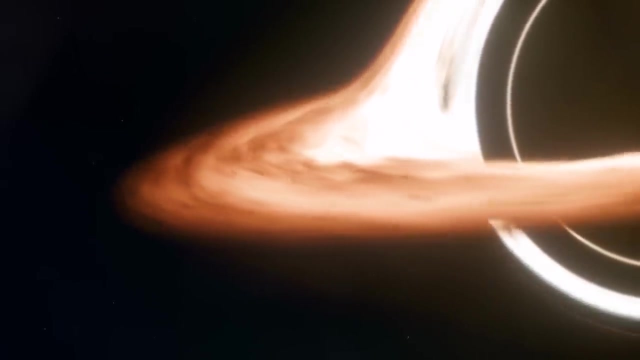 presence so soon in the cosmological timeline implies that innumerable stars have already lived and died. And here is where the problem lies: Plugging in the masses of these early supermassives and the well-constrained estimates of star formation in the earliest phase of stellar growth, these supermassive black holes just 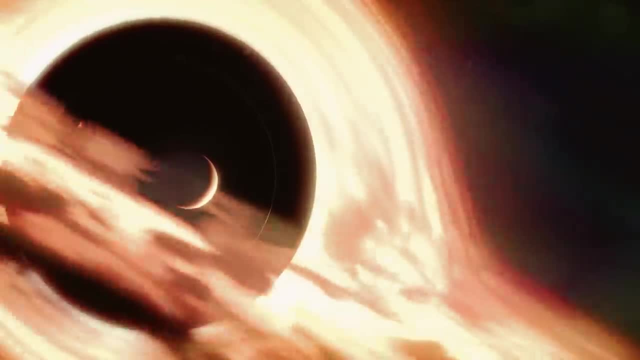 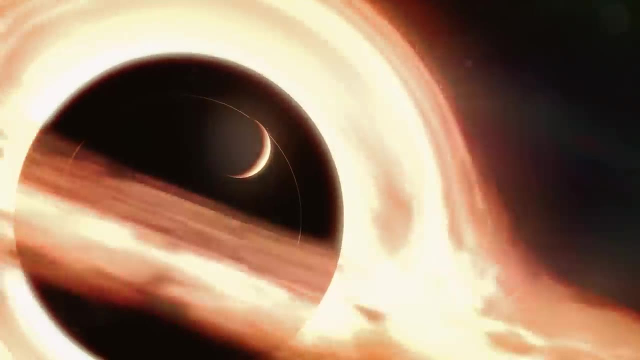 shouldn't be possible. Some giants had grown to 1 billion times the mass of our sun by less than a billion years after the big bang, But calculations show that only 100,000 solar masses should have been formed. The mass of the sun is only 1 billion times the mass of the sun. 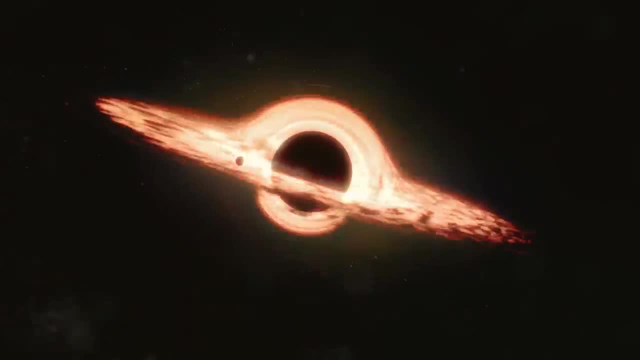 The mass of the sun is only 1 billion times the mass of the sun. It's seen as a 만th salesman on the complex. as the mass of the solar masses should be possible, a difference of 4 orders of magnitude. 3 cântu patriot Heals, chunk 2. 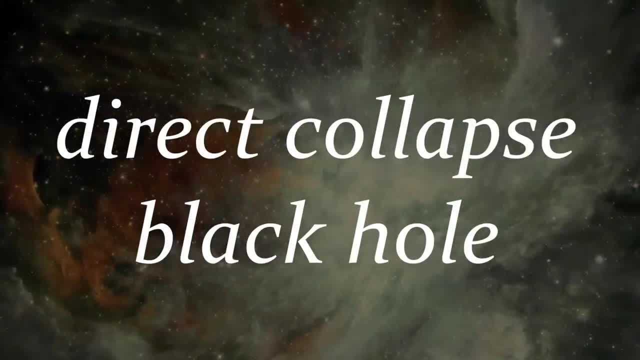 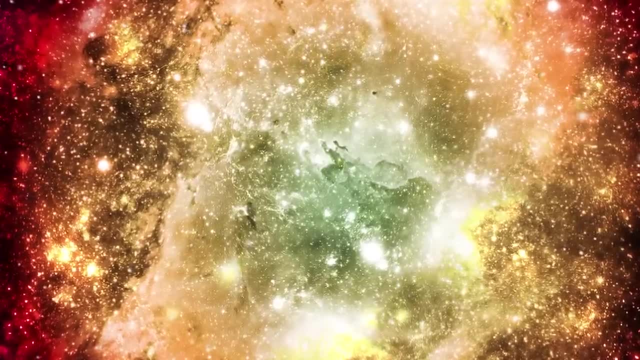 There is another phenomenon, called a direct collapse black hole, that could offer at least a partial explanation. Instead of forming during the death of a star, as with stellar black holes, direct-collapse singularities form, as their name suggests, directly from the collapse of material in 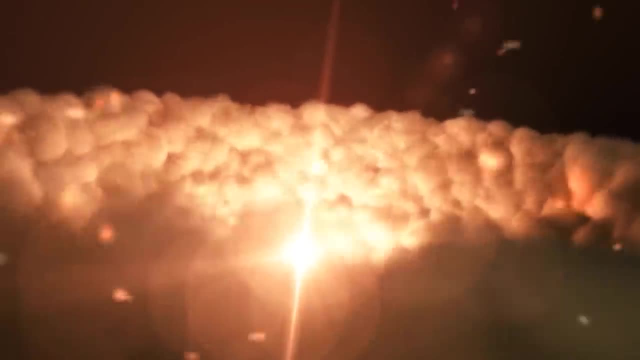 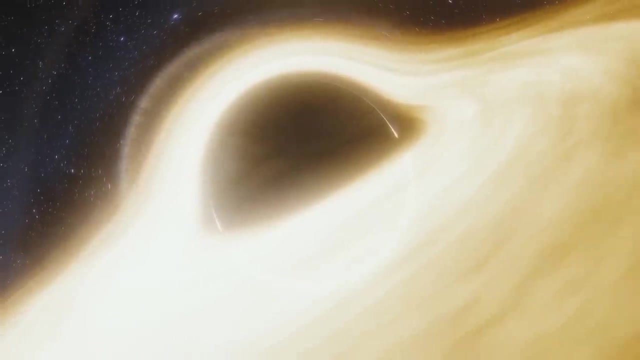 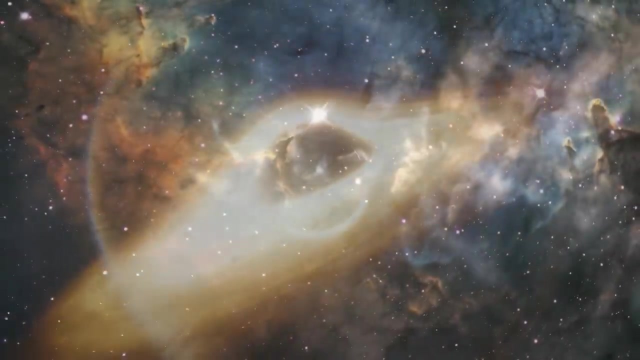 the early universe C aerGG Type Cumen formation. Such early high-mass black holes could be the beginnings of the supermassives we see today, But they probably aren't the ultimate solution. The conditions for their formation are so restrictive that they were likely rare phenomena and not enough to explain the 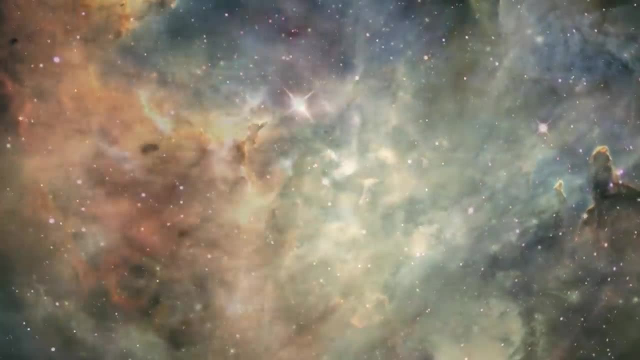 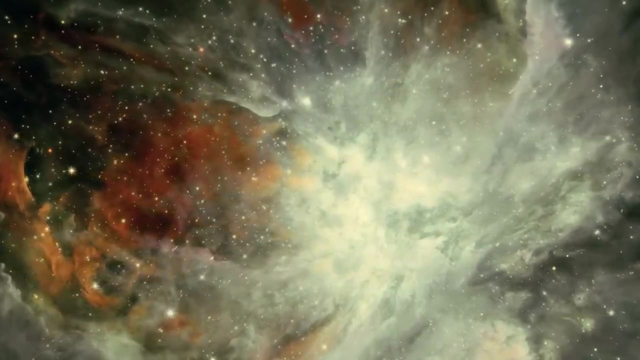 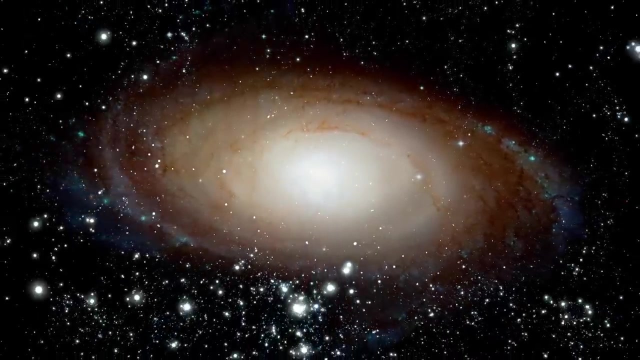 supermassive shepherds and their galactic herds that fill the universe today. There must be another piece to the puzzle Lurking back at the dawn of time. there must be something, Something that helped to feed these giants from their birth and help them to grow into the black. 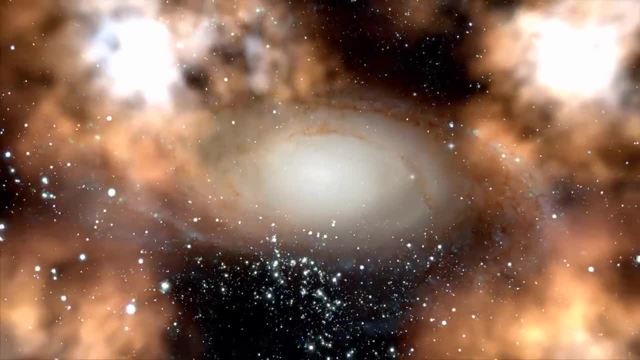 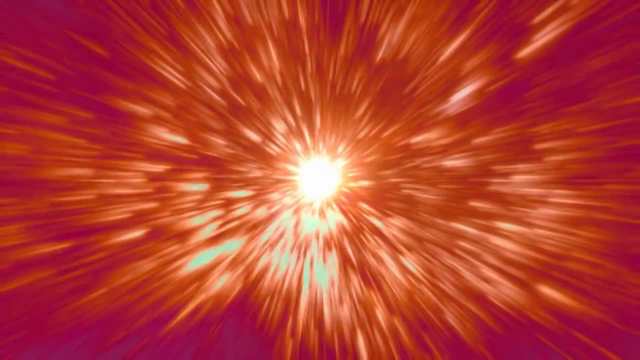 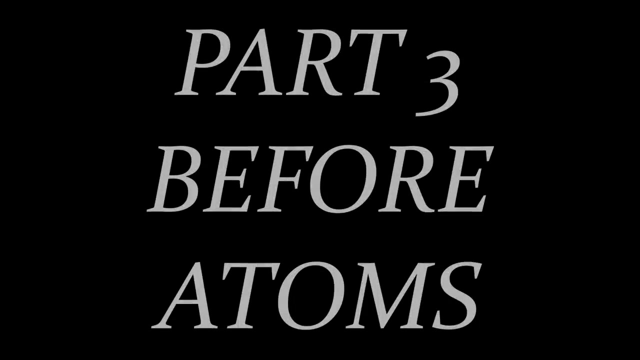 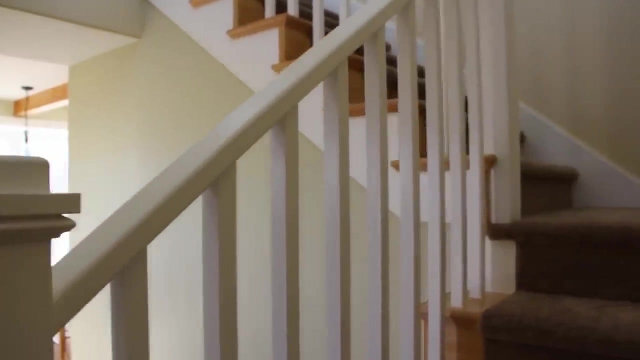 behemoths that power our galaxies today, But what could create a black hole before stars are born? When a 20-year-old undergraduate student first fell down the stairs in Oxford in 1962, his doctors helpfully told him to lay off the beer. But when this clumsiness continued into 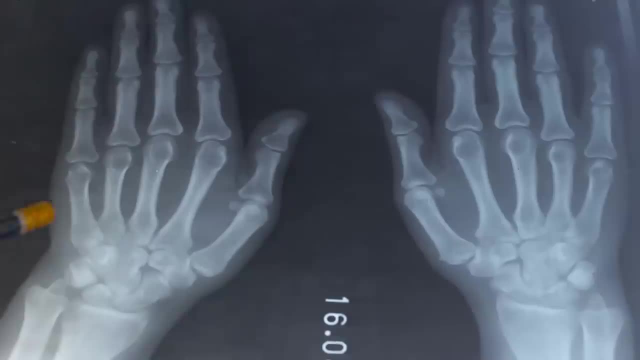 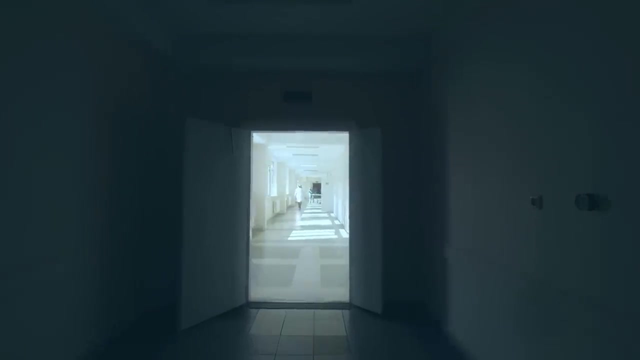 the next year, his family began to worry and the young scholar was sent to hospital for a series of tests. After two weeks of rigorous investigations, the physicians still didn't tell the young man what was wrong with him, except that he was an atypical case and that he was a man of 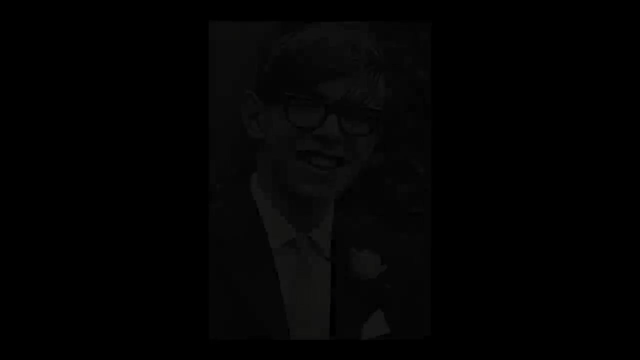 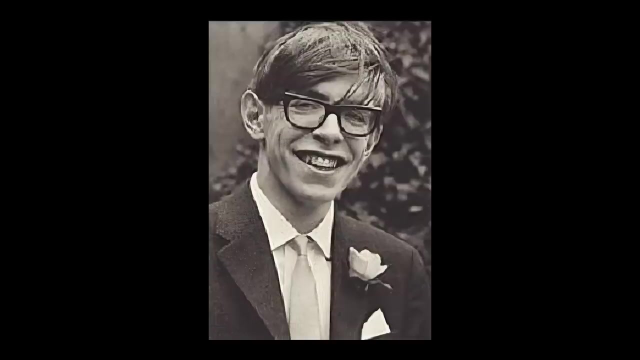 and they expected it to get worse. Reluctant to ask for more details, the young Stephen Hawking simply took the vitamins the doctors recommended, even though he could see in their eyes that they didn't expect them to work. By this time, Hawking had begun his postgraduate studies at the 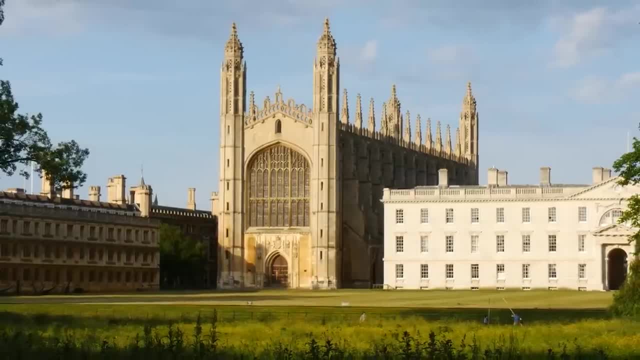 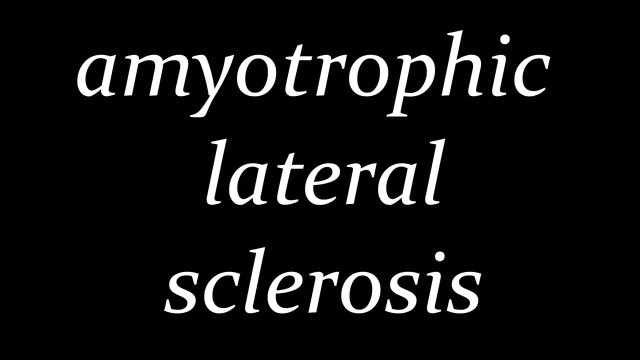 University of Cambridge. The medical diagnosis he had avoided facing was one of amyotrophic lateral sclerosis, or ALS, which sees the motor neurons in the brain rapidly degenerate until they are completely gone. The doctor's diagnosis was that the young Stephen Hawking 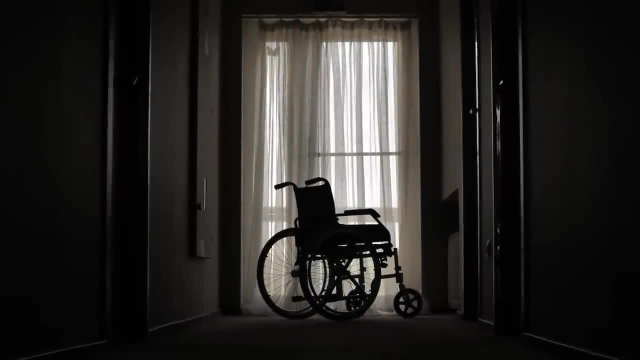 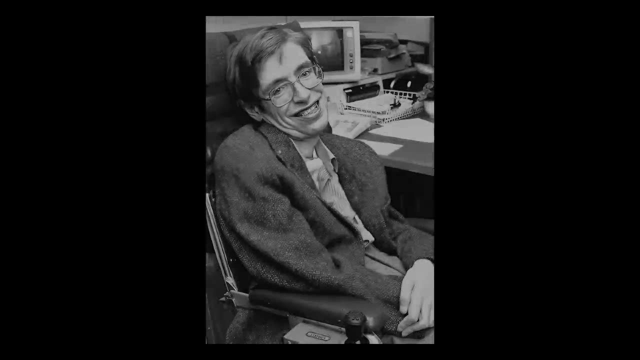 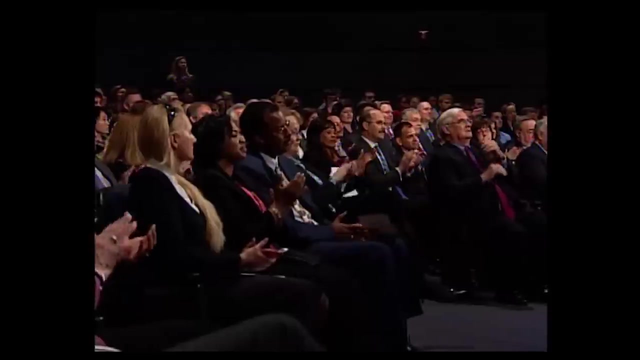 could no longer be able to coordinate his movements, talk and, eventually, swallow and breathe. The doctors predicted that 21-year-old Hawking had two years left to live, But Stephen Hawking defied his doctors Instead of fading away over the next two years. 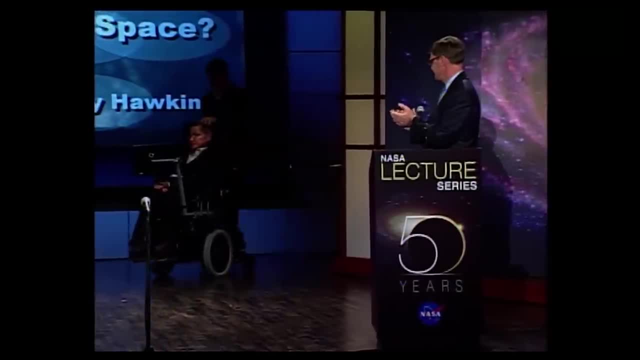 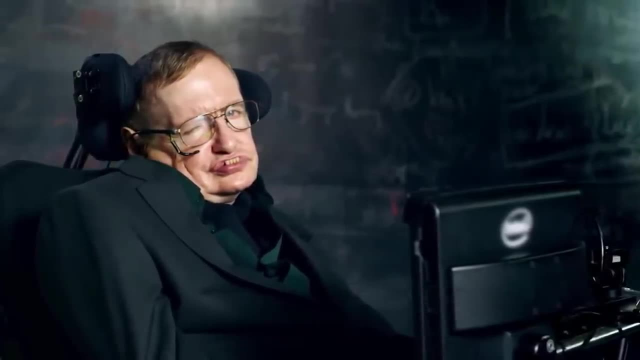 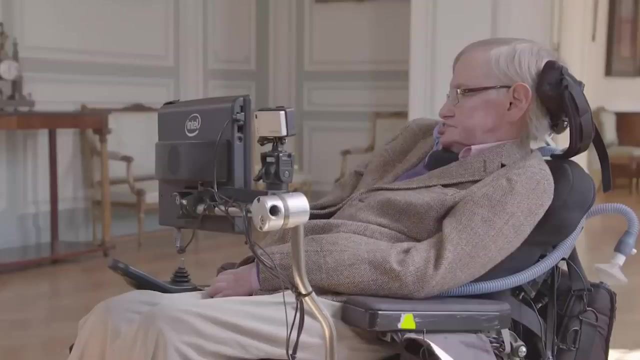 he took his vitamins and kept fighting for 55 years more. In refusing to surrender to his ALS, Hawking completes his postgraduate studies, becomes an esteemed academic and eventually a household name, Arguably one of the most famous scientists of all time, rivaling the great Charles Darwin and Albert Einstein. 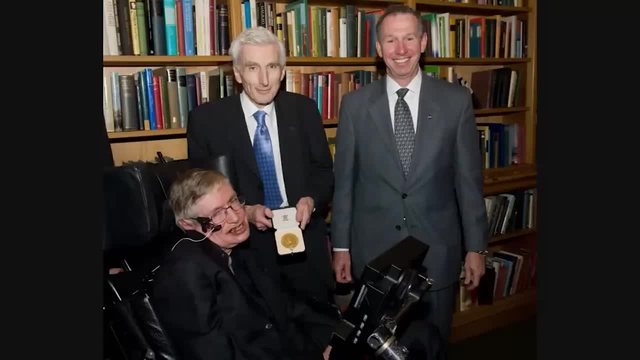 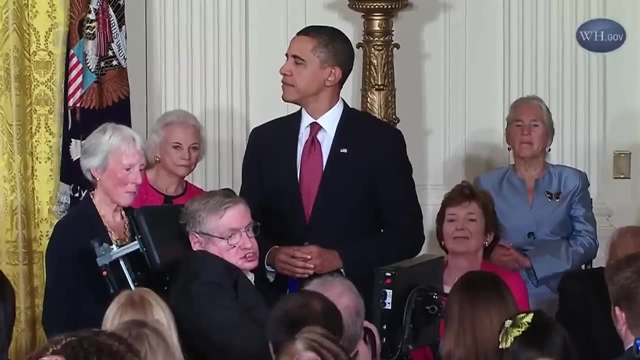 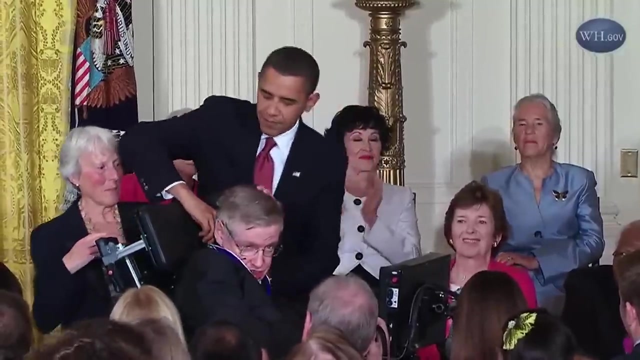 and becoming one of the youngest ever scholars to be elected a Fellow of the Royal Society, And yet to the public, many of whom failed to grasp the nuances of his physics, he became defined by his ALS and his tenacity in overcoming it for so long. But his science was. 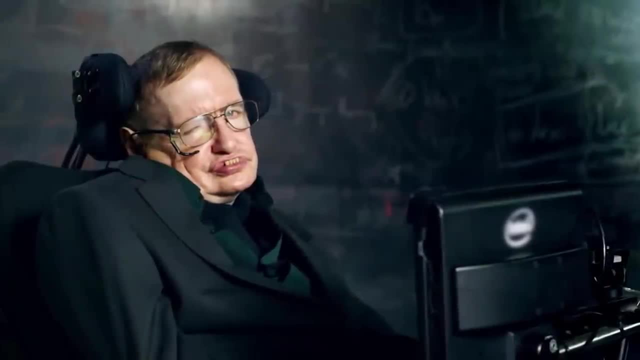 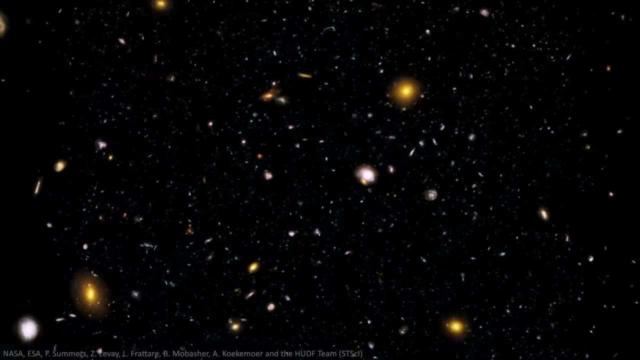 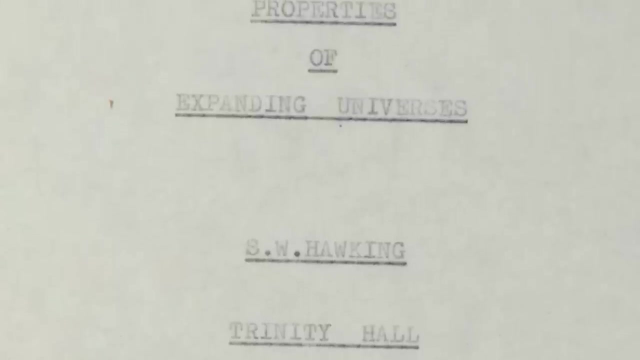 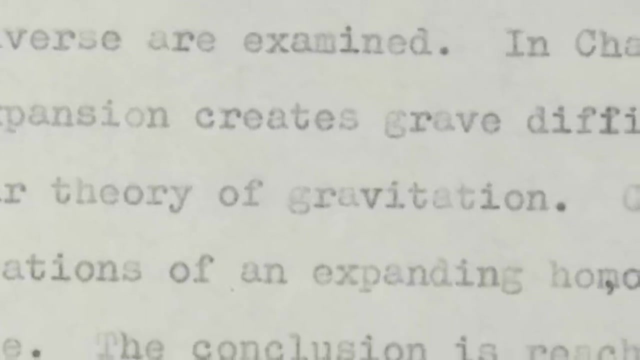 truly worth the accolades and fame he received, For during his long and fruitful academic career, Hawking transformed our understanding of the universe's beginnings and black holes. His doctoral thesis, completed in 1966 under the shadow of his recent diagnosis, focused on the debate that raged at the time concerning the beginnings of the universe. 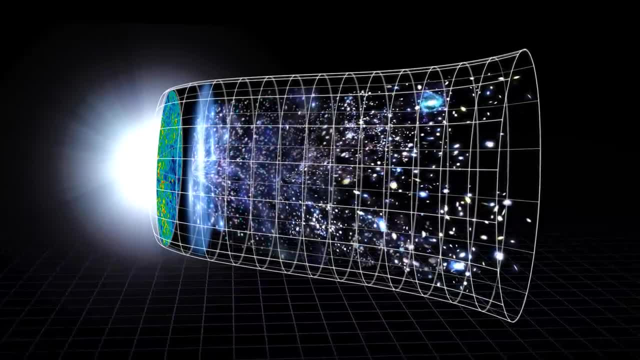 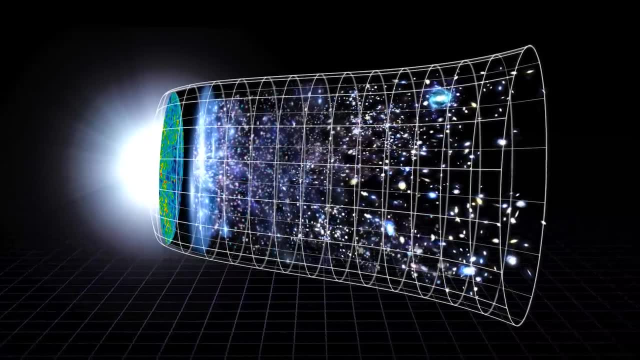 Inspired by the novel physics of an impossibly dense point at the centre of black holes, Hawking made a similar suggestion for the beginning of the universe itself. Throughout the early 1970s, he described and defined the fundamental rules for black holes. 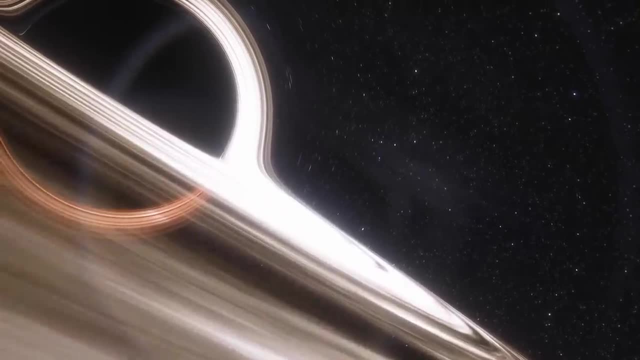 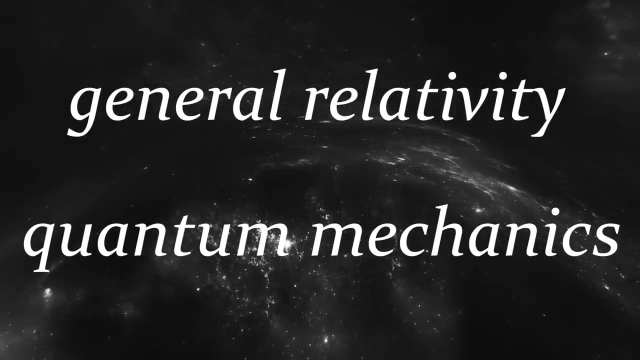 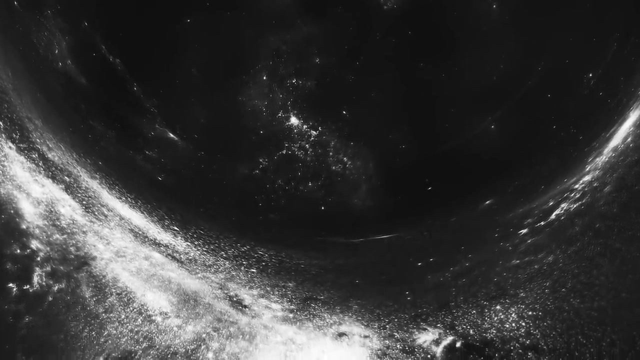 including the observation that an event horizon could never get smaller. Later, however, he attempted to unite the fundamentally incompatible theories of general relativity and quantum mechanics to postulate the existence of a kind of radiation that could actually see black holes evaporate and eventually disappear. This Hawking 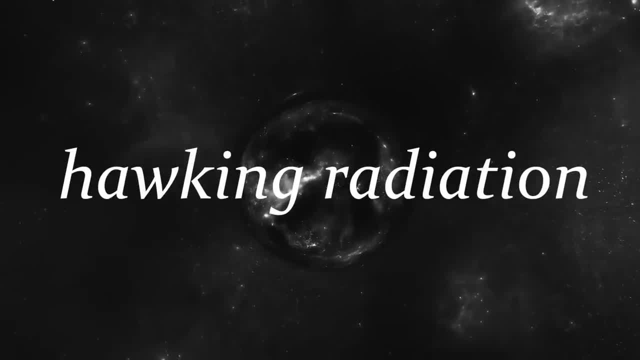 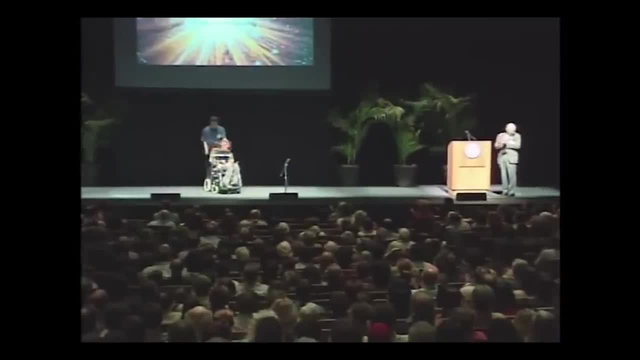 as it became known, was a phenomenon that held up in theory but had not been seen in practice in any discovered black hole. Hawking continued to grapple with these problems throughout his entire academic life, But even while he was tackling the unknowable about modern black holes, 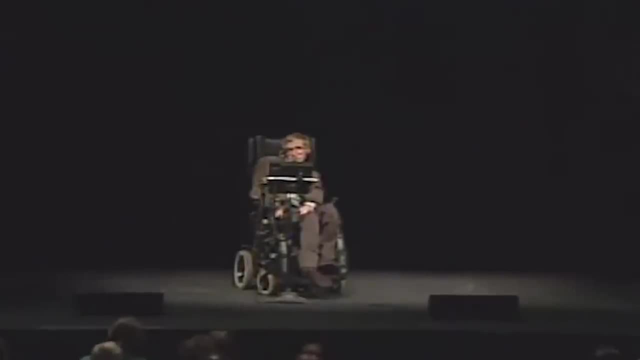 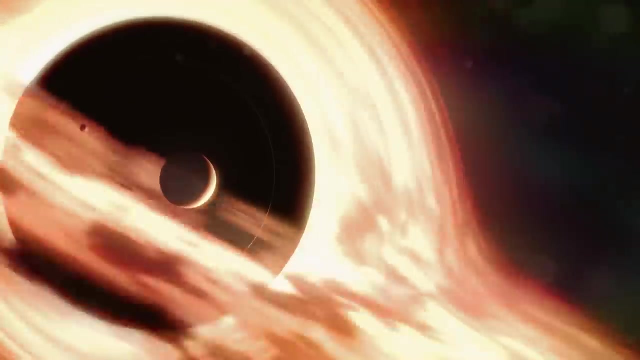 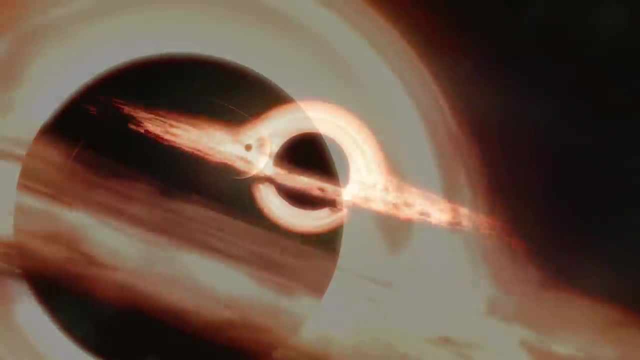 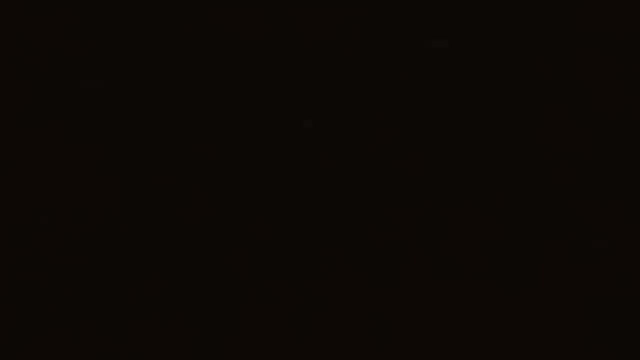 Stephen Hawking's attention was continually drawn back to the cosmos as a whole, and in particular its beginnings. Hawking's study of black holes endlessly informed. his research in the unreachable Big Bang and his unique understanding of the universe's first moments gave him new insights into black holes. And so, in 1971, he popularised a radical 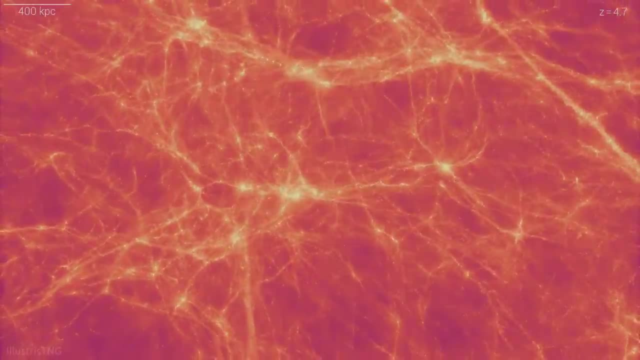 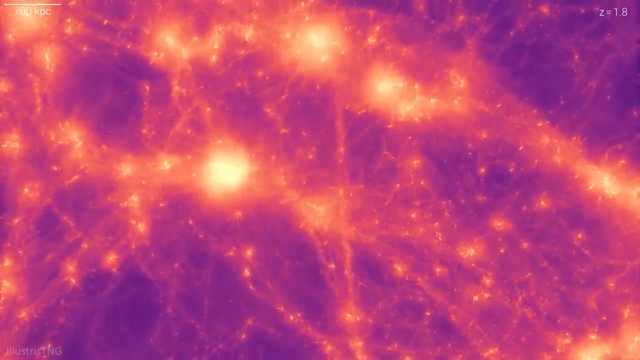 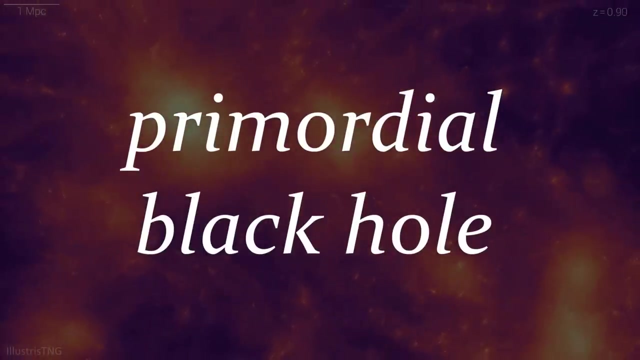 suggestion for which, at the time, there was little tangible evidence. He proposed that a new type of black hole could be found at the beginning of the universe, A so-called primordial black hole, Which formed not from dying stars but from the birth of the cosmos itself. 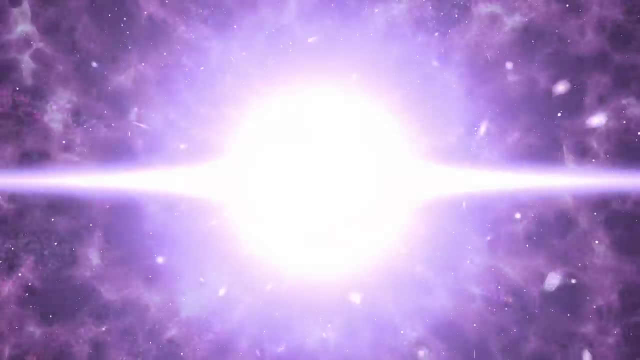 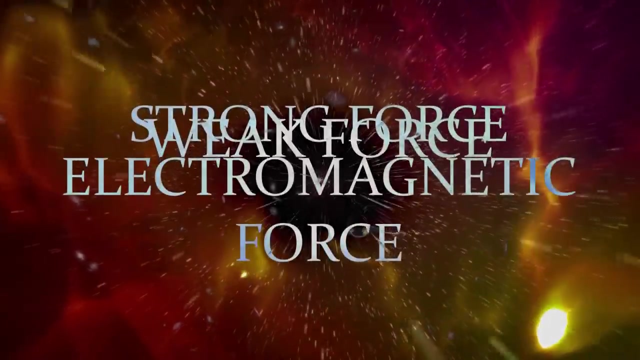 13.8 billion years ago, the Big Bang results in the creation of energy fields that permeate the cosmos and which, as the universe cools and expands, disentangle into the fields of force that rule our lives today. Further cooling sees the very first subatomic particles, quarks and 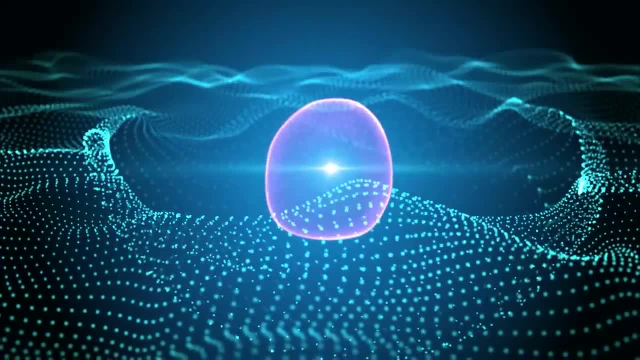 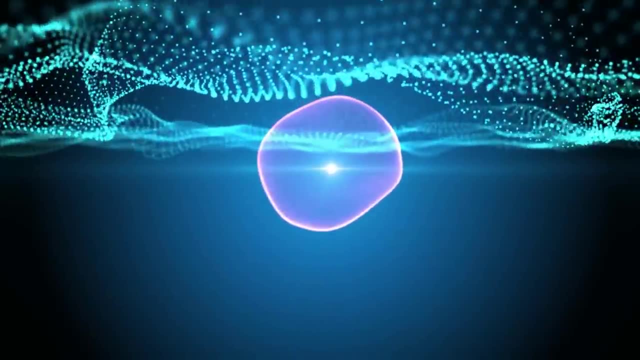 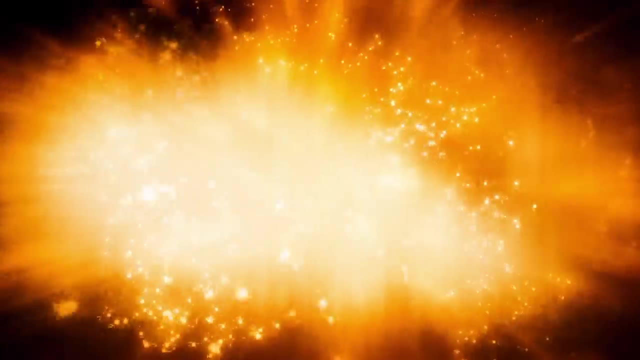 leptons spring into existence and be endowed with properties like mass and charge, which will again come to rule the physics of the next 13.8 billion years. But the universe is still far too small, hot and turbulent for any real matter as we know it today to exist. Suddenly, inflation. 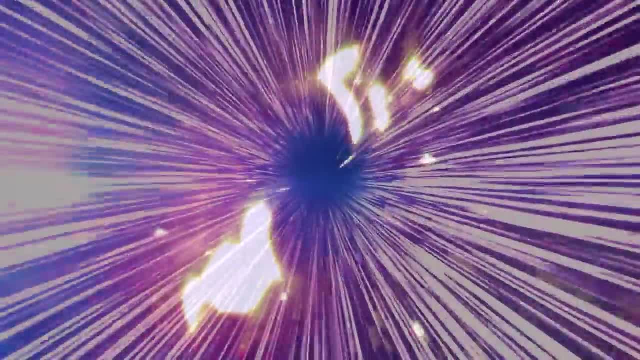 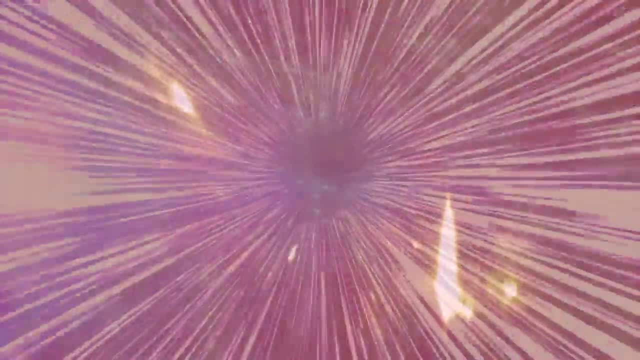 triggered by as yet unknown forces, sees the universe double in size around 90 times in 10 million billion, billion billionths of a second. The universe is now a whole. The universe is now a second. Tiny variations in quantum energy throughout the minuscule pre-inflationary. 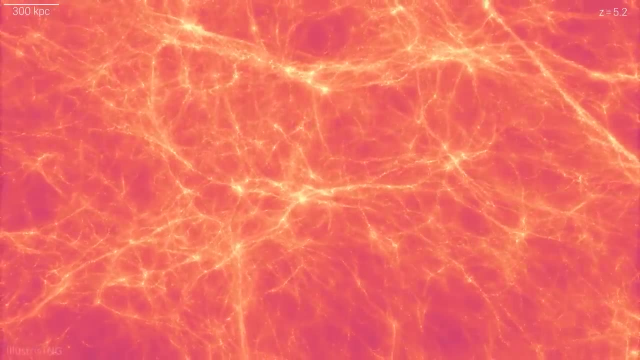 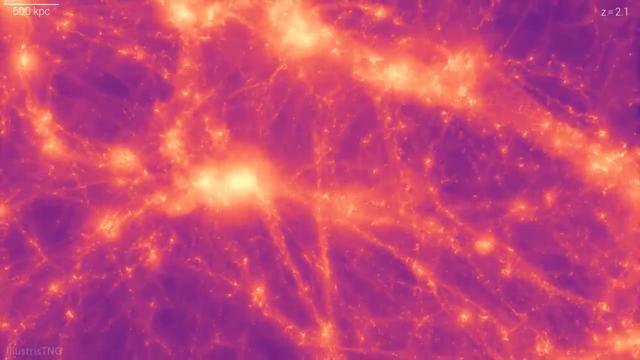 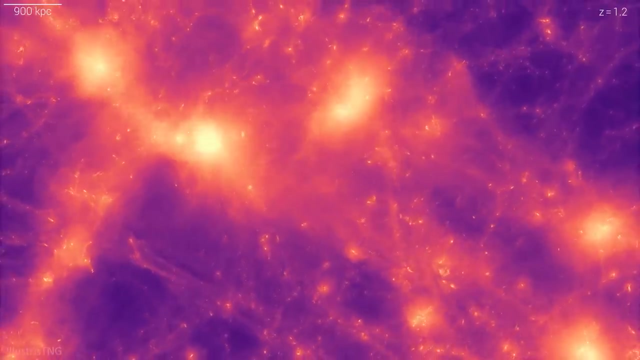 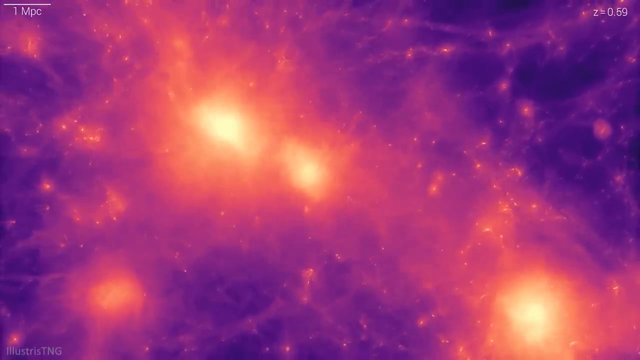 universe are now almost instantaneously transformed into vast regions of inhomogeneity. All over this inflated universe there are variations in the density of particles and energy that will provide the seeds for the overall structure of the cosmos many billions of years later. But Stephen Hawking also foresaw another consequence of these density variations: over newly. 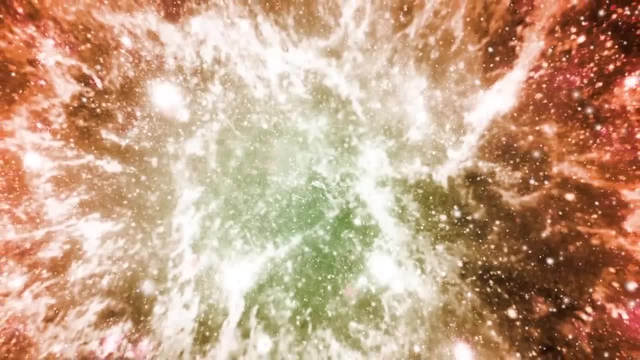 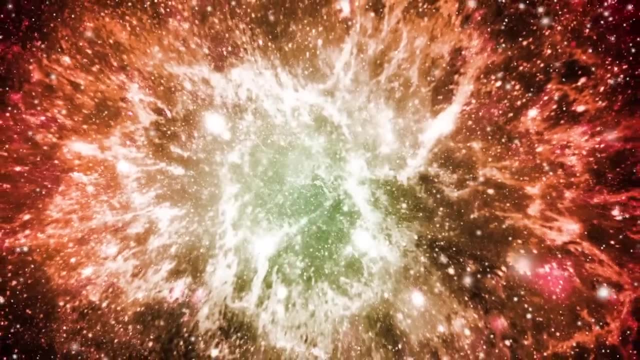 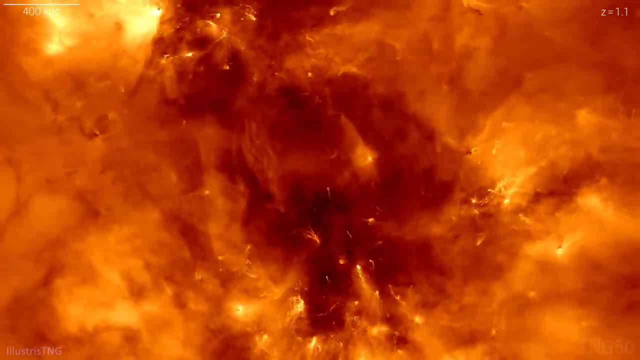 expanded space. Where there is stuff, there is gravity, and these denser regions begin to curve the fabric of spacetime on a macroscopic scale for the very first time. According to Hawking, the response to this sudden and spontaneous shift was for the denser patches to begin to tumble into. 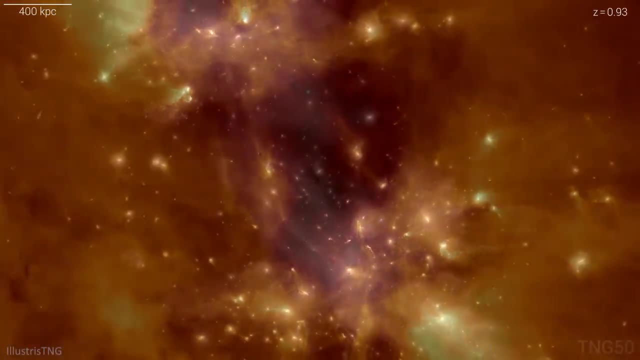 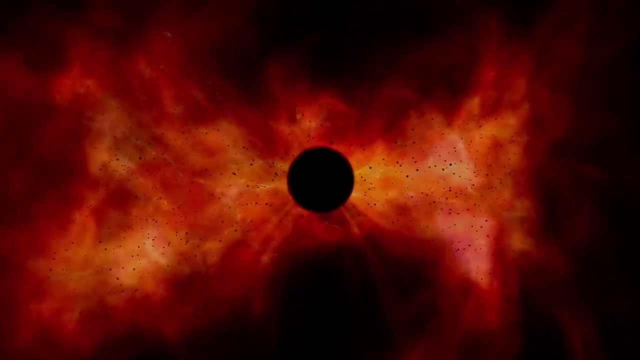 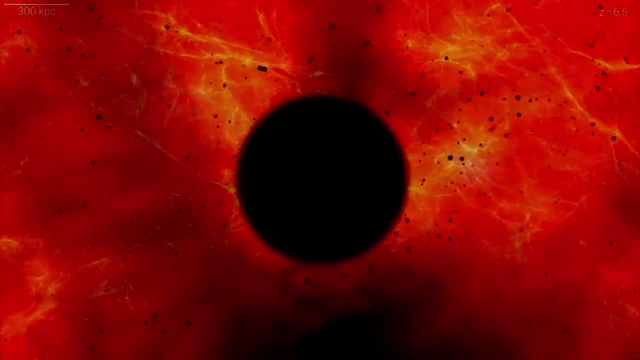 their own gravitational wells collapsing in on themselves due to gravity and, in doing so, exponentially increasing their own gravitational potential. SPACE TIME. As this runaway gravitational collapse continues, the fundamental stuff of the universe is compressed into the mathematically infinitely dense singularity which captures all. 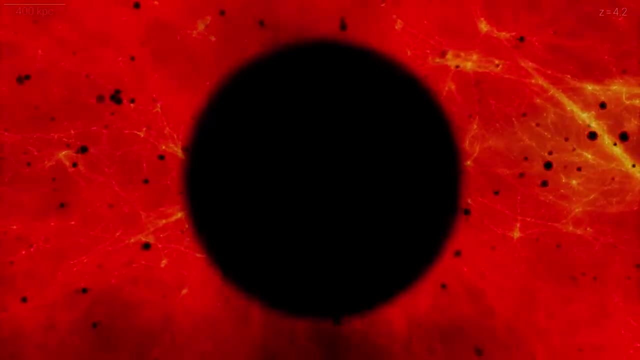 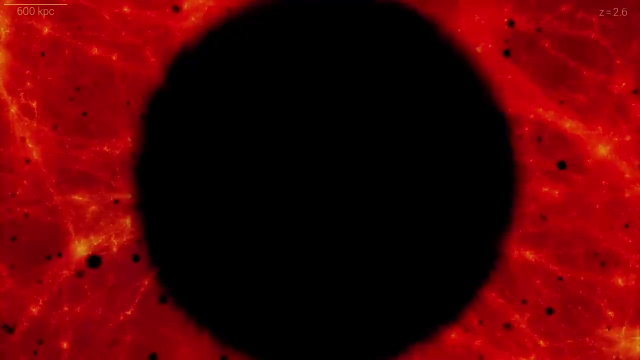 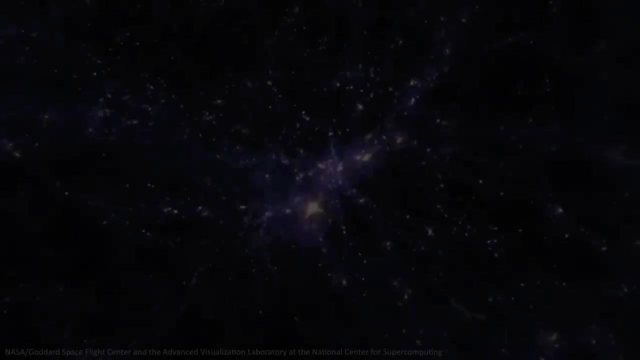 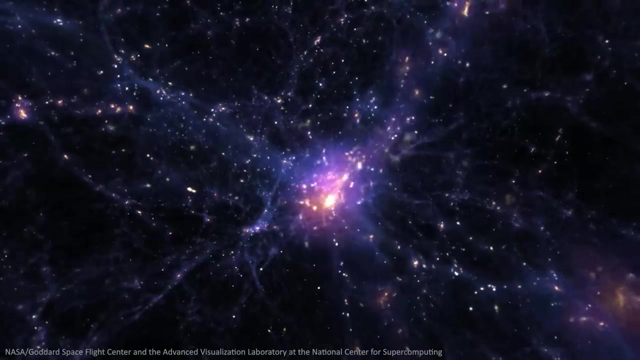 The singularity is cloaked in an event horizon and the newborn particles are locked away for eternity before spending even one full second. in the universe, The Cosmos, All over the freshly expanded cosmos, primordial black holes appear at the hearts of the densest patches of nascent matter. Mathematically, there is only a very brief window. 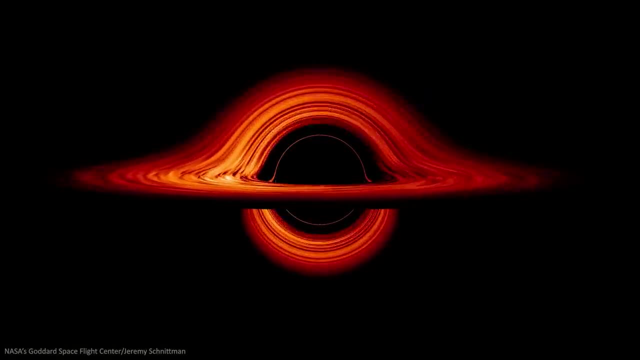 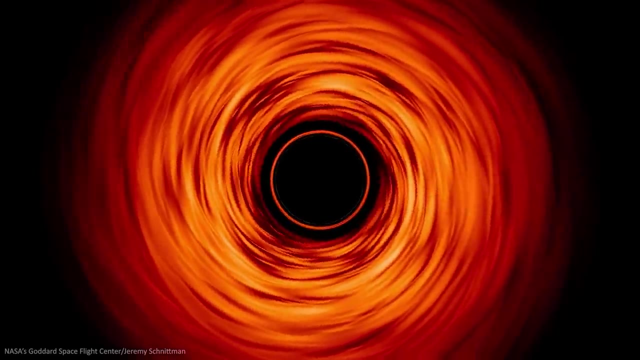 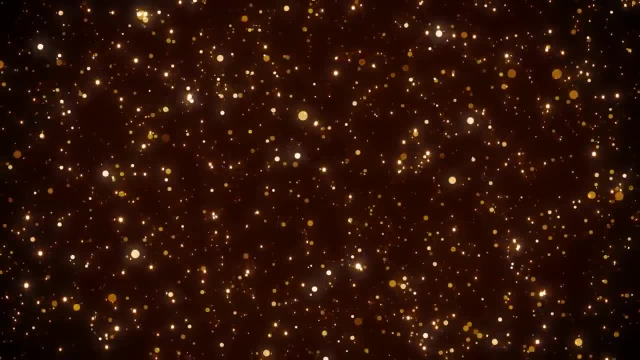 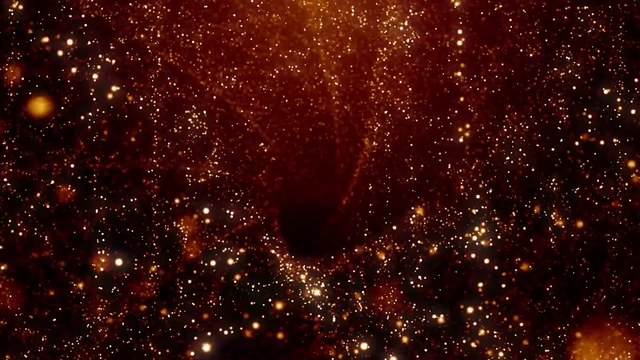 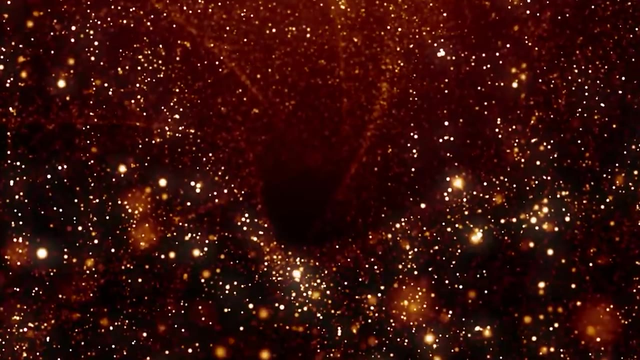 But prior to this point there is no physical reason why primordial black holes couldn't have filled the embryonic cosmos. Hawking and others calculated that the later in this one-second window that this gravitational collapse occurred, the larger the primordial black hole would actually be. 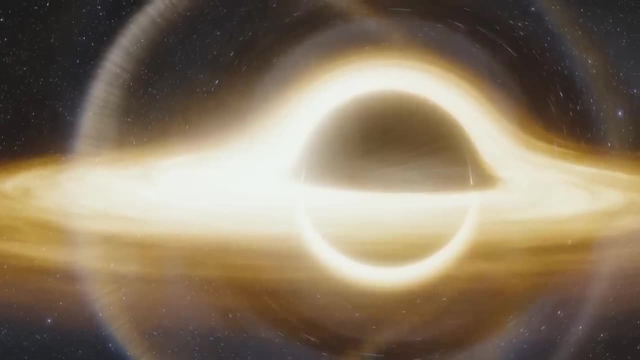 This means that they could range in size from anywhere from 1 100,000th the mass of a paperclip up to Lewis, rasped to 100,000 seconds. 7 degrees up faster than the earth alone. across the davoness is a signal going to exit the universe in day traffic Up to 100,000 seconds. 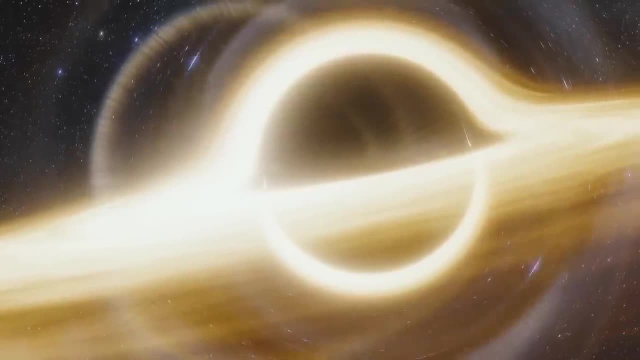 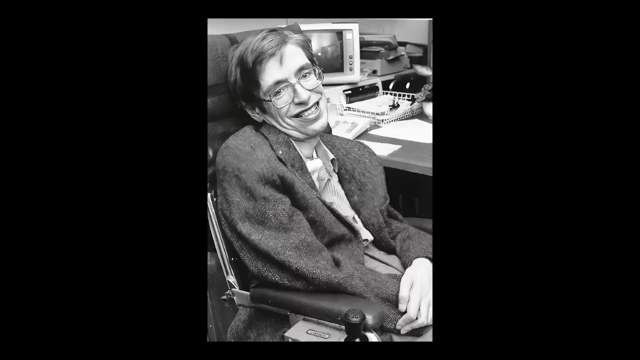 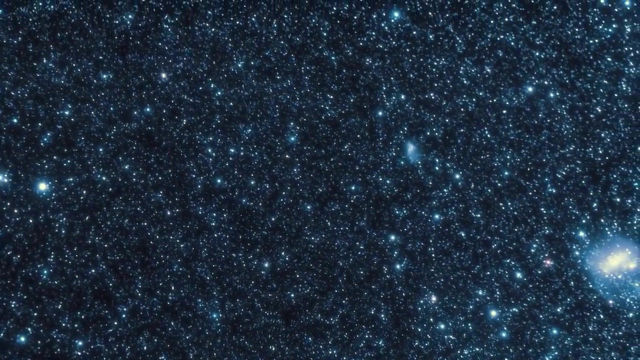 thousand times the mass of the Sun. But here lies the problem. Like so much of Stephen Hawking's work, his elegant mathematics are watertight, but it leaves us with little in the way of testable hypotheses. How do you go about proving that primordial black holes did or didn't exist? 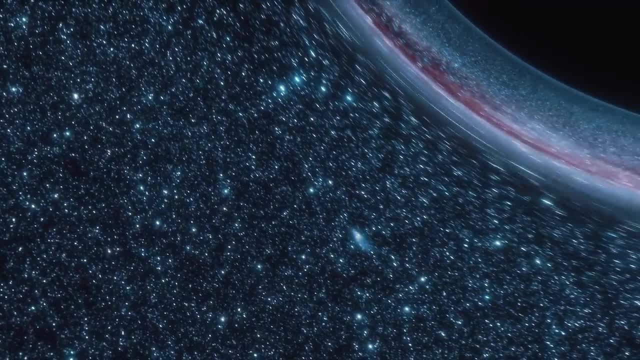 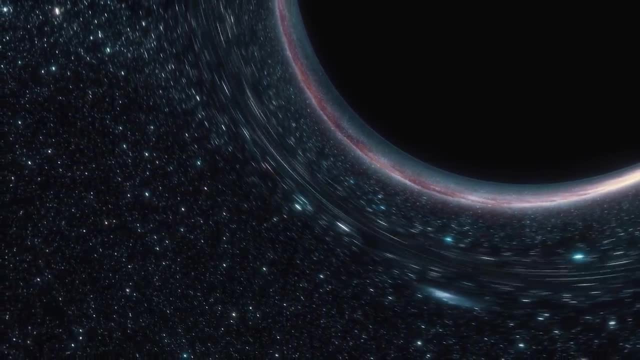 We must find a way to detect them, or at least detect their tangible effects on the early evolution of the universe. But when we don't know how numerous they were exactly when they formed and exactly what size they're likely to be, then searching for the earliest black holes is tantamount. 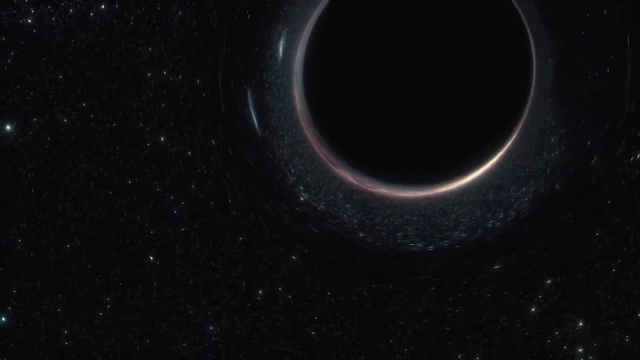 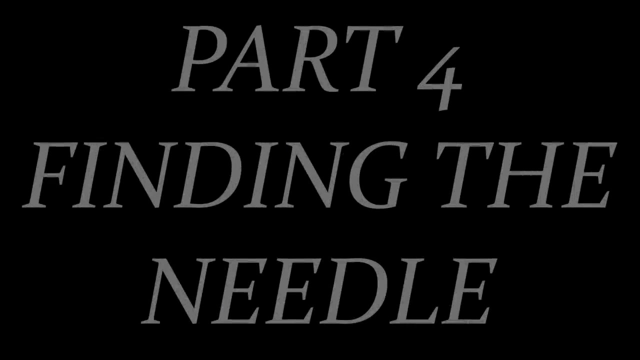 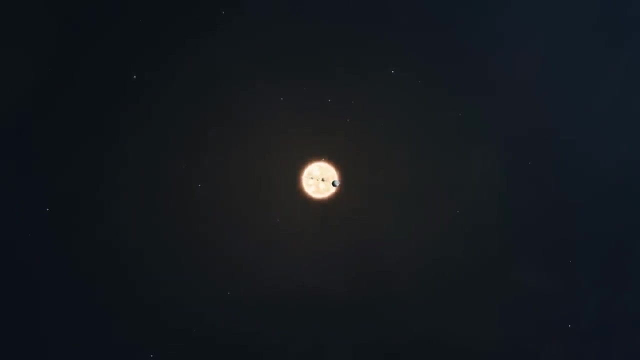 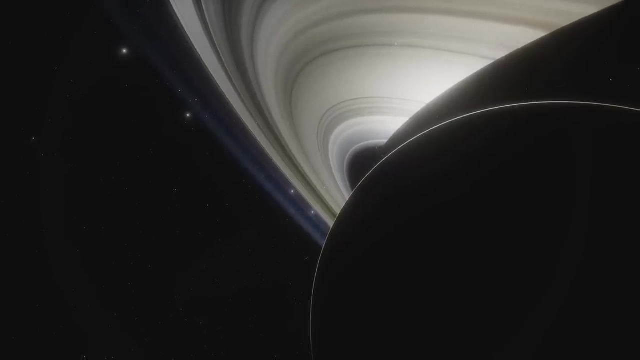 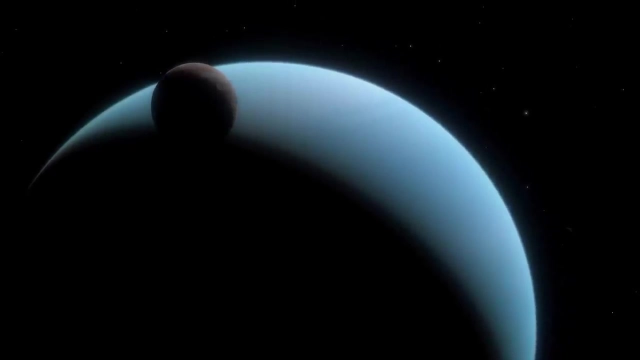 to finding a needle in the cosmological haystack. Mercury, Venus, Earth, Mars, Jupiter, Saturn, Uranus, Neptune- The eight major planets of our solar system. Some have been observed since the second millennium BC, seen and studied with the naked eye. Others have been spotted by telescope or predicted based on their effects on other objects and 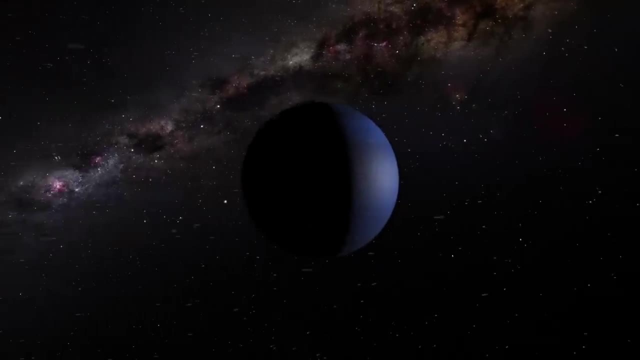 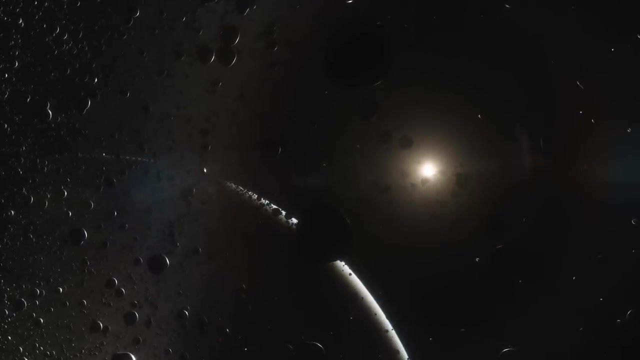 subsequently discovered right where we expected them to be. But there may yet be one more object left to find, Even after 4,000 years of astronomical research. But there may yet be one more object left to find Even after 4,000 years of astronomical research. 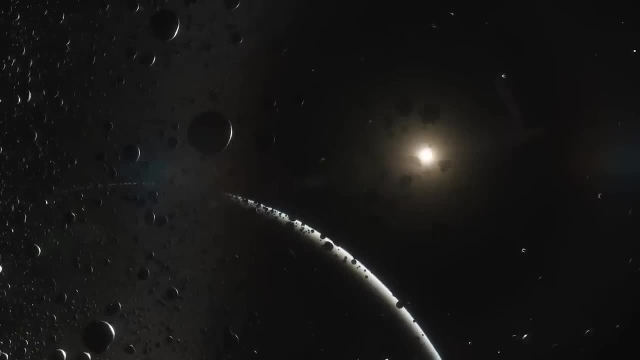 But there are much to discover on our celestial doorstep. But there are much to discover on our celestial doorstep. But there are much to discover on our celestial doorstep. In 1951, Gerard Kuiper, an astronomer and professor at the University of Chicago, contemplated: 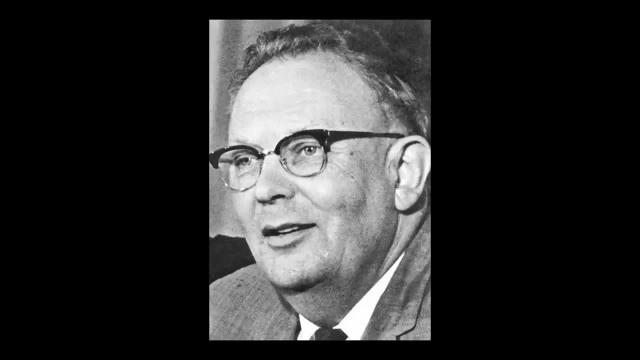 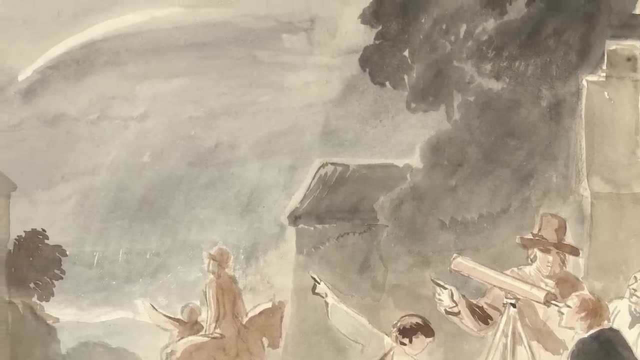 And in 1951, Gerard Kuiper, an astronomer and professor at the University of Chicago, contemplated a cometary conundrum. Scientists had long observed so-called short-period comets, Icy bodies which swing through the solar system on elongated orbits passing close to Earth. 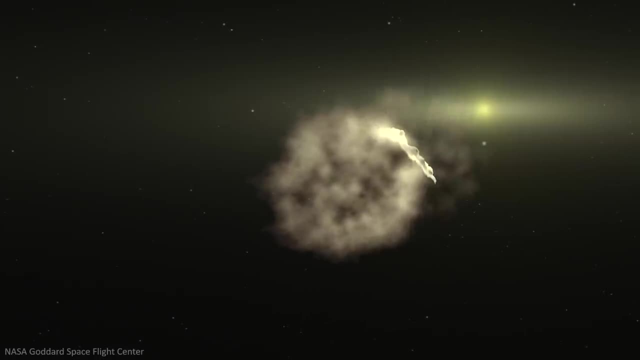 and the Sun every 200 years or less. Halley's Comet, which was last visible to the naked eye in 1986, was probably the last They악 comet of the 2008 exploration. Ms Mcomenne, The late engineers at Lewis and others had 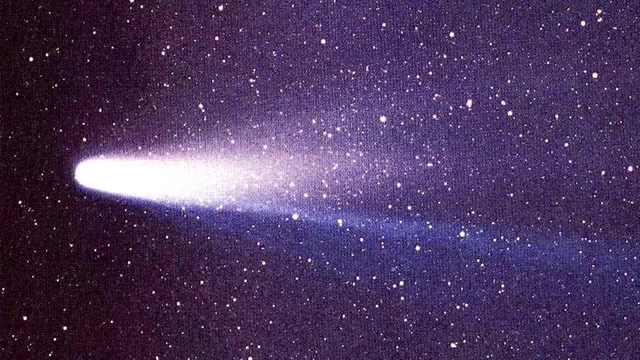 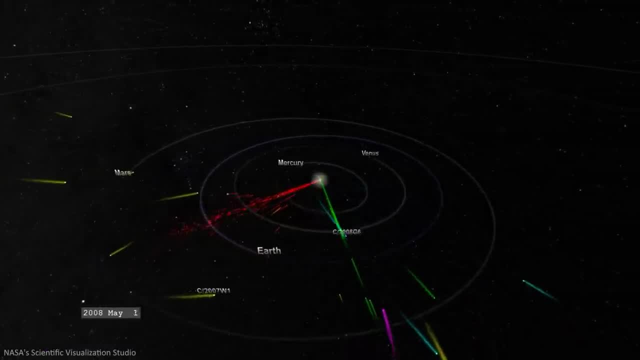 discovered this comet that would allow기에 helium 1986, and will revisit us again in 2061,, is one such visitor, But its flybys won't last forever. Every time the comet passes close to the Sun, it evaporates more of its icy core and after 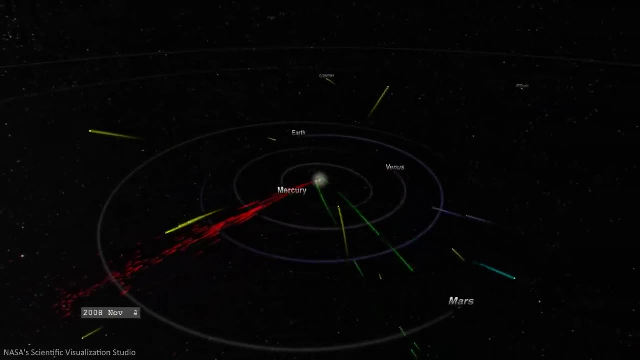 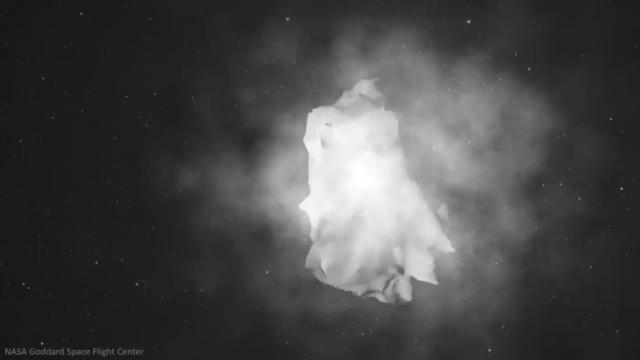 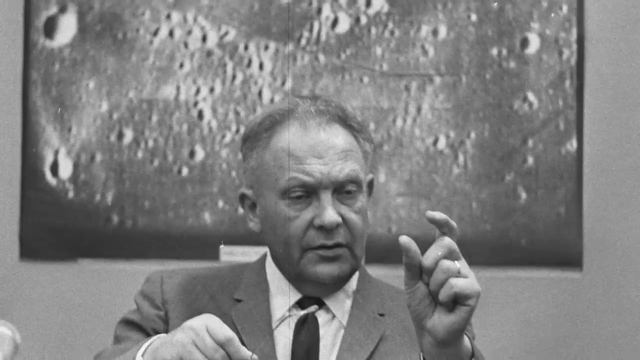 a few more orbits it will be lost completely to nebulous interplanetary space. But by this reasoning, after the four and a half billion years that our solar system has been around, there shouldn't be any more short period comets left, Unless Kuiper reasoned there was a nursery of icy bodies far out in the outer solar system. 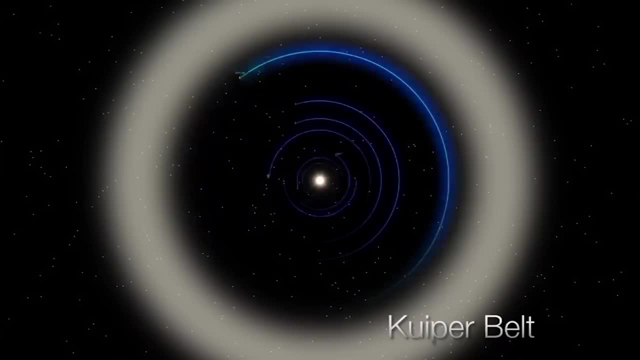 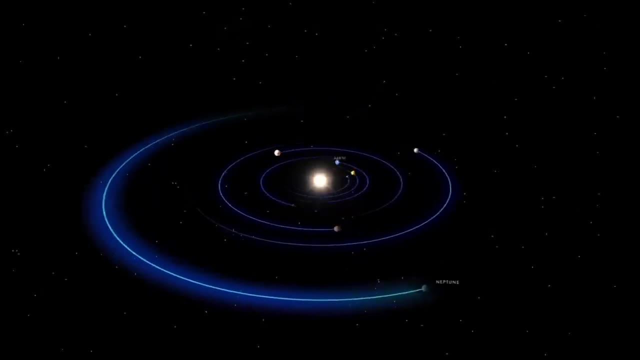 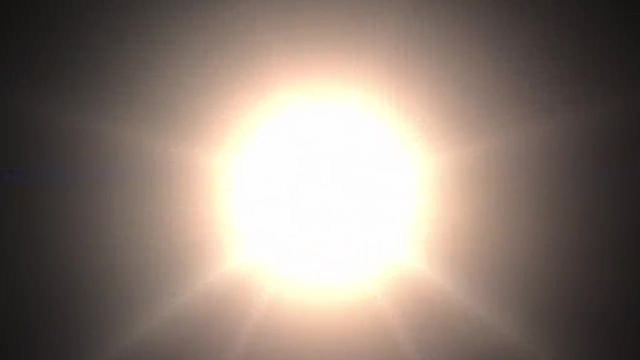 beyond the orbit of Neptune. A belt filled with orbiting chunks of ice could be disturbed by the gravity of Neptune and the other giant planets flinging ice blocks in towards the Sun to become comets on a swinging death spiral that lasts thousands or even millions of years. 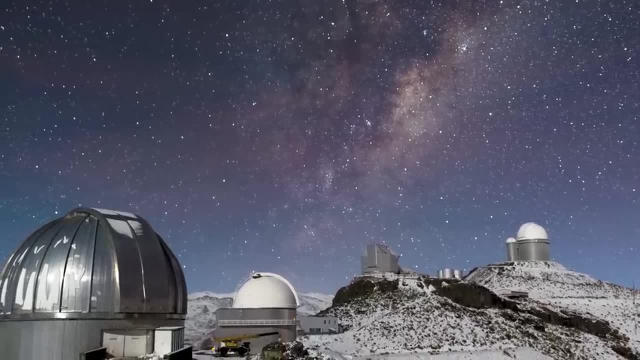 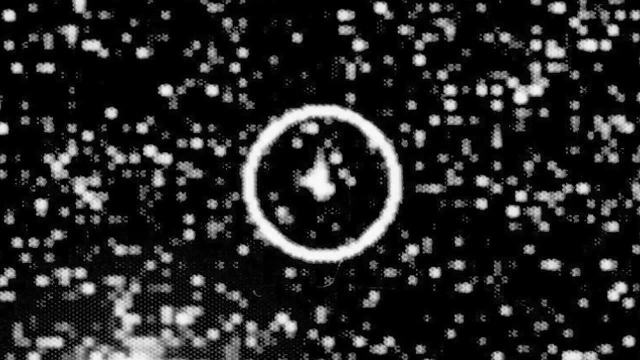 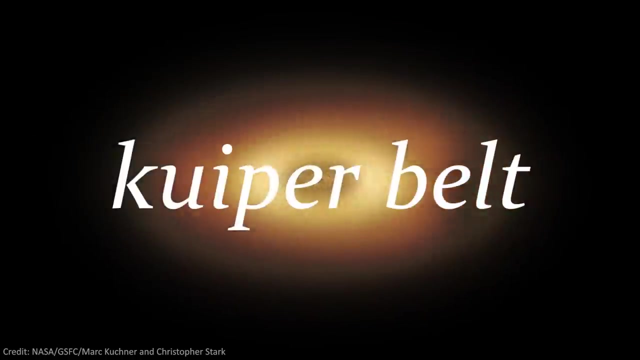 Despite Kuiper's early predictions, it wasn't until 1992 that evidence for this belt of icy objects was found. NASA scientists spotted the first one, and then many more of these so-called trans-Neptunian objects, and the space they occupied became known as the Kuiper Belt. 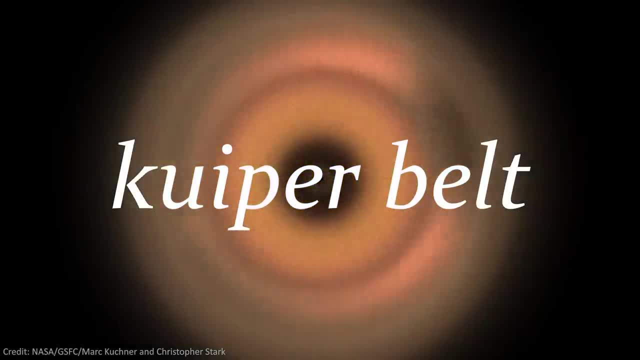 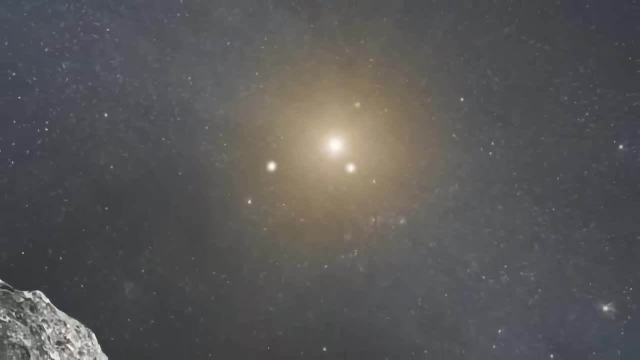 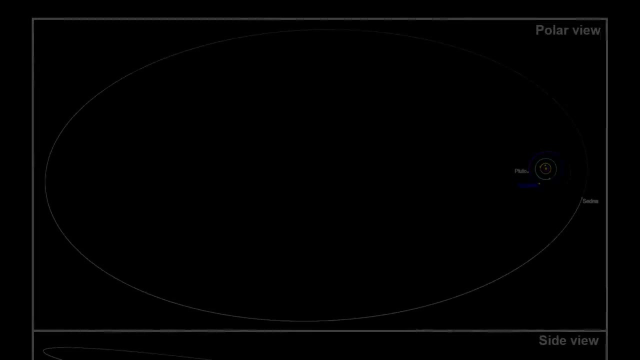 But as the inventory of Kuiper Belt objects grew, another conundrum presented itself. There were some that seemed to behave quite strangely. Saturn, a dwarf planet named Sedna, discovered in 2003,, has a very long, extremely elliptical. 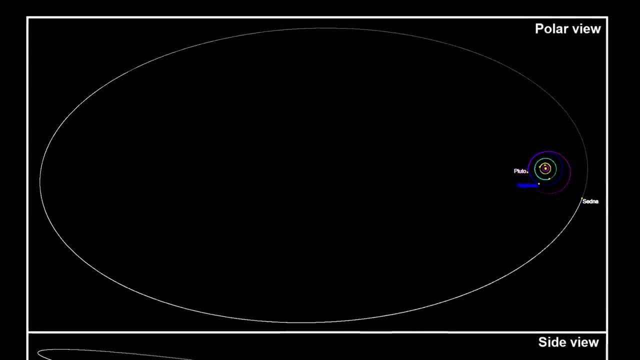 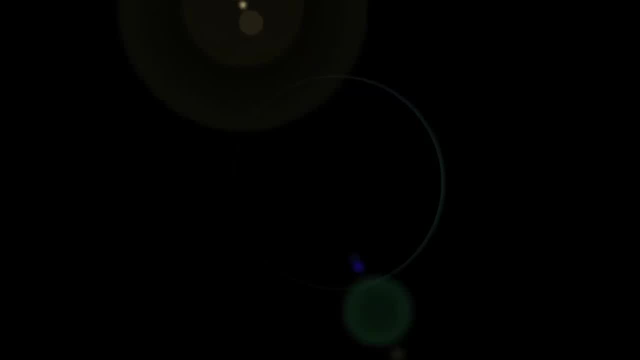 orbit that takes more than 10,000 years to complete. And even at its closest approach, Sedna is still two and a half times further from the Sun than Neptune. There is simply no way that Neptune could be responsible for setting off this huge motion. 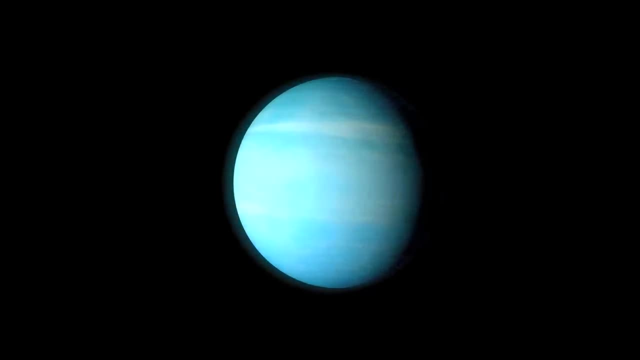 Other extreme trans-Neptunian orbits also show a surprising pattern, clustering to one side of the solar system and tilted deeply below the equatorial plane. Saturn, on the other hand, is a dwarf planet named Sedna, discovered in 2003, and has a 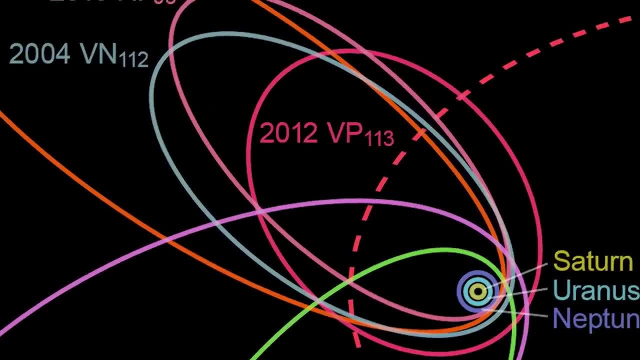 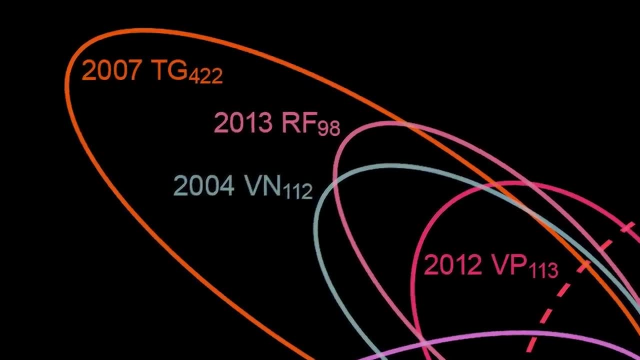 very long, extremely elliptical orbit that takes more than 10,000 years to complete. Statistically, such a distribution is extremely unlikely In the absence of external influences. these objects' orbits should randomize over a hundred million years, And so, in 2012,, a Brazilian astronomer named Rodney Gomes suggested an explanation for. 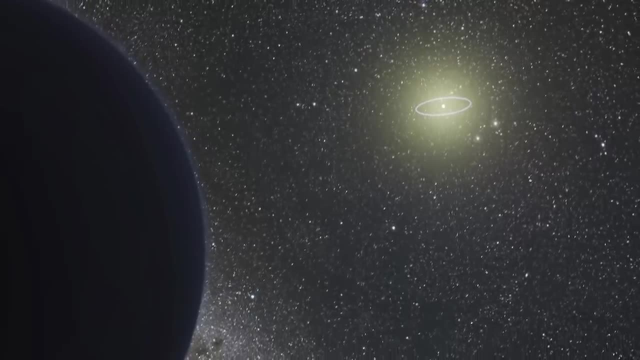 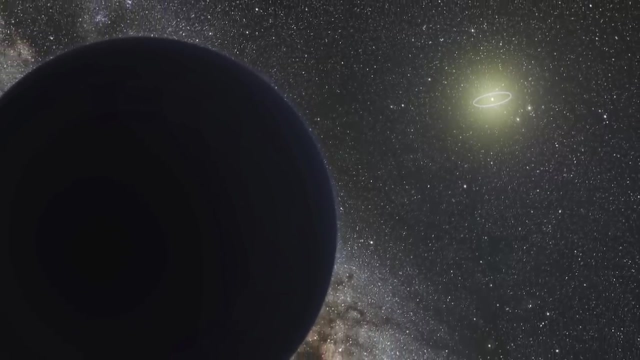 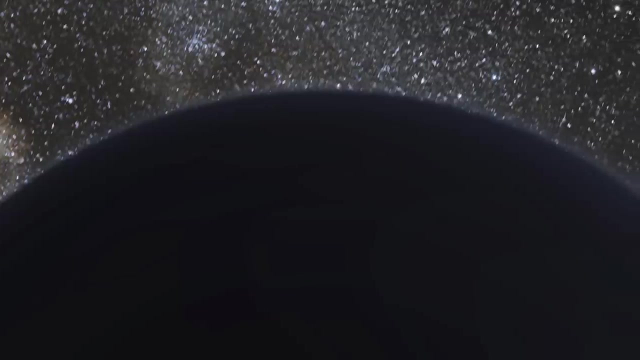 these bizarre orbital patterns, That there was in fact an external influence in the form of a distant, massive planet that shepherds them around. That hypothetical planet has come to life. It's been a long, extremely elliptical orbit. It's come to be known as Planet 9.. 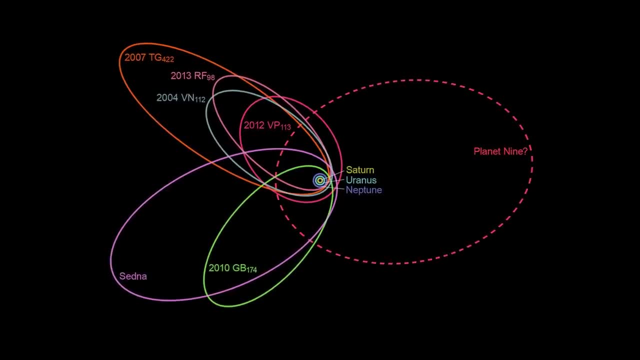 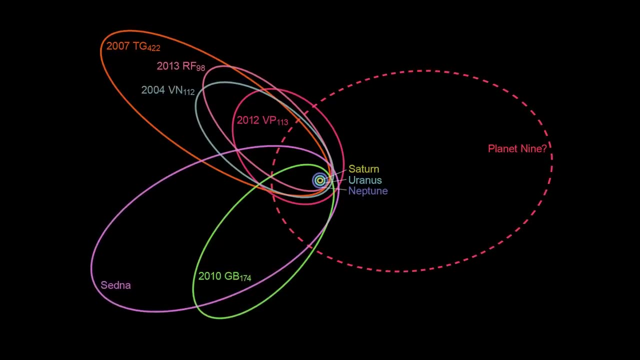 By the orbital calculations, Planet 9 would be around 6 times the mass of the Earth, travelling on an elongated and tilted orbit around 400 times further from the Sun than the Earth's own orbit. But despite knowing this and searching specifically for it with the highest resolution instruments, 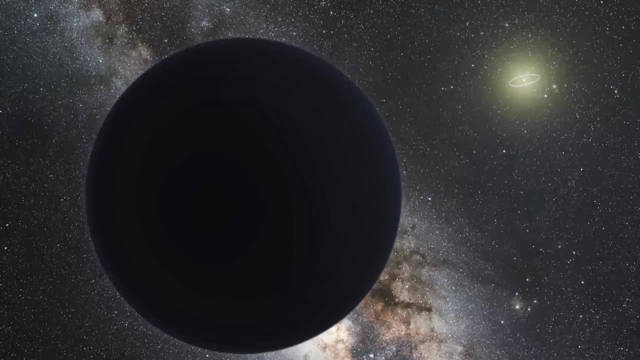 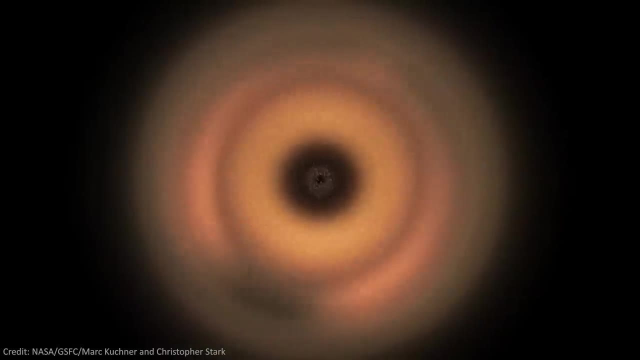 we possess. astronomers haven't found a trace of this Neptune-sized planet. Critics have countered that the anomalous orbits could be the result of observational bias. They are shaped by how and where we can search for Kuiper Belt objects, and that Planet 9. 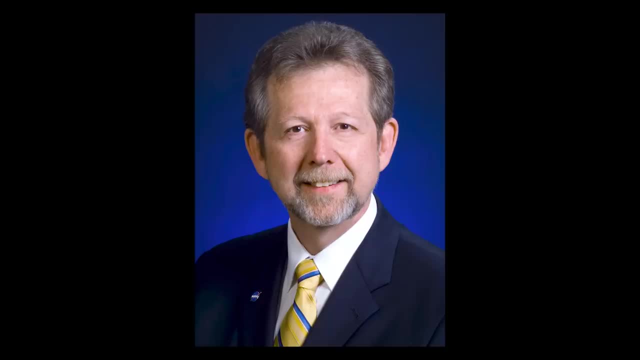 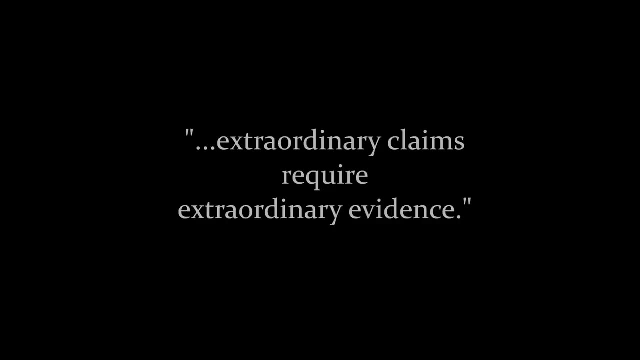 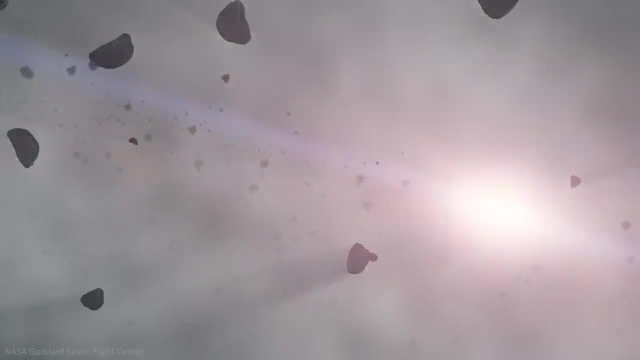 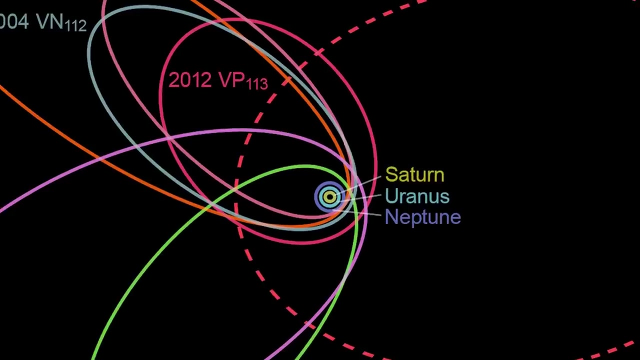 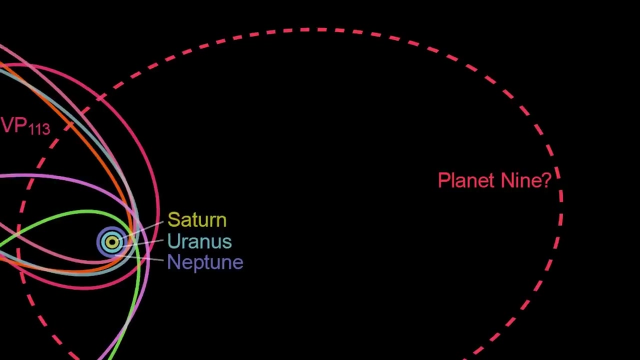 doesn't really exist. Jim Green, NASA's chief scientist at the time, quoted Carl Sagan saying: Extraordinary claims require extraordinary evidence. And there is another tantalising possibility, Another even more extraordinary claim: What if, What if, What if we found something? 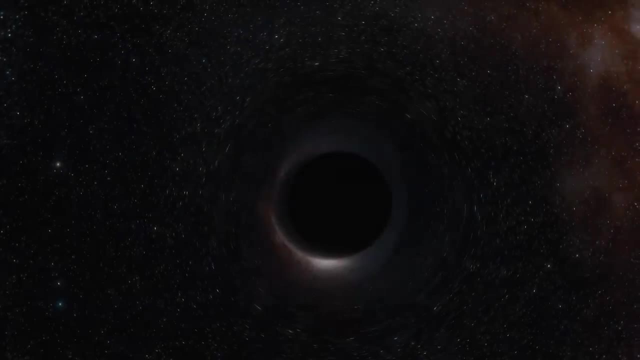 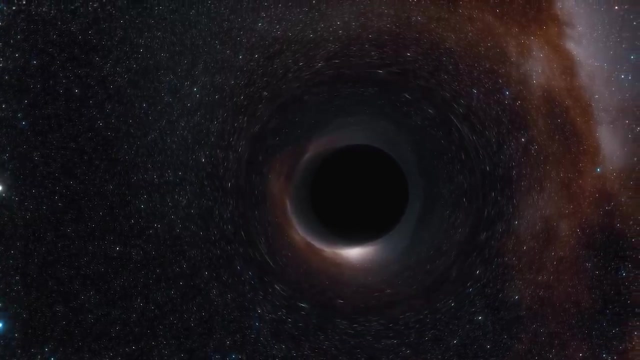 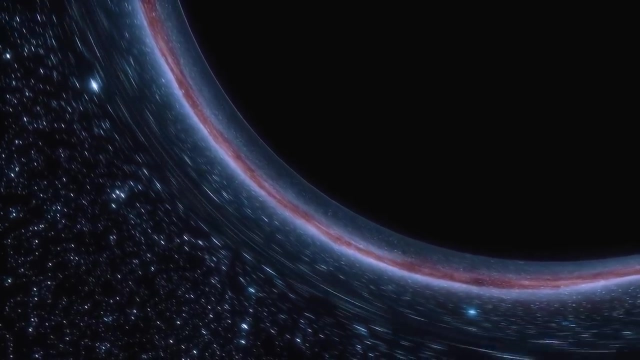 much, very small. Wow, Oh dear. What if? What if? Would we believe this, or would we just be scared? Is this one of the ambiguous stories they're starting to bring to light? Ourbur selber horizon would be approximately the size of a tennis ball. Not only would it be completely black. 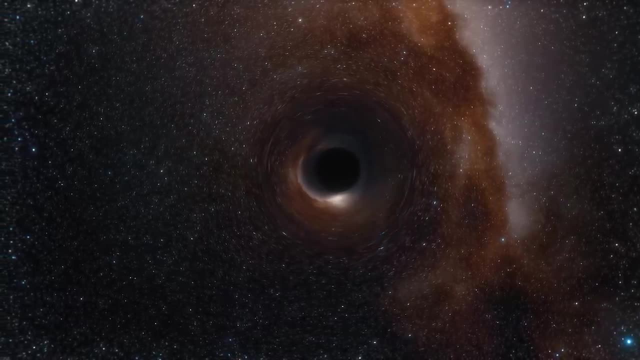 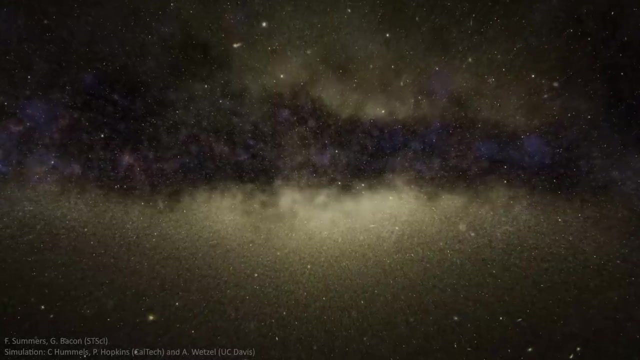 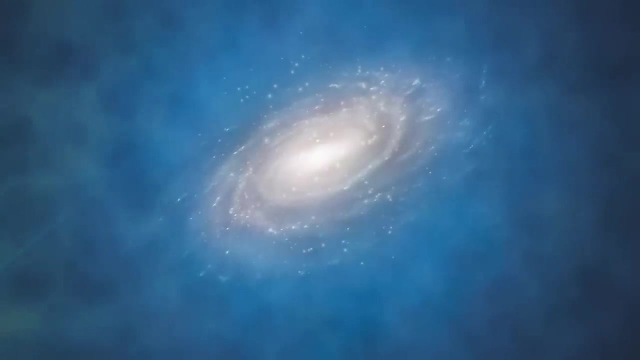 but set against the vastness of space, it would be almost impossibly tiny too. Of course, theorising primordial black holes in our galactic neighbourhood is one thing. Actually detecting these tiny but potent objects is quite another. Some suggest that their intense gravity would be enough to attract a micro-halo. 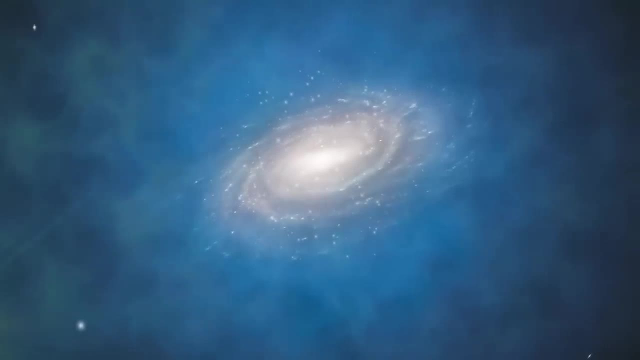 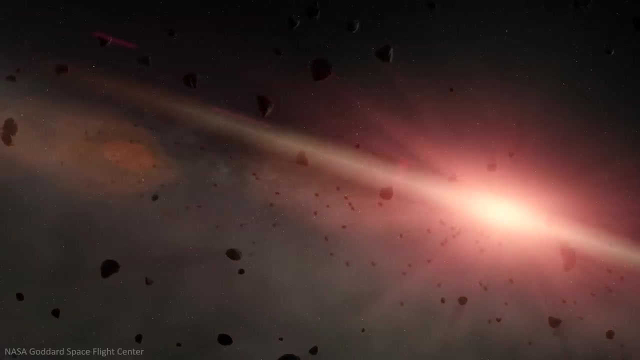 of dark matter. just as entire galaxies are thought to be enveloped in a dark matter halo on a massive scale, So by searching for the dark matter and its associated radiation in the direction of planet 9, we might hope to distinguish planet from black hole and, in doing so, provide 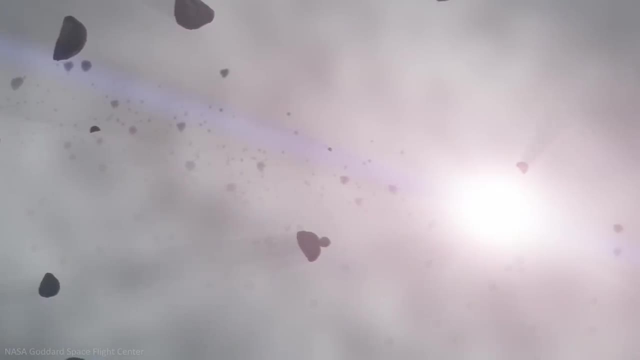 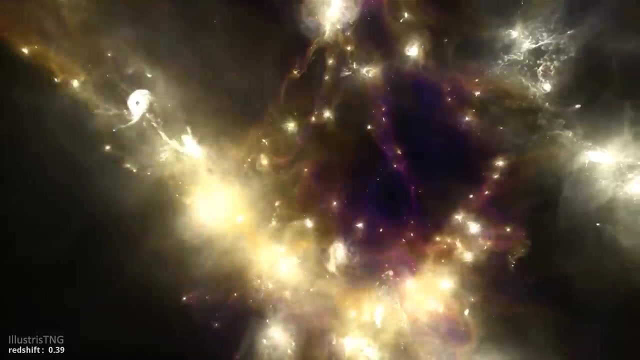 evidence for the early evolution of the universe itself. And yet this methodology depends very much on the theoretical assumptions of what exactly dark matter is and how it behaves, which is by far the most important part of this theory. And yet this methodology depends very much on the theoretical assumptions of what exactly dark matter is and how it behaves, which is by far the most important part of this theory. 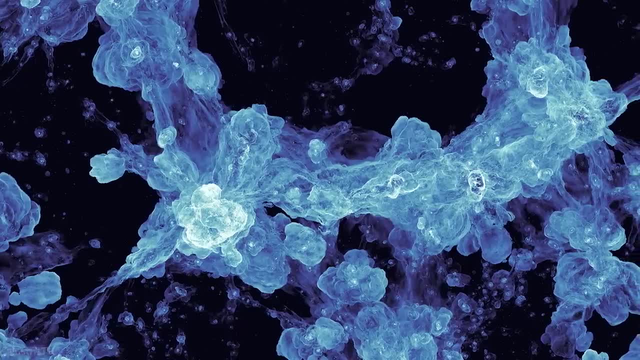 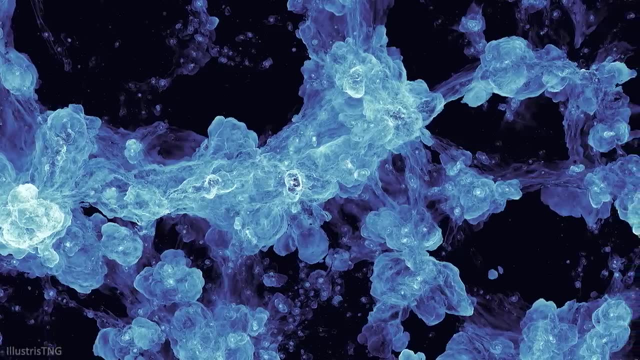 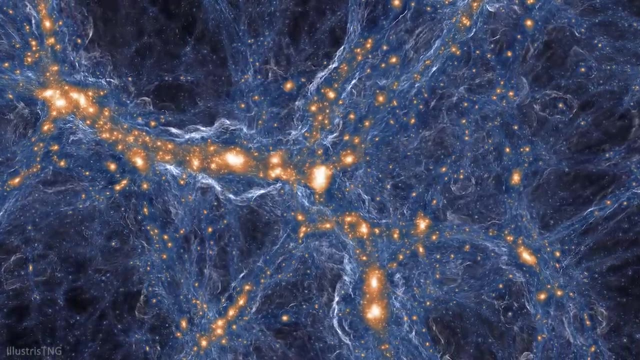 Dark matter is so named because, although it makes up some 27% of the universe as a whole and outweighs normal matter by some 6 to 1, we have never been able to detect it directly. It is dark, invisible to every instrument we have yet invented. 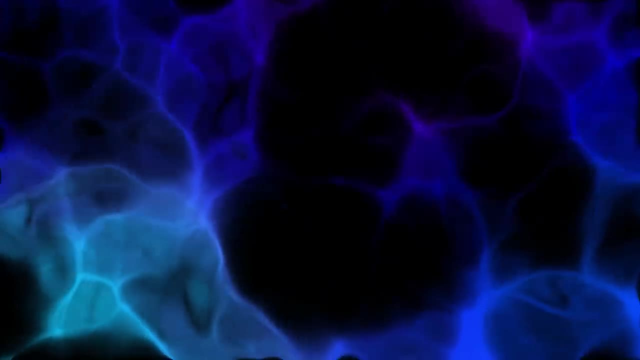 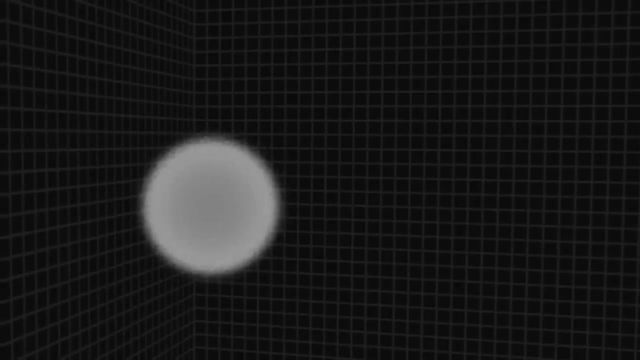 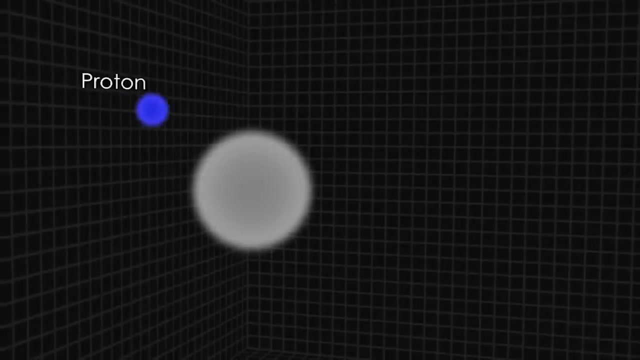 Two camps suggest two different options for the identity of dark matter: Wimps and matches. Wimps, or weakly interacting massive particles, are a subatomic particle that interacts with the universe via gravity but does not otherwise fit into the standard model of particle physics. 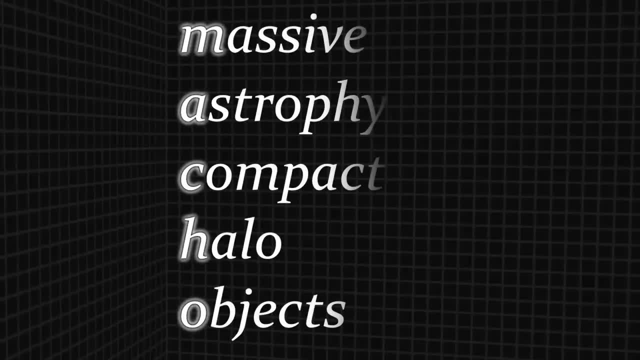 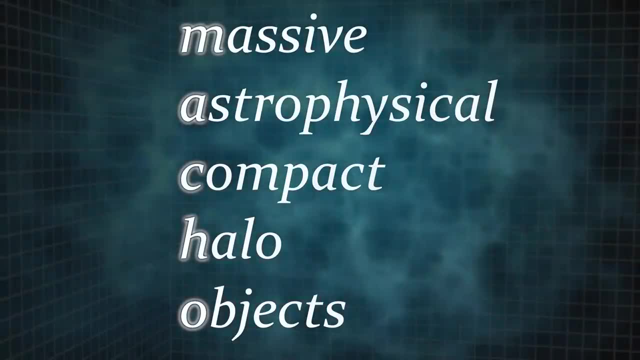 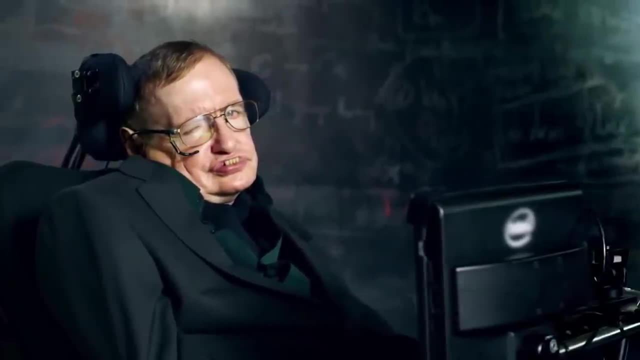 On the other hand, Matchos are massive astrophysical compact halo objects and are theorised as heavy astronomical bodies that could explain the gravitational effects in dark matter halos. Stephen Hawking himself was among the first to suggest that the primordial black holes he predicted could be dark matter halos. He also suggested that the black holes in 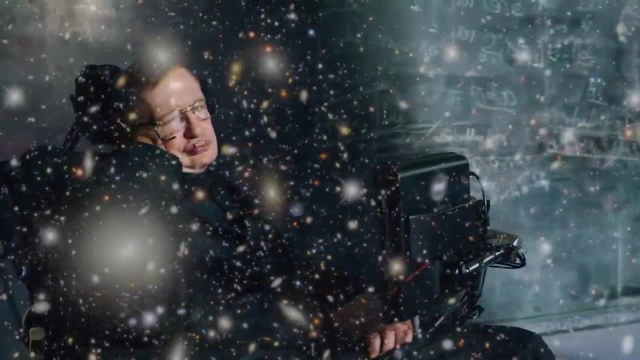 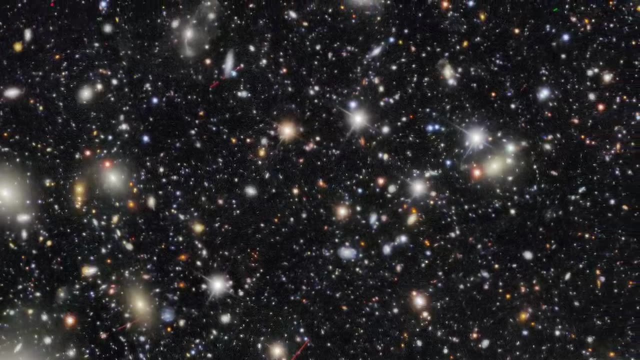 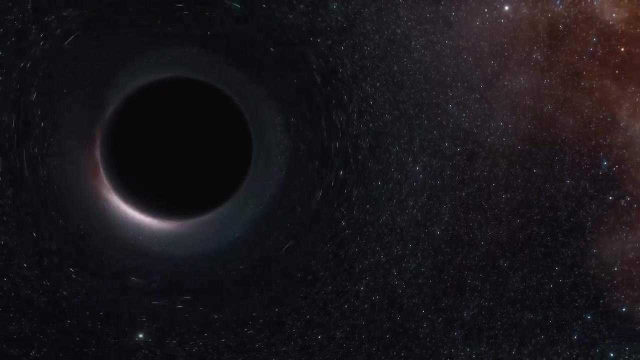 the universe could be a type of macho, thereby making up some, if not all, of the missing matter. If so, the dark matter that holds the universe together is not only dark because it is unknown, but because it is dark by its very essence. Primordial black holes become tiny pinpricks. 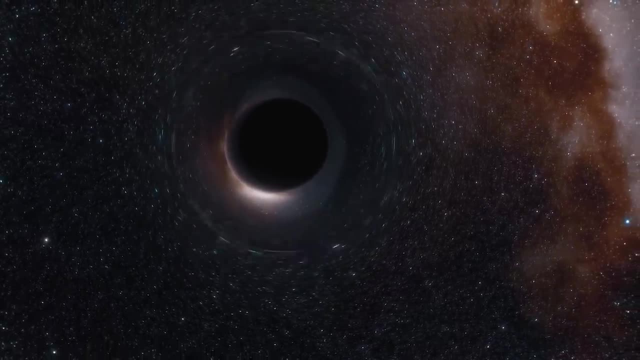 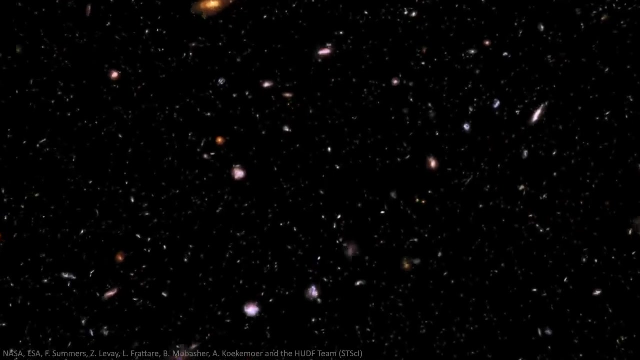 in the fabric of spacetime which, when clustered around galaxies, help to keep swarms of billions of stars in check. The combined mass of primordial black holes formed in the first second of the universe is the mass of the universe. The mass of the universe is the mass of the universe. The 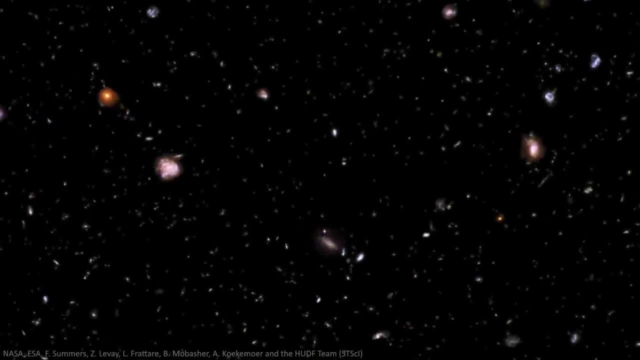 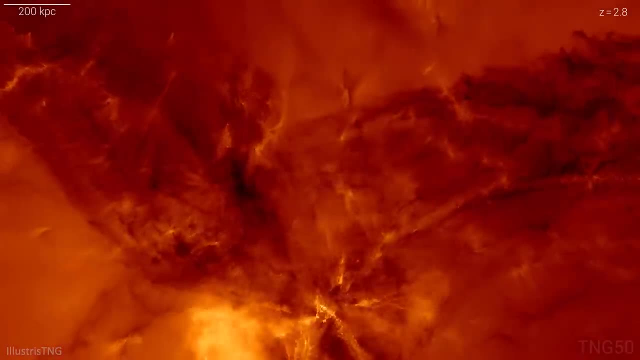 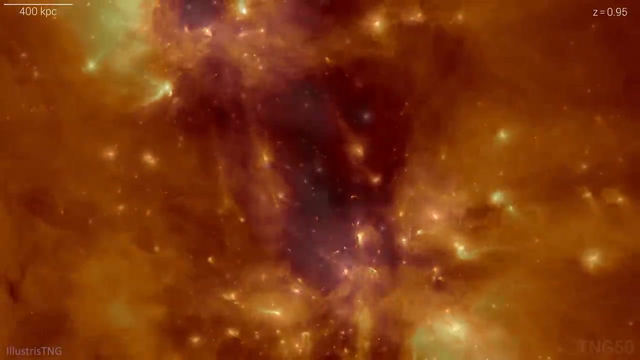 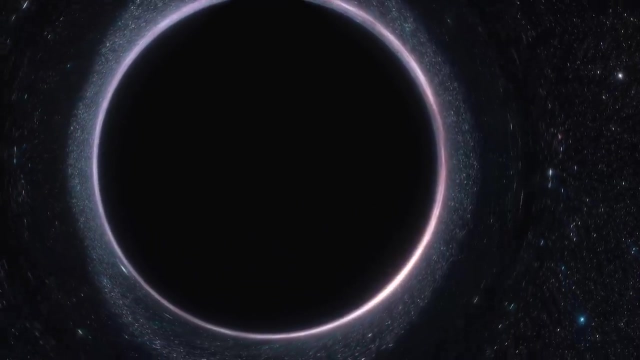 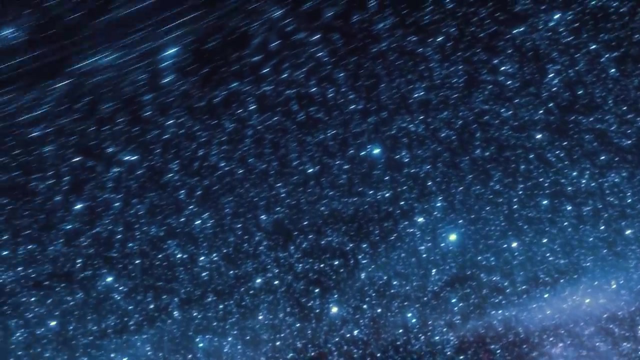 only a sixth of matter that came into existence at the birth of the universe escaped immediate imprisonment behind an eternal event horizon. How then, would you detect a primordial black hole? One toolkit depends on another of Stephen Hawking's predictions: Hawking Radiation. 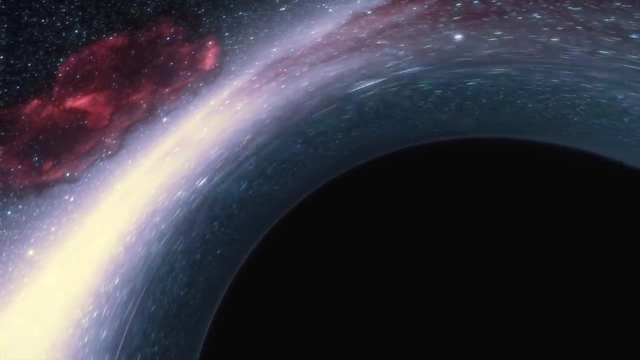 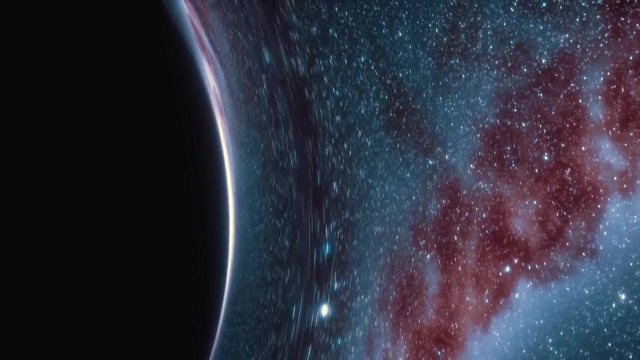 This is thought to be produced at the event horizon of all black holes, when quantum-particle interactions are subjected to general relativity. The result of this is that black holes emit a kind of gamma-ray glow and will shrink over time as they undergo something like evaporation. 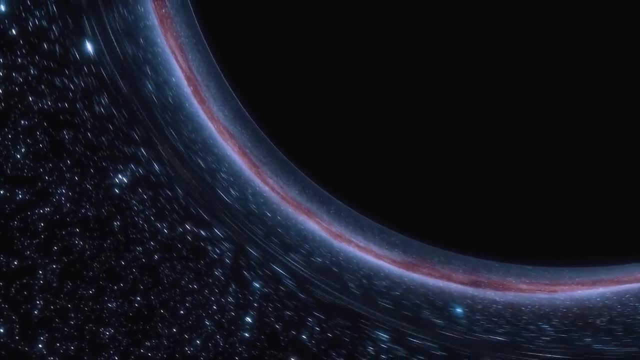 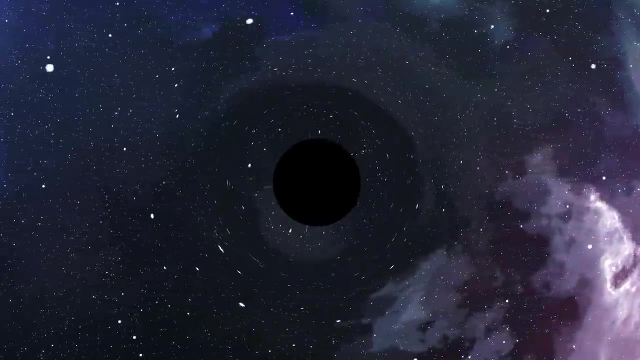 Not only that, but Hawking predicted that the smaller a black hole's event horizon, the faster it will evaporate, leading to an exponential emission that ultimately produced an explosion. Any black hole that was less than 10 to the power, 11 kilograms in mass, would be. 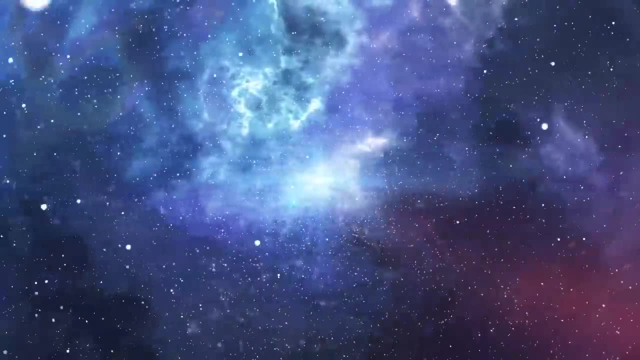 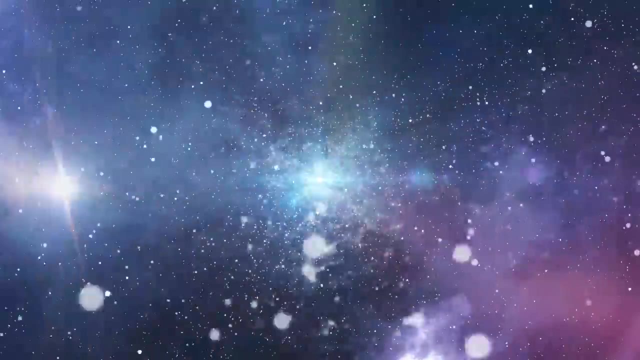 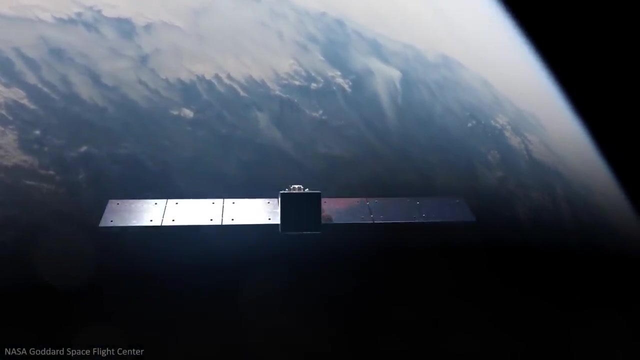 expected to decay on a time scale shorter than the age of the universe, so we could search for their swan songs across the night sky. The Fermi gamma-ray telescope, which has been circling our planet in low Earth orbit since 2008,, is well equipped to search for these gamma-ray explosions. 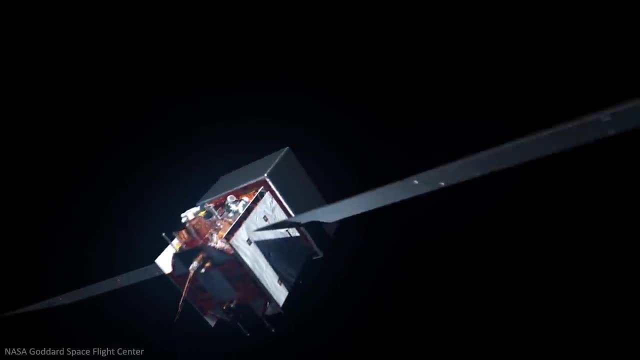 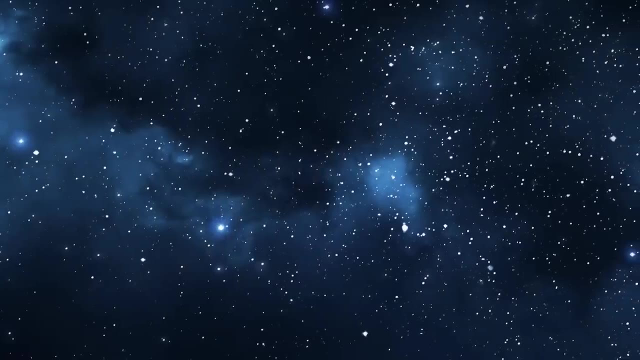 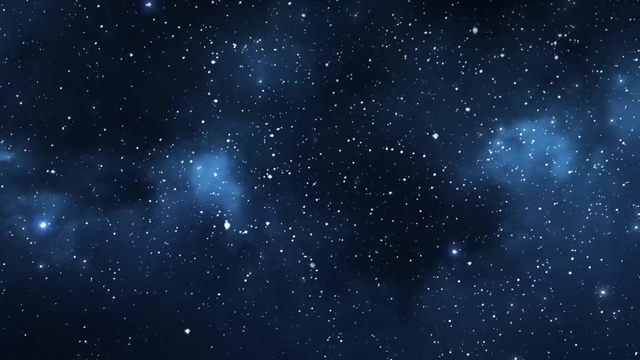 but the results of nearly 15 years of observation have not been promising, And here is a key piece of evidence, or lack thereof: The absence of Hawking Radiation outbursts suggests that, statistically, less than 1% of dark matter could be composed of these tiny primordial black holes. There is always the possibility that Stephen Hawking's theory was somehow incorrect and that Hawking Radiation and the associated explosions don't actually occur. Indeed, the conclusions are based on a mathematical house of cards with no robust data points to glue anything in place, But other possible detection methods are. 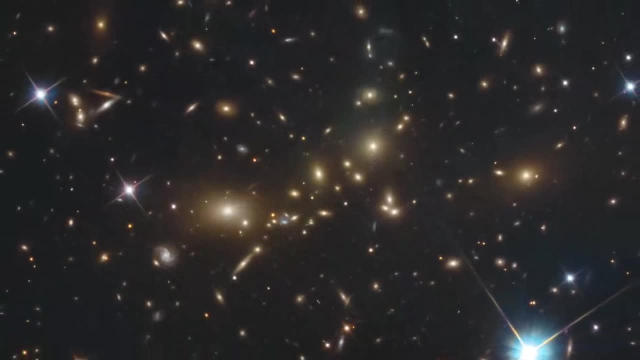 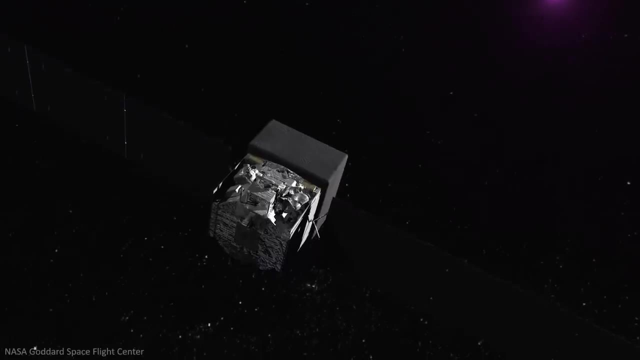 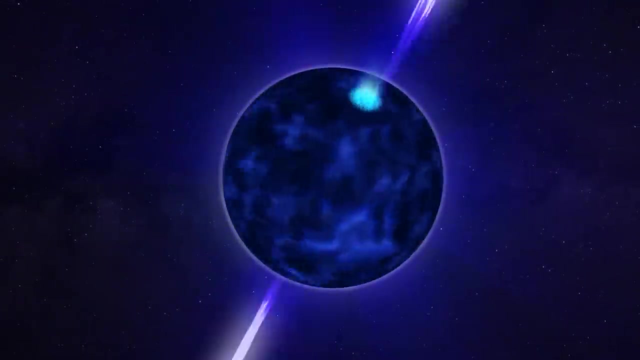 rooted in more traditional orbital mechanics and observed phenomena. The Fermi gamma-ray telescope has the ability to search for gamma rays from other sources, not just from potential primordial black holes, If those gamma rays from, say, pulsing neutron stars or supernovas flicker unexpectedly. 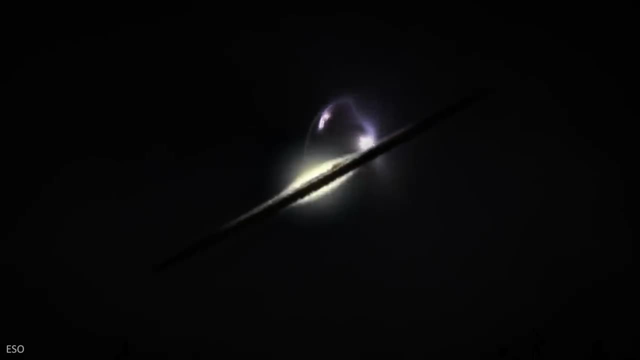 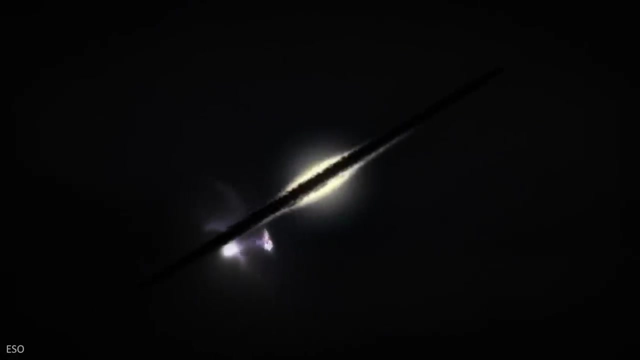 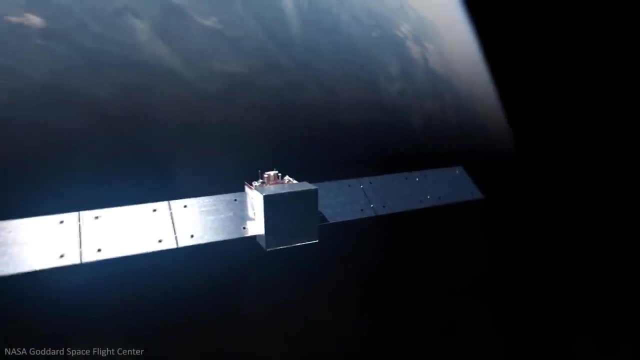 then this may be due to gravitational lensing as a primordial black hole passes by. Still, however, the results are not promising. Both gamma-ray and optical astronomy have failed to find convincing evidence of any black hole flybys, and the statistics based on the duration 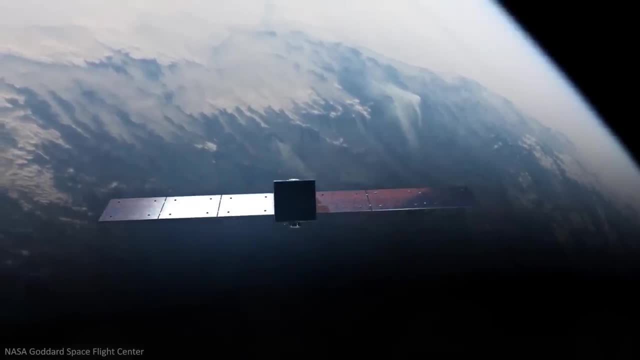 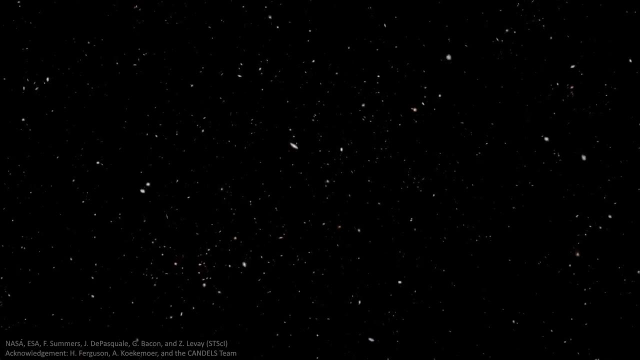 of the survey and number of candidate discoveries puts a limit on the numbers of primordial black holes out there that weigh a certain amount, And based on this, it's very unlikely that Earth-size or smaller black holes are the hidden machos that make up dark matter. 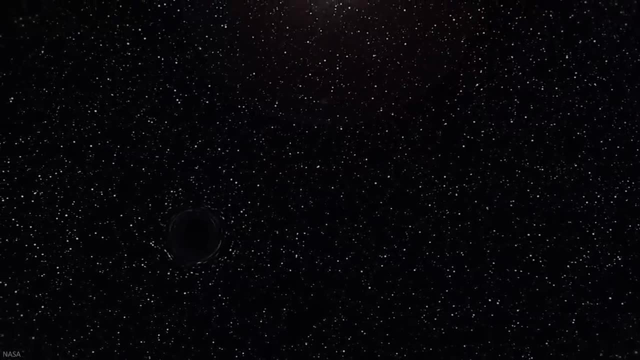 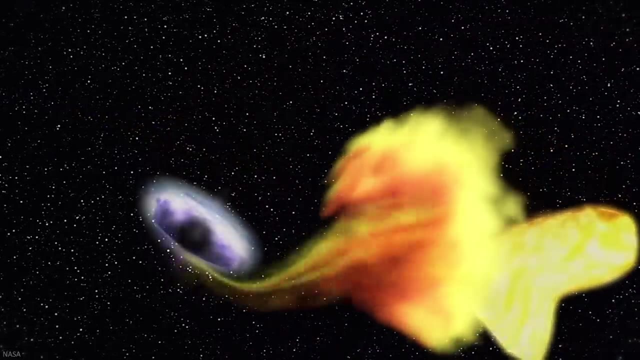 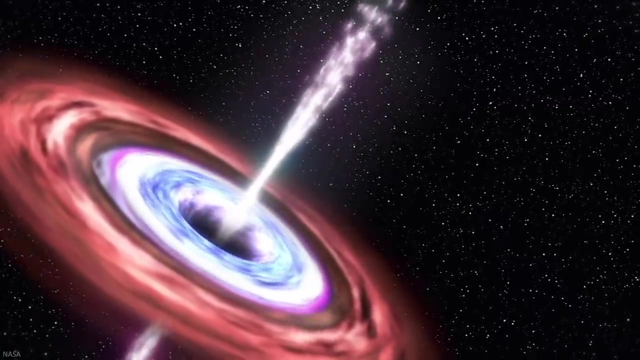 Some of these clues have been sought but are similarly lacking. It's expected that the gravitational wells of wandering primordial black holes would be able to capture other dense objects like neutron stars and white dwarfs, leading to their ultimate destruction. But the fact that these stars still exist in great numbers puts yet another limit on. 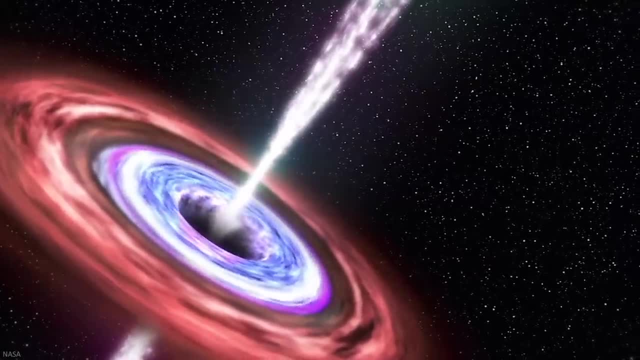 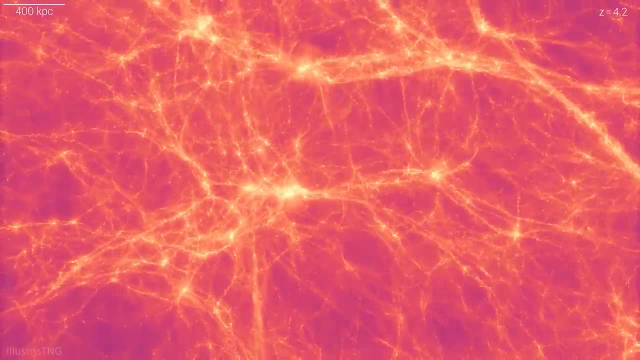 the possible number of primordial black holes that have been hanging around for the last 13.8 billion years. Even probing the cosmic past for traces of these early phenomena leaves us wanting. The existence of primordial black holes so soon after the Big Bang would have led to. 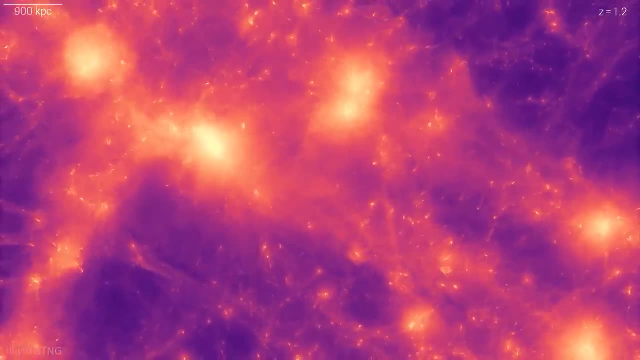 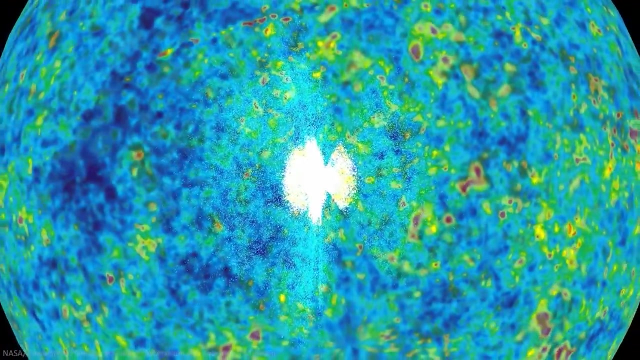 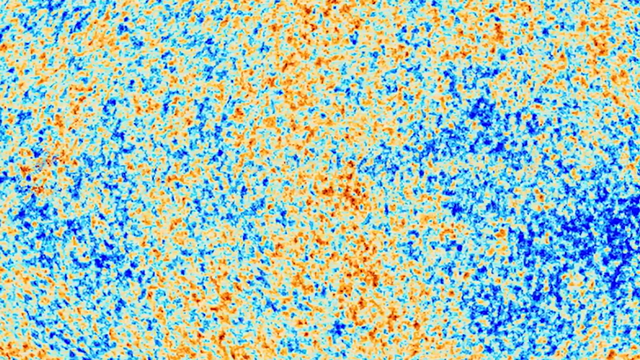 an accretion of matter early in its history, Early enough that it might be expected to create recognisable signals in the pattern of the cosmic microwave background radiation. But analyses of that universal-scale fingerprint reveal no signposts to early black holes, At least those between 100 and 10,000 times the mass of our sun, If they existed then. 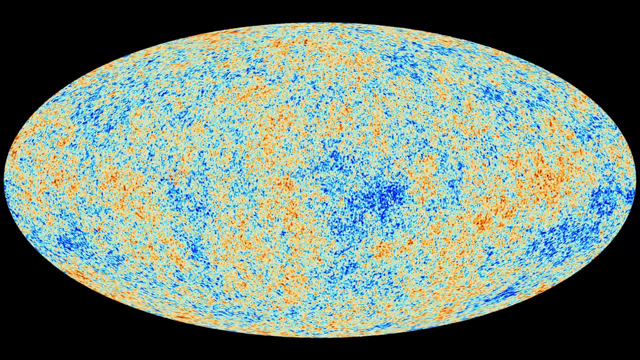 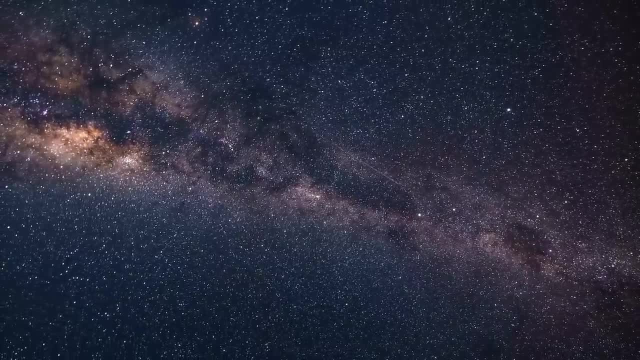 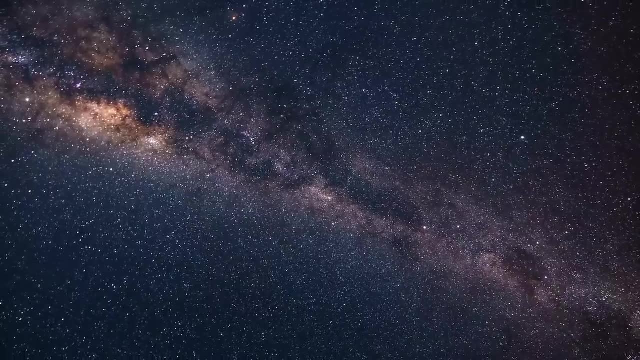 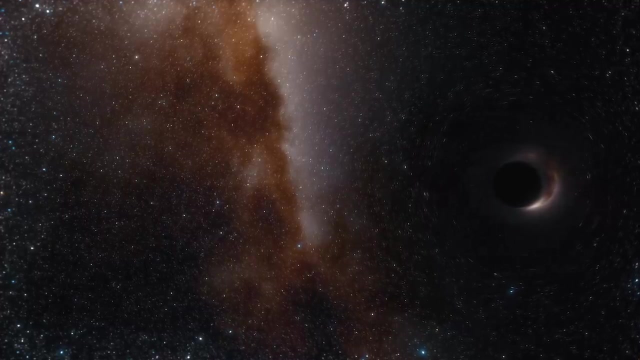 they were too small to leave a scar. Since Stephen Hawking first popularised the idea of primordial black holes in 1971, astronomers have tried to think outside the box to try and find ways to verify or refute his hypothesis. For the most part, they have yielded little in the way of positive results and for a 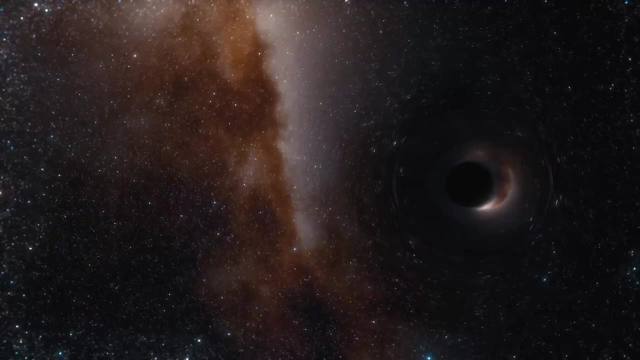 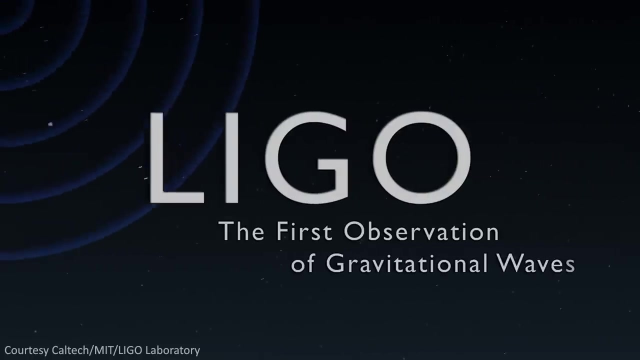 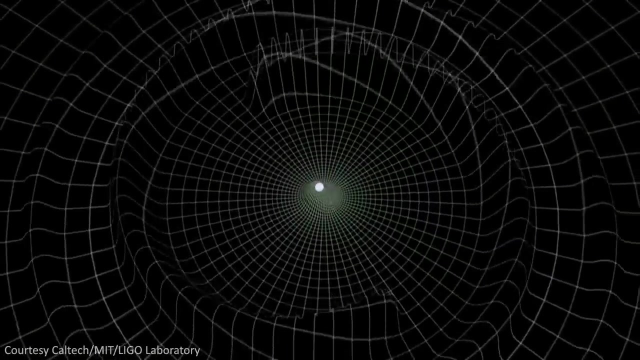 time the future of primordial black hole theory looked bleak. That was until 2015.. That was until 2015.. That was until 2015.. When the brand new LIGO instrument in the United States detected gravitational waves that were traced back to the collision of two black holes, each with a mass 30 times. 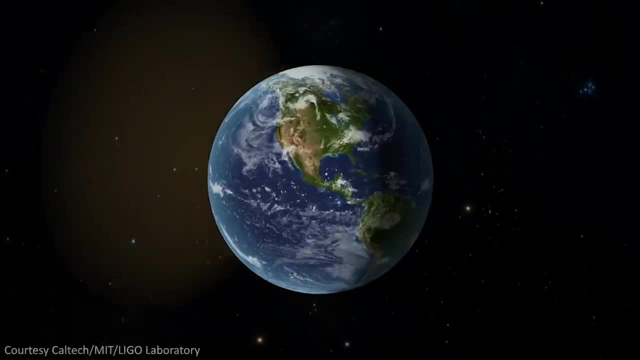 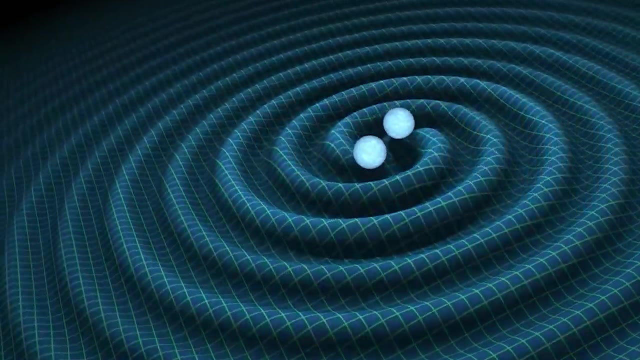 that of our sun. This detection alone was exciting and confirmation that gravitational waves were not only real and detectable but could also be a useful tool in probing the distant universe. But the implications of what they had found had black hole scientists excited for an entire 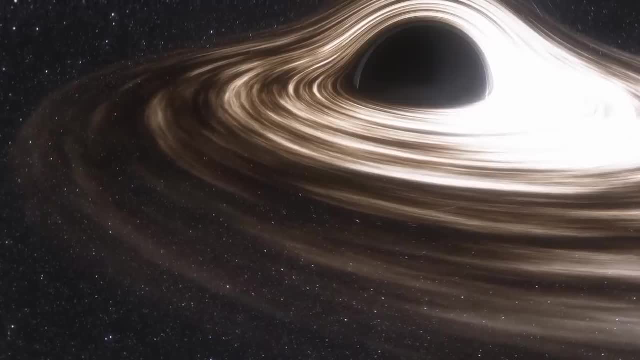 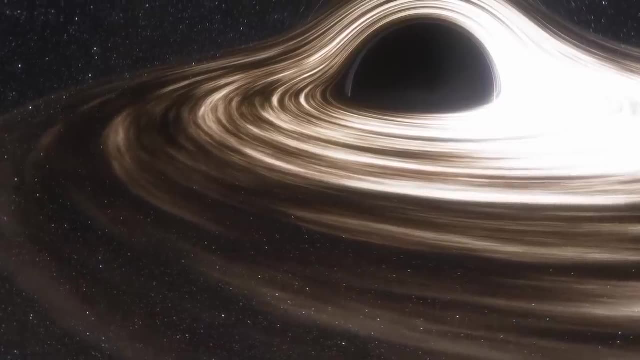 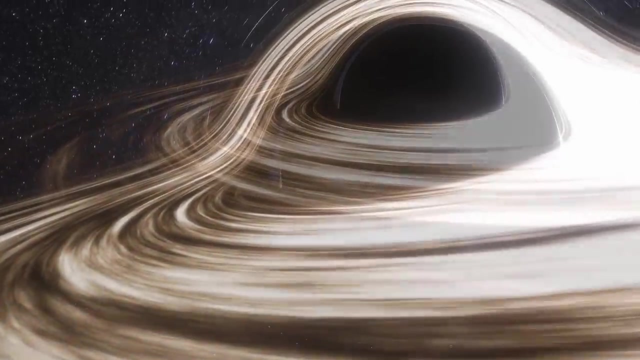 different reason. Black holes with 30 solar masses are too big to have been formed by conventional stellar death, And yet they are too small to be explained by supermassive black hole mechanisms either. Is there another possible explanation? Primordial black holes could very well be it. 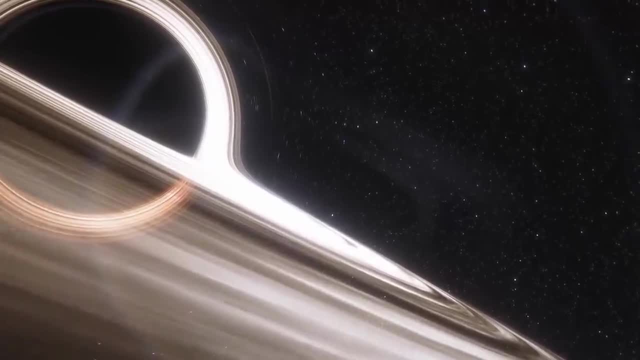 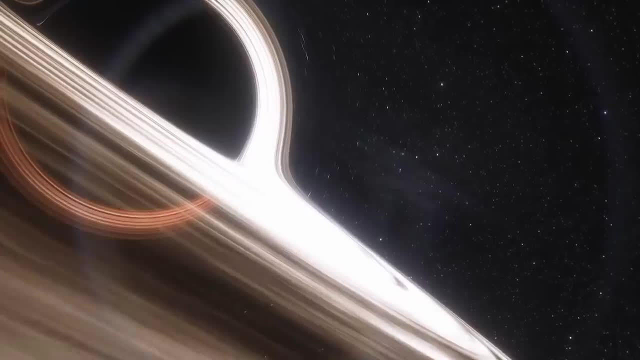 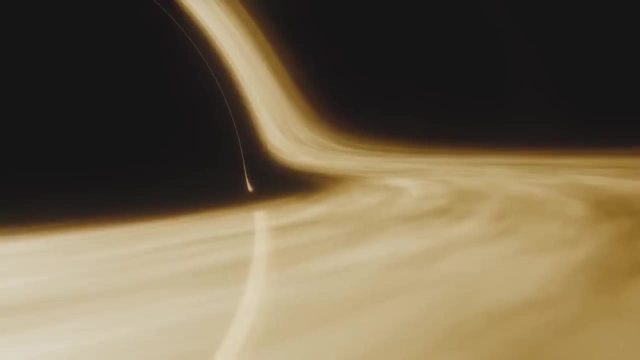 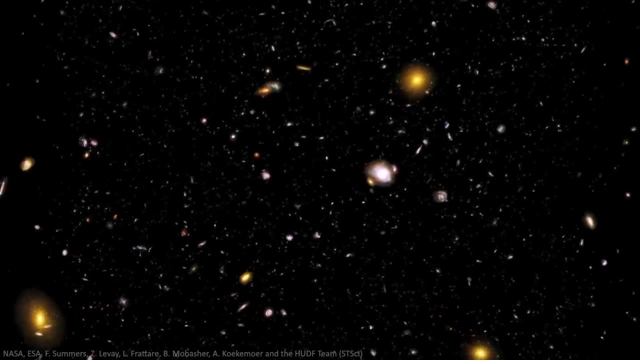 But what if they did? And so, finally, a measurable result seems to be breathing new life into old black holes. The earlier negative results hadn't altogether ruled out the possibility of primordial black holes, but rather put stricter limits on what masses they are likely to be. 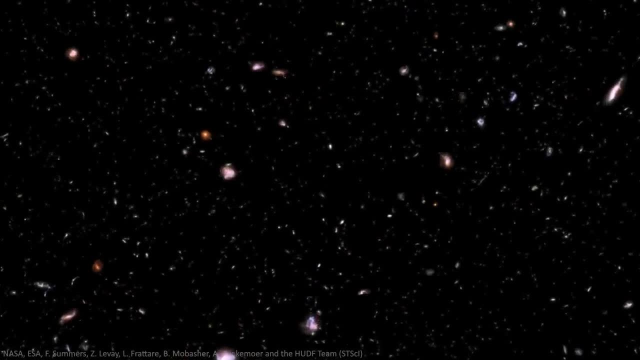 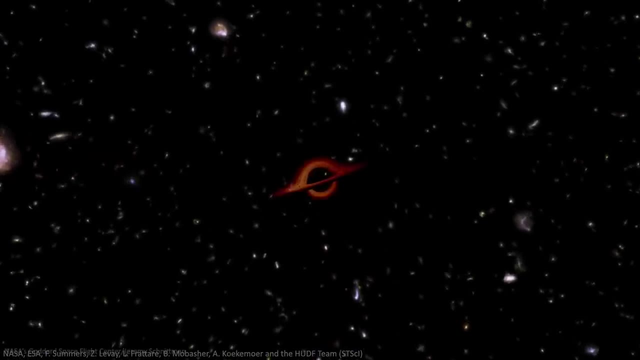 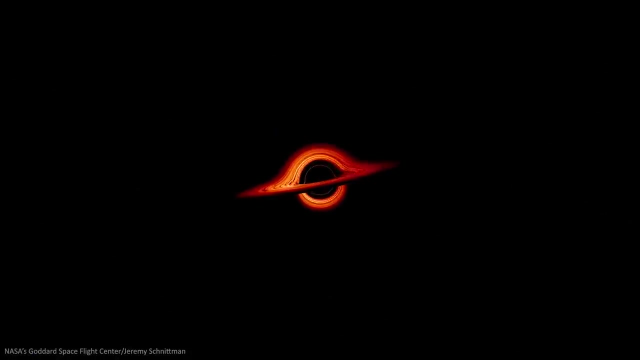 Such limits probably rule them out as the sole source of the universe's dark matter, But the case on their formation and influence is by no means closed…. and the mass ranges that still haven't been explored by current observational techniques do offer a tantalizing possibility: Indeed simulations that replace all of the assumed dark matter with primordial 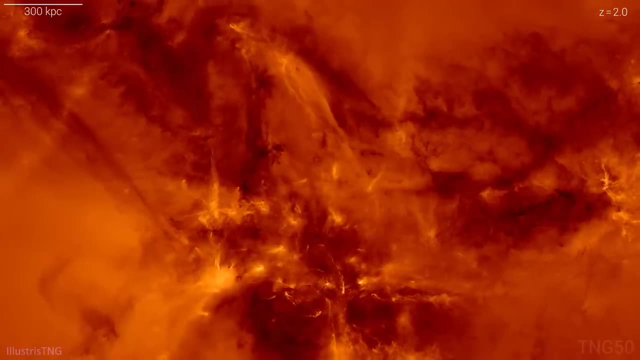 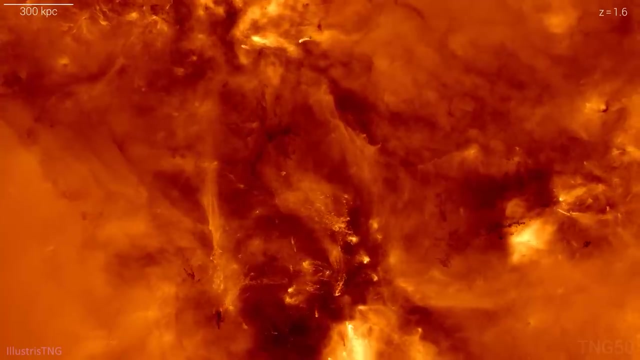 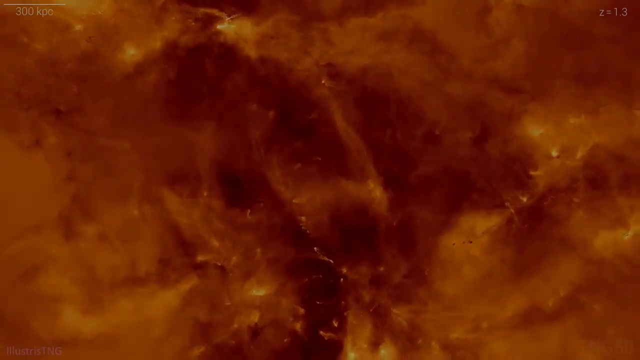 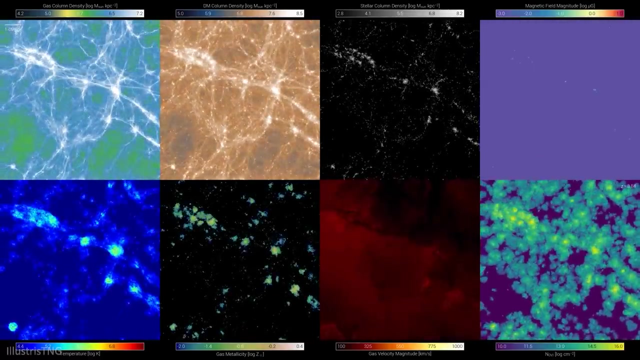 black holes of 1.4 solar masses show us that they could play a major role in the early evolution of the universe, including seeding the first stars, galaxies and supermassive black holes. The question of whether, when and how primordial black holes formed and evolved in the first second. 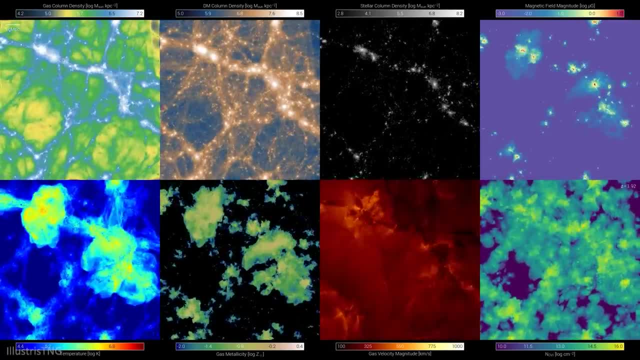 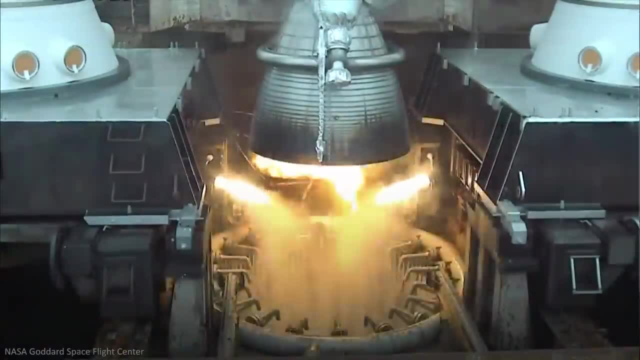 of the universe is still one of the biggest mysteries in cosmology today, and a topic that continues to attract speculation and experimentation. Scientists' hopes lie in the newest and most advanced instruments, such as the James Webb Telescope, which will image the earliest stars.